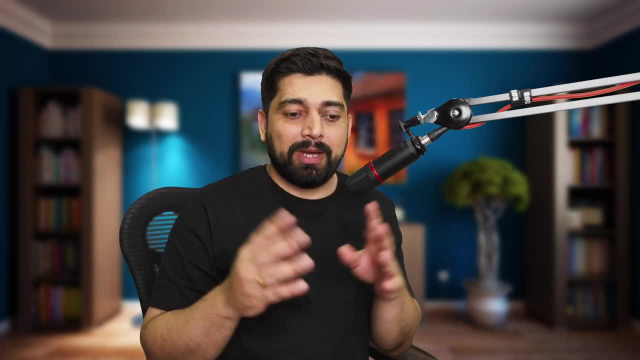 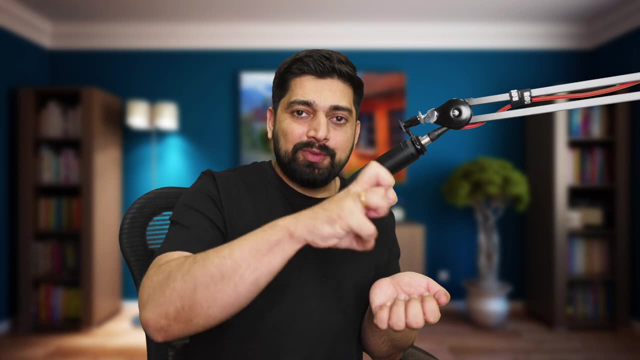 So the whole idea is to manipulate the DOM as much as possible. When you actually say I want to go into register page, React never goes anywhere. It's a single page application. It removes some of the elements from your homepage and injects some of the React register page on there. 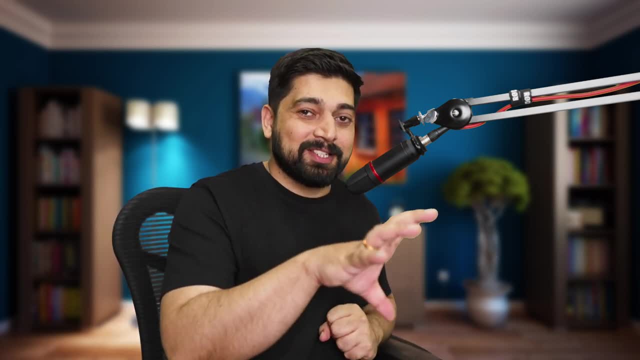 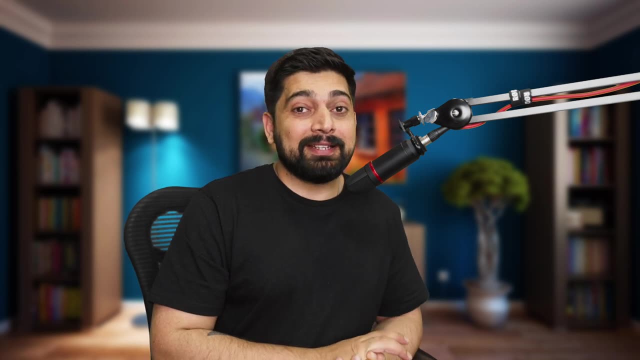 It removes the register page and injects the login component and once you are successfully logged in, then it removes that and gives you a dashboard just right there and your page never, ever refresh. But this is not ideal For a regular user. A regular user doesn't really understand. 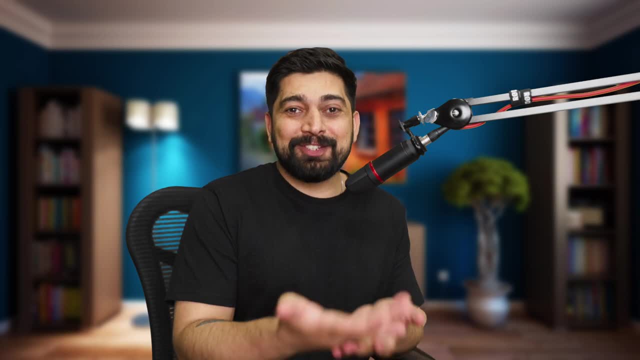 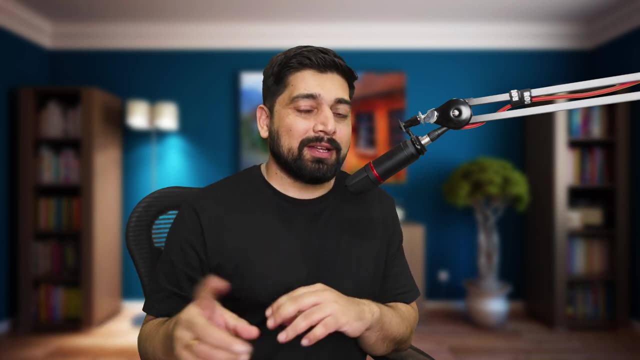 and we cannot train the entire world population how to reuse the internet just because we have designed a new framework or a library. So the concept of moving users onto different URL, like register page login, is so common that if you don't do this, people might think that it's very suspicious. 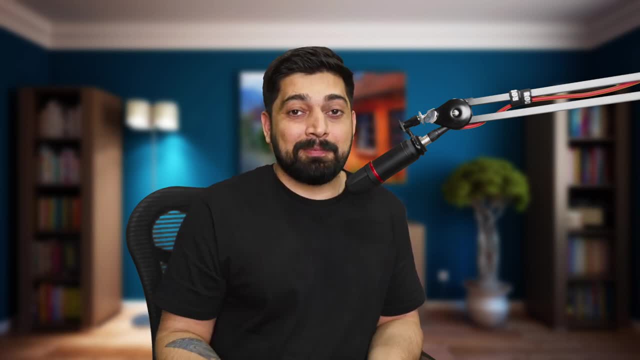 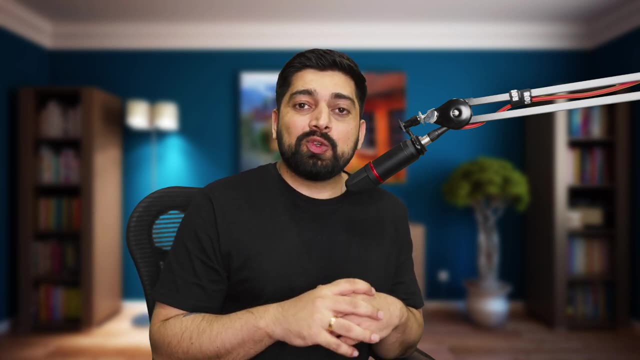 and it's not really a great thing for the URLs and the safety precautions, And that is why we need to figure out a way that how we can artificially inject the routing so that the URL looks great and user feels like they are moving onto different page. 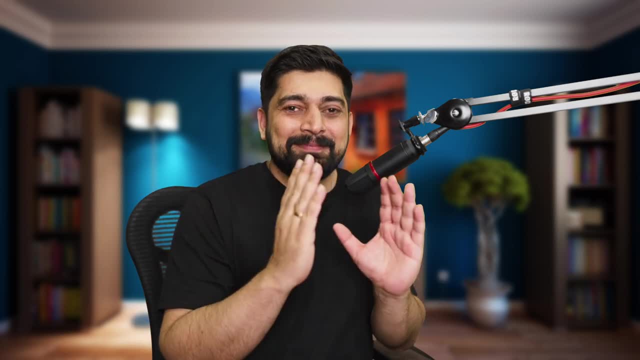 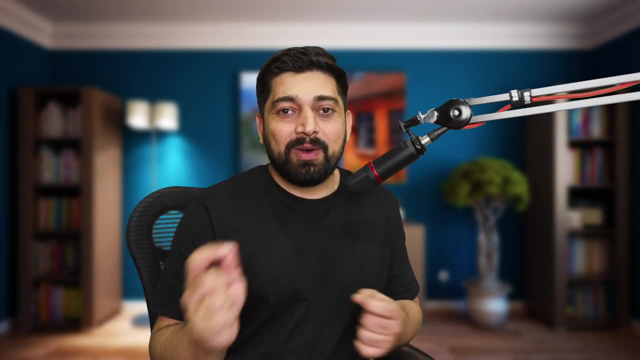 although it's just React at the behind the scene. It's just a single page application And, yes, everything happens artificially. That is just a simulation being done that you are onto different URLs. Your page will never refresh. still the React concepts bringing in the components. 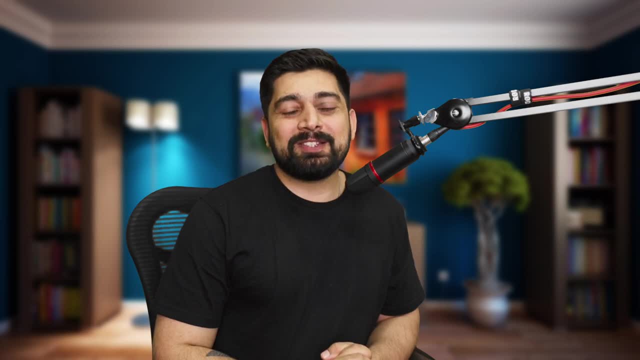 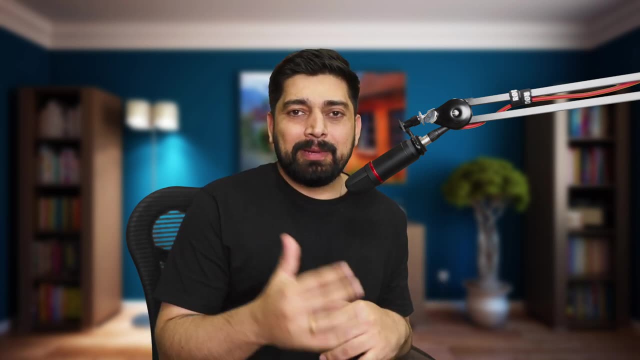 injecting the components and all of that. So we'll be learning one such way of doing that. By the way, this is a core React course. That is why we are discussing about the routings. By the way, on my channel you will find there is a Nextjs playlist. 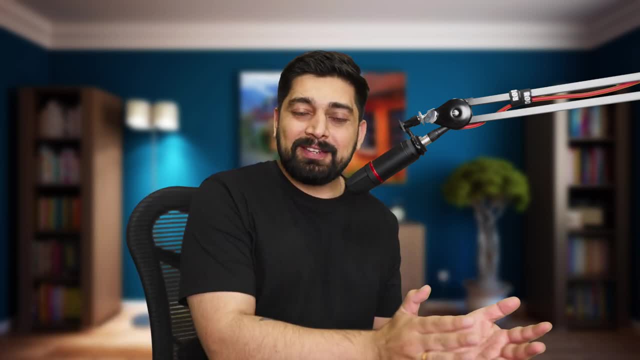 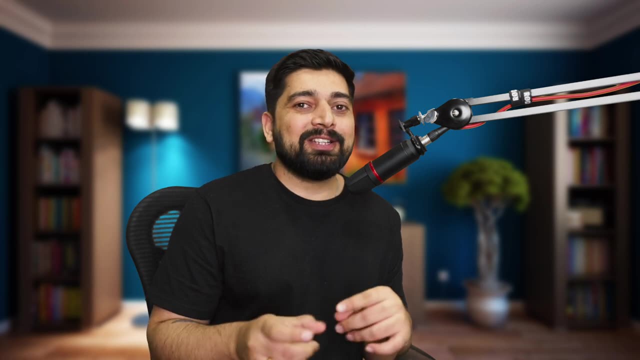 separately available. So in that we don't discuss too much of routing, that routing is different And, by the way, in case you are just interested, I do have a separate video on my channel in which I have showed you that how the Nextjs routing can be designed customizably. 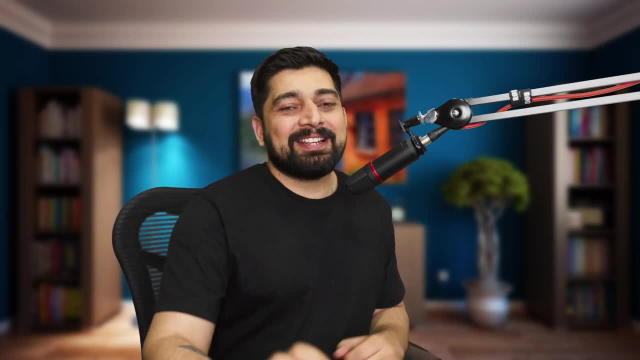 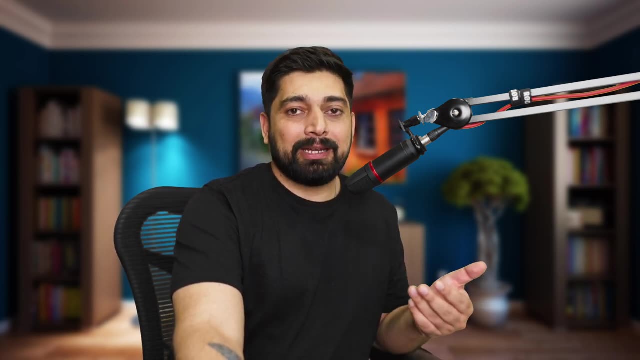 Yep, pure JavaScript, how the React router works. Anyways, let's move back. So in this video, first let me show you what we are going to build, and then I'll give you some of the concept of how to study the documentation. 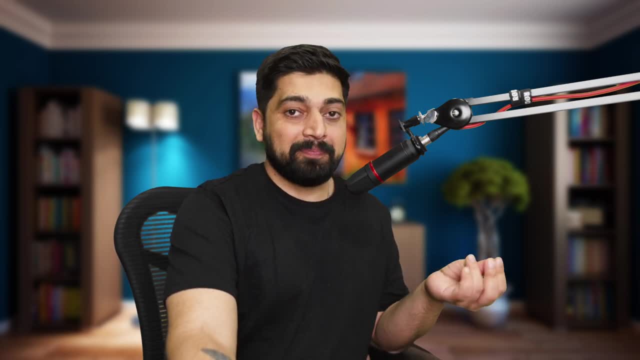 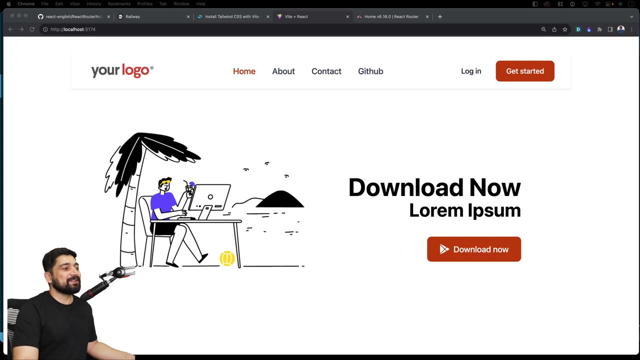 and figure out things on your own With the React router DOM. That is the library which we'll be studying, So let me first take you onto the screen. There we go. Sorry, we don't have any dark mode for this one. 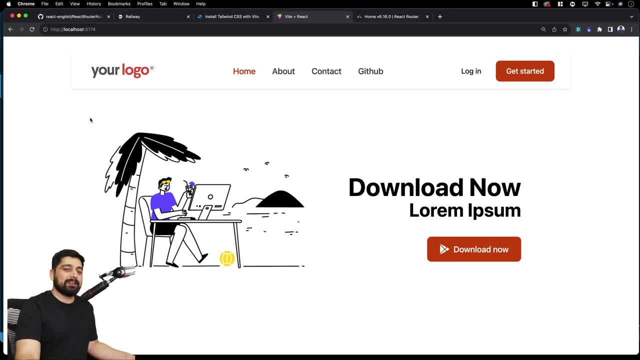 But this is the application that we'll be building. Luckily, you don't have to worry about CSS. I'll be giving you some of the files. I'll show you that as well. So this is our homepage, and I recommend you to notice the URL. 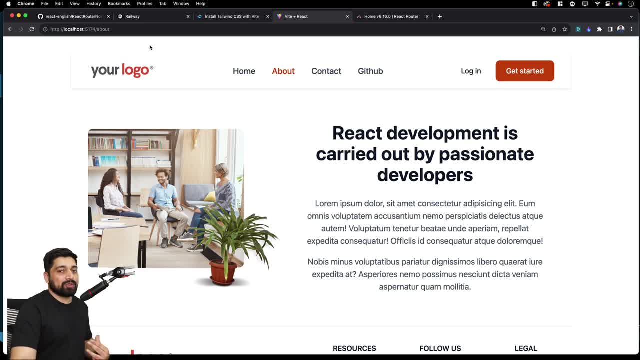 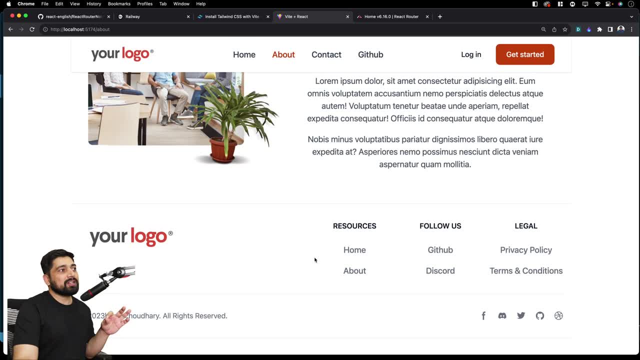 This is the homepage. When I go onto about page this is slash about. So this is simulating that you are moving onto the next page. but end of the day this is just React. Navigation bar never changes. Our footer also never changes. 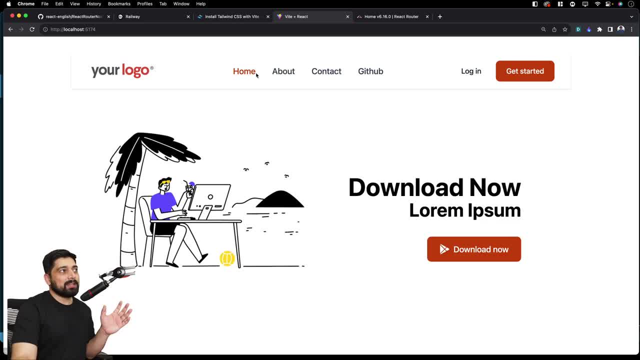 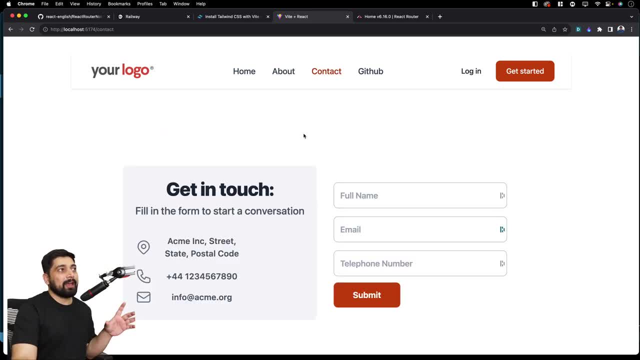 They stay exactly the same. So, if I go back to the home, navigation, bar remains exactly the same, but our URL changes a little bit. So we have a homepage, about page and a contact page that we have And similarly we will be having a GitHub page. 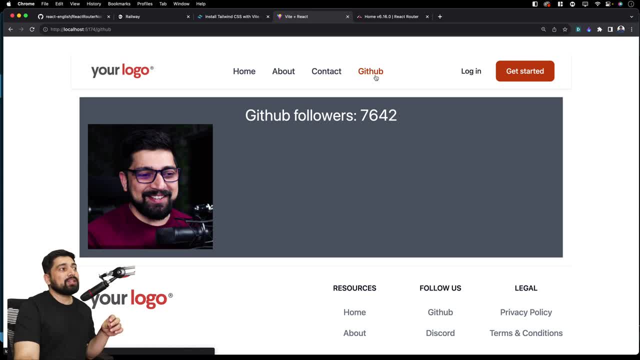 but the GitHub page, additionally, will do something different. The GitHub page will show my photo as well as my GitHub account, and we'll see that how we can optimize it through the React router DOM, which is the library we are using. So every single time we have these application going on, 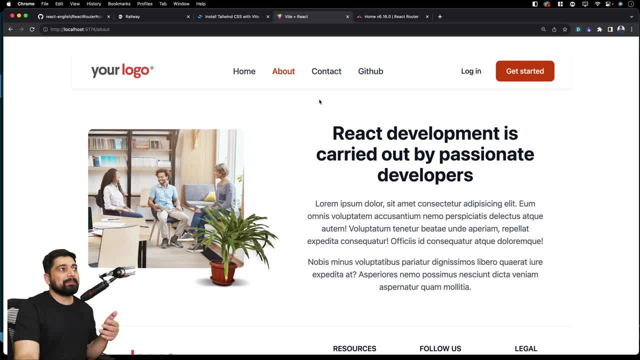 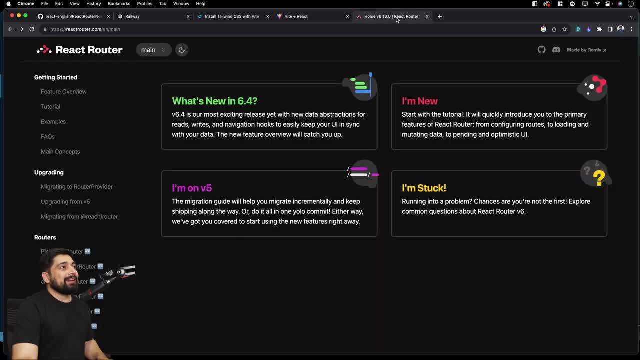 like this, GitHub and about. we'll also see how we can grab some of the URLs and whatnot. There's a lot more that we'll be studying than just being shown on the website itself. All right, And the package that we'll be studying is React router DOM. 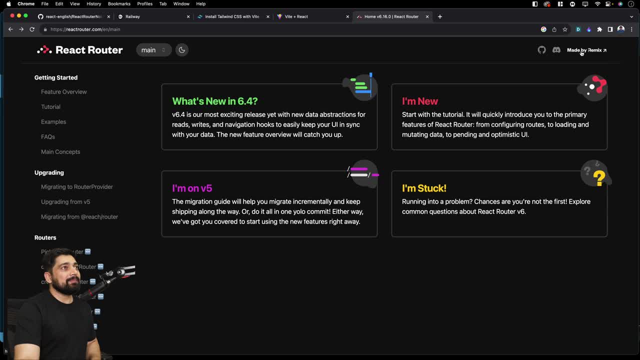 It's available on reactroutercom. It's by the Remix team, made by Remix, And what we'll be doing is there are a lot of ways how router actually evolves, and especially the version six which we are at the time of the recording video. 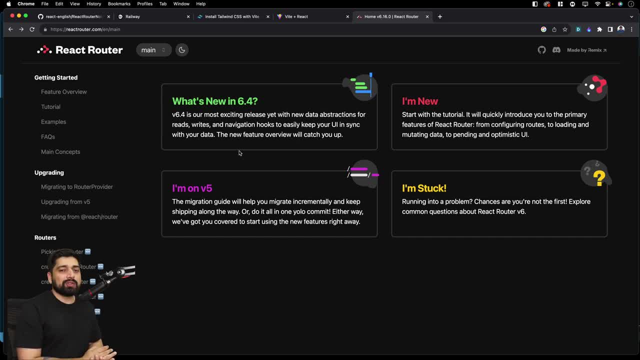 This is the newest one. We'll be using that one only, But I'll walk you through how you can actually explore the documentation. Otherwise, my channel is always available for you to help, But we'll be seeing that how we can use the six version. 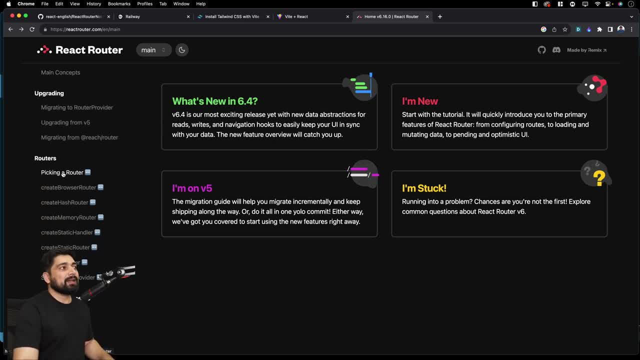 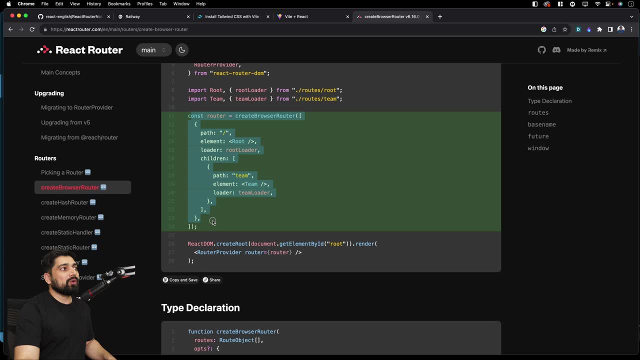 We won't be talking about the five at all. We'll be seeing that, how we can pick up different variations of the router. We'll be using the create browser router And the whole idea is to study this piece of code so that we can load things on our own. 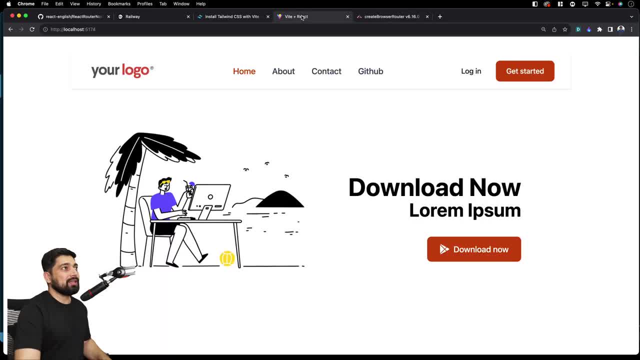 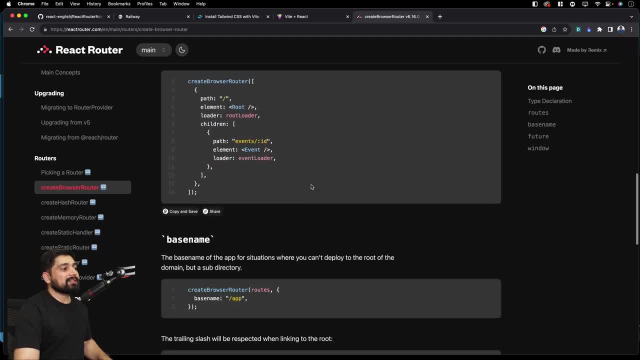 and can design the routing for this application, the sample application, which will give us the entire idea of how the application is built and all of that. We'll see some of the optimization tasks and techniques and whatnot. So everything will be pretty nice up there. 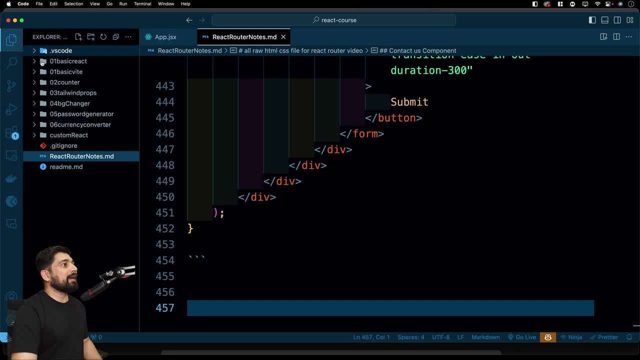 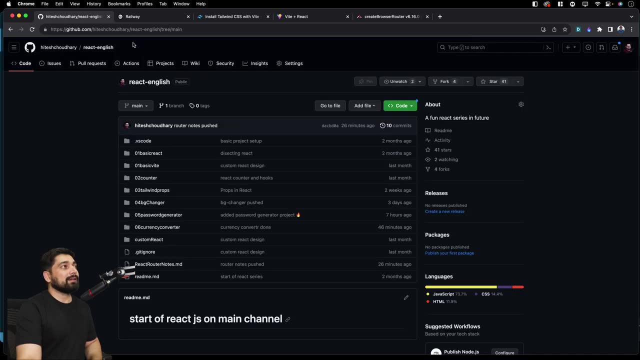 All right, enough of the talk, Let's go back onto this one. And, by the way, one more thing, If you'll go onto this one. so I have a repo on my GitHub account: githubcom- slash iteshaudhari. 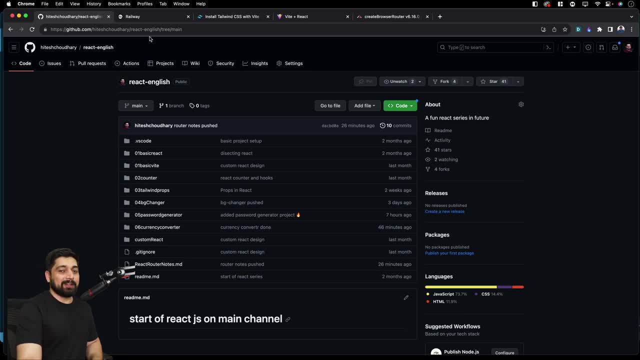 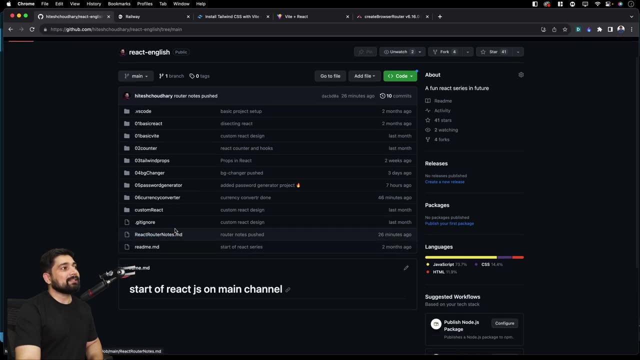 You can find a repo with the name of React English, because these videos are in English, And you can see that there is reactrouternotesmd, which is the code that I'm using right now, And you can see that this repo is available for you. 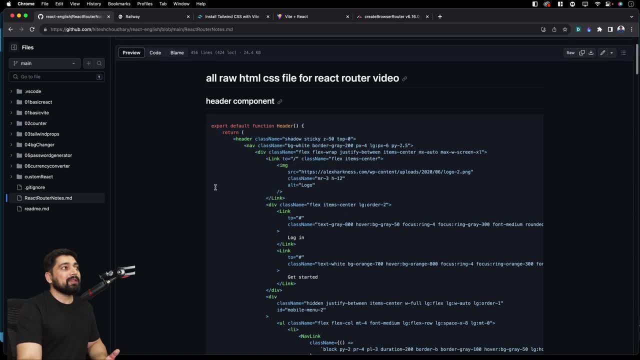 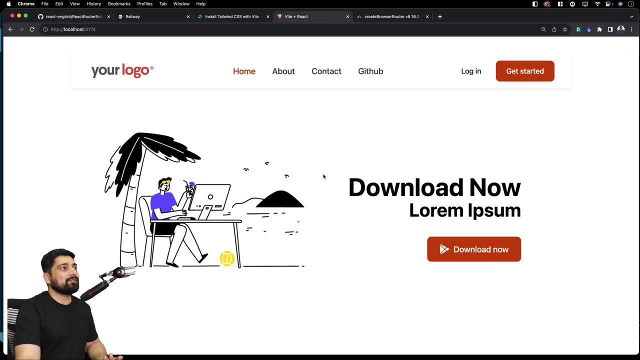 This is a markdown file which will help you to actually grab the components, Like, for example, for the header part or the navigation bar. this is all the code, which has nothing to do with the React routing. majorly, It's just a CSS. 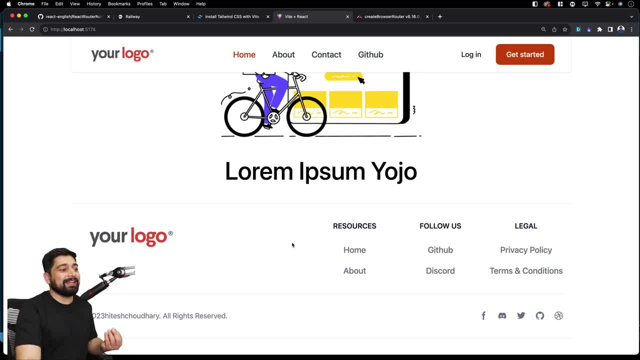 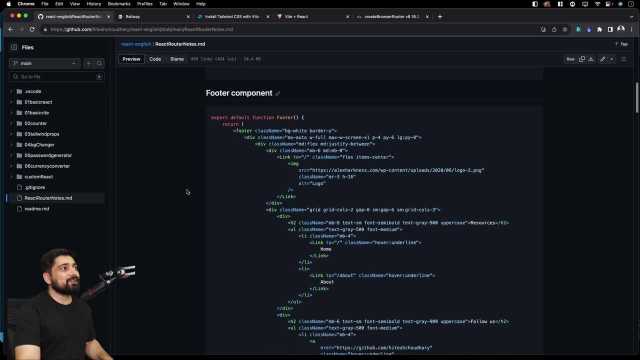 Similarly in the footer. if you check out the footer, this is just a static footer. We just need it to understand a few concepts. It could be just one liner, but nobody gets impressed with the one liner text. That's why we are actually giving it to you. 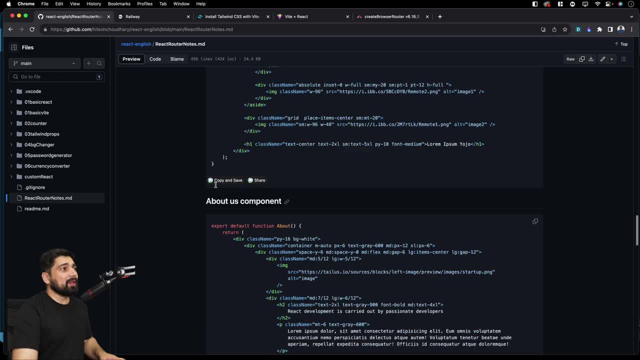 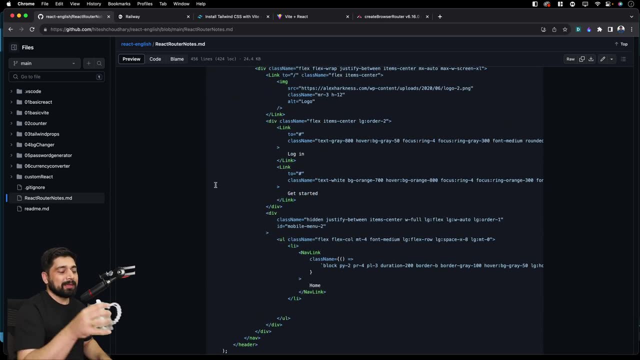 So you can find the footer component. Similarly, we can have home component and contact us page. That's it. GitHub will be designing on our own, So that's the basic part of it. So let's go ahead and create a fresh new project. 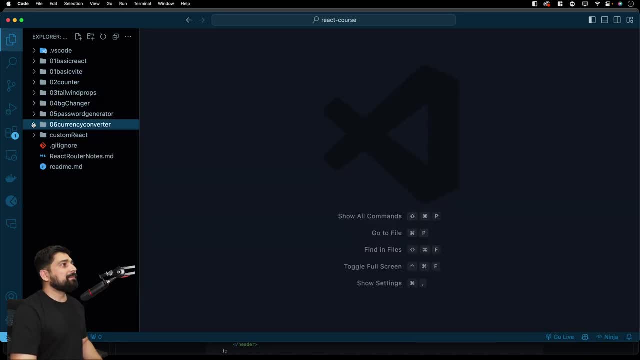 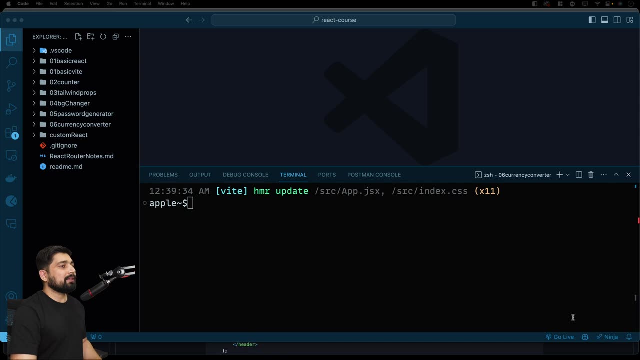 and work with it. Okay, let's grab And there we go, Okay. so first of all, let's kill this. We don't need you And let's go ahead and work on with this. Just give me a second. 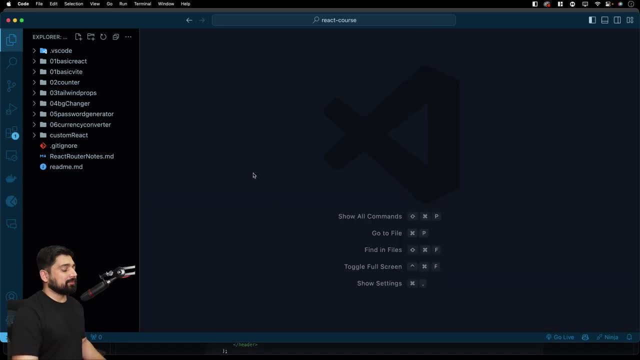 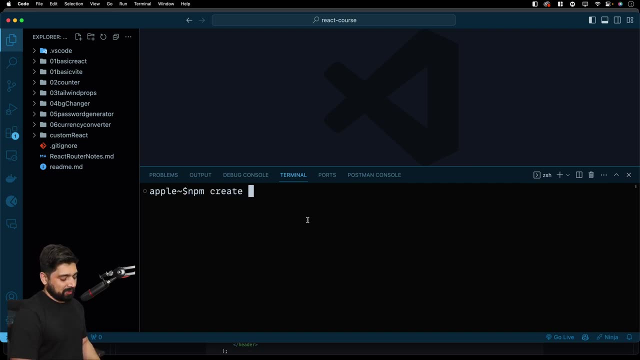 I'll align the things and remove this one. Let's start a fresh one And we'll say NPM, create Vite, not React. And this one is going to be an introduction to just the routing, So we'll be calling this one, I guess. 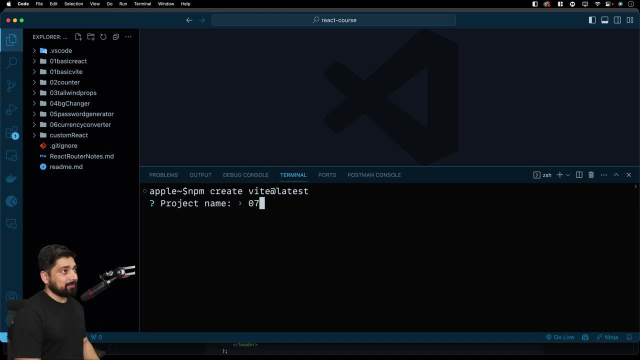 the seventh application that we have, So zero seven, And we'll be saying React- router Package name is same. We'll go with React and JavaScript, All right. so this seems good. Now we need to go inside the folder, But, as you know, I prefer to actually right click. 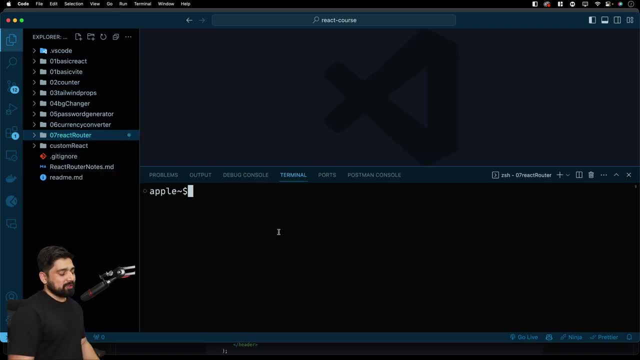 and open the integrated terminal. That way I'm always into the route, So I can just run NPM I to install the application And we can actually go ahead and move on to the browser itself. So let me go ahead and get into the browser. 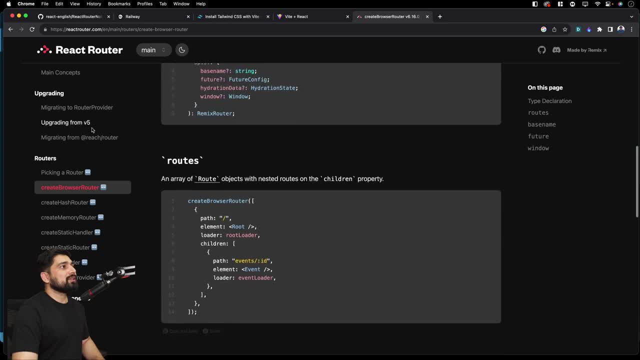 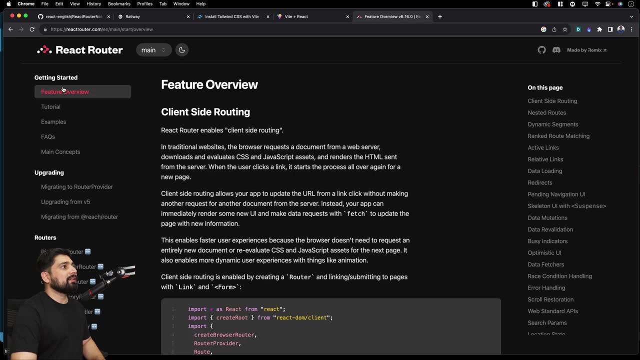 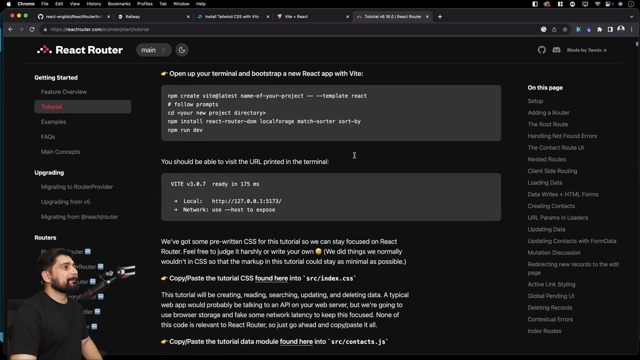 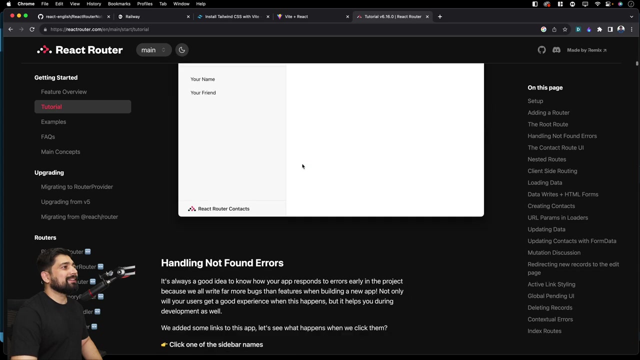 And how we can actually install this. So there are main concept, migrating, all of this. Let's go on to getting started, And there should be getting started guide tutorials. Oh yep, the project install. Just get me the NPM install command or I'll do it myself. 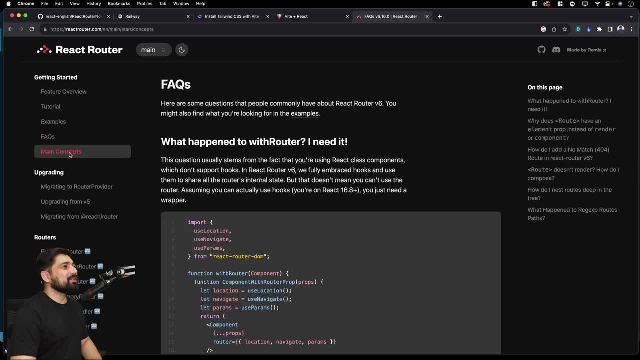 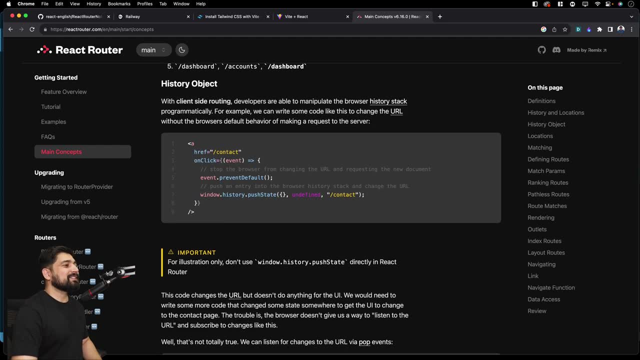 Okay, no examples. FAQ: main concept. Okay, I understand the main concept. Just give me that path. Okay, probably it's not going to be nothing. it's a React router DOM, So I'll just install it. So NPM install it's React. 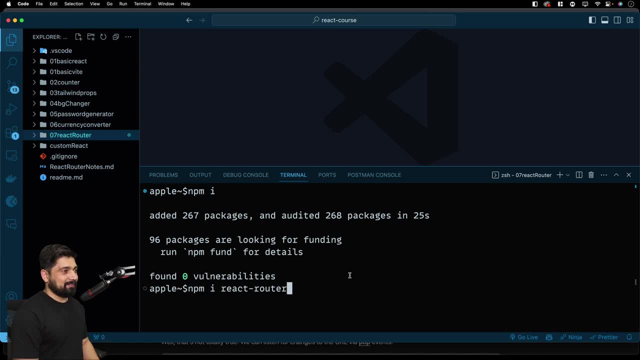 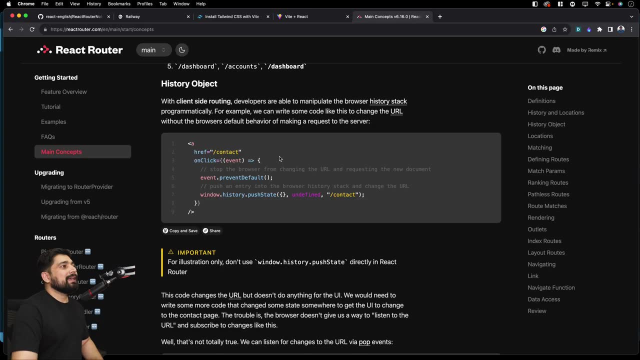 Somewhere it is, I'm not able to find it. React router DOM, a very famous package. If you are anytime working on the React, this is the package you will be dealing up with that. Now, in this package entirely, all you have to do is go with the main concept. 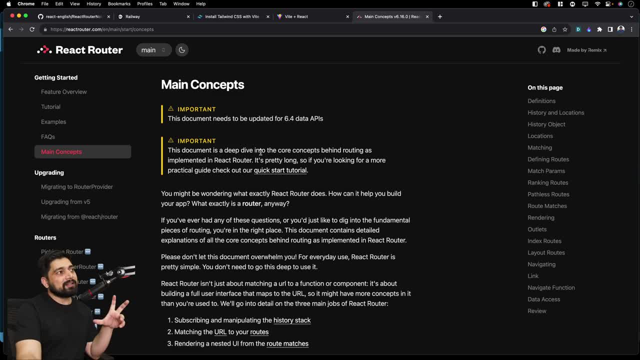 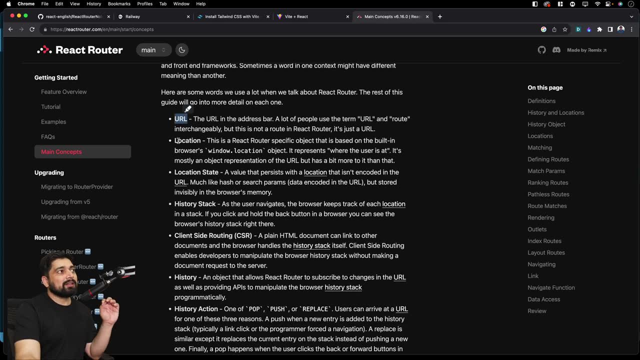 This is really the essence of how to understand the React- React router DOM: what happens, how it happens, And a lot of essential things are mentioned in this one. So how you track the URL, how you track the location forceful, although we'll be studying a lot of it. 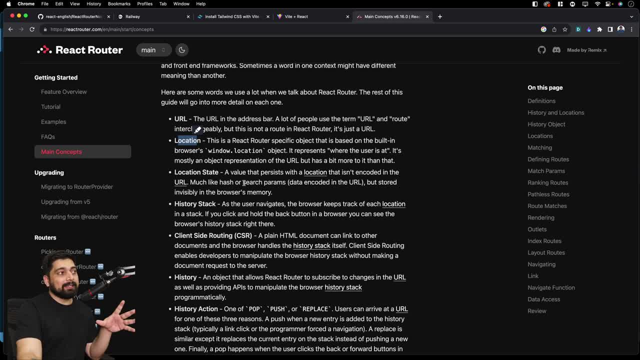 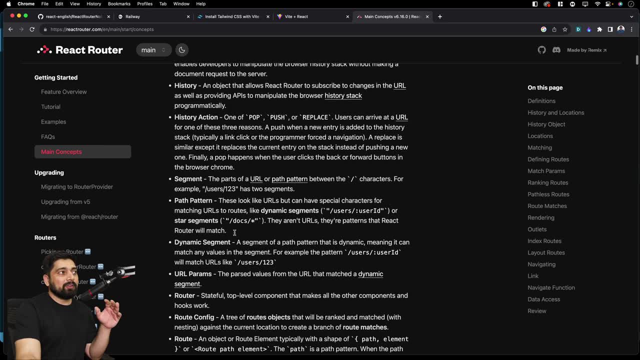 especially the router inside, when we'll be building a mega project finally in this series. So all these things like client-side routing, the location state and all of that will be taken care there. But if you have time, go ahead and go with the main concept. 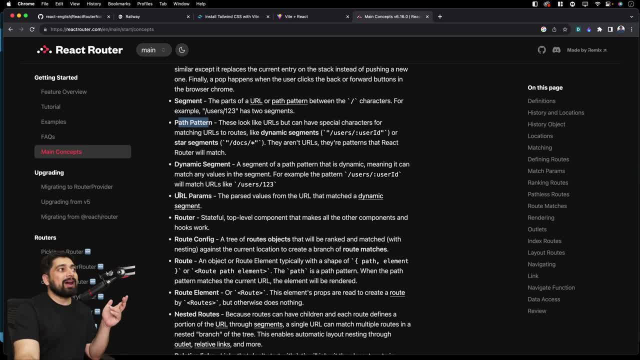 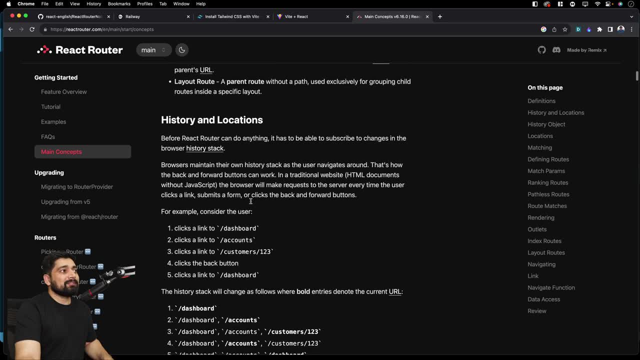 Some of them we'll be studying here, like the path patterns, what this is, how to grab the URL, params, dynamic routes, dynamic routing- we'll be studying in this one, But definitely this is a very rich guide, These kinds of concepts. 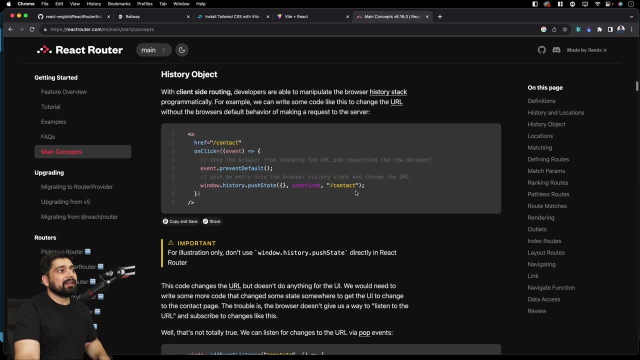 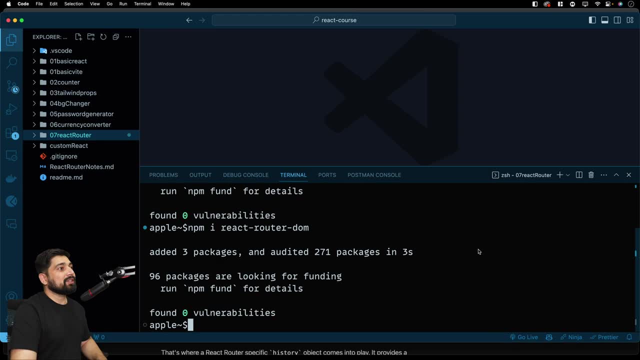 these all will be taking care of this, But it is always a good idea to actually go with the main concept documentation. This is the part where you study and you read out the stuff. Okay, moving back. So now everything is installed, Let's first go ahead. 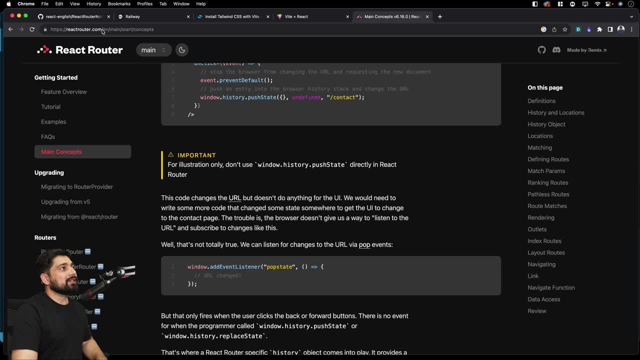 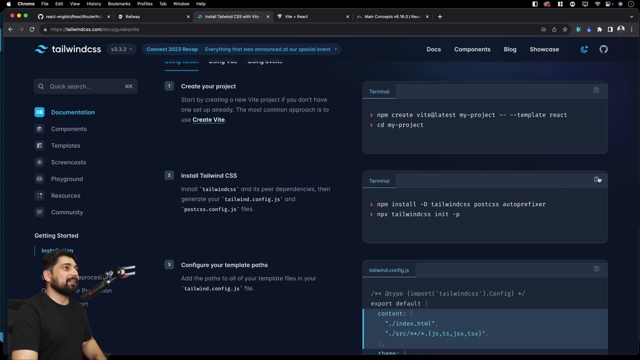 We'll be needing Tailwind as well, because if you look out the classes and all of that, yes, there's a lot of Tailwind, So let's go ahead and install the Tailwind as well. One more time, In fact, a lot more time will be coming up. 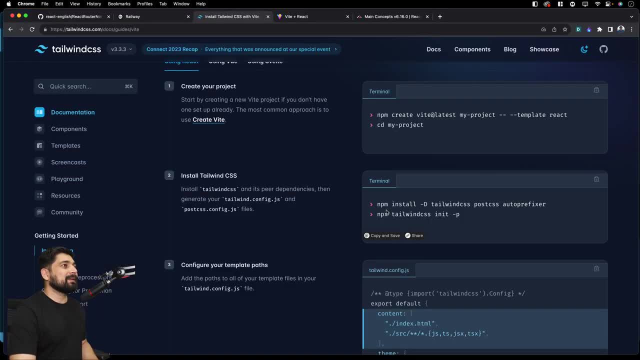 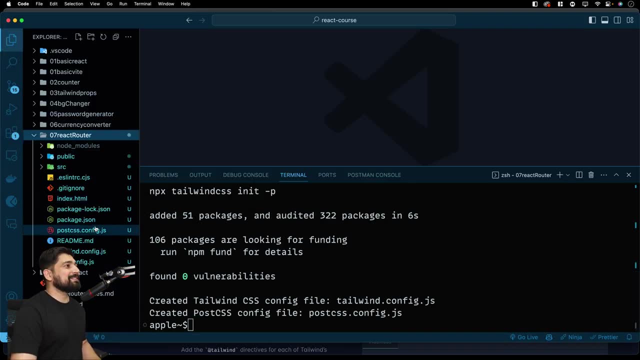 in the future as well. Okay, so this is what we have as a Tailwind, And we need to actually copy the content. I'm pretty sure you might be just kind of memorizing this at this point of time. Okay, the content will be replaced. 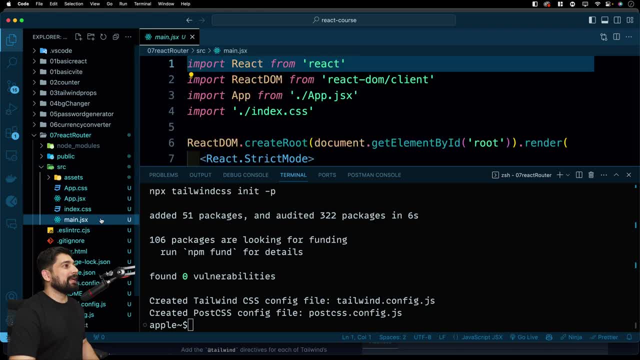 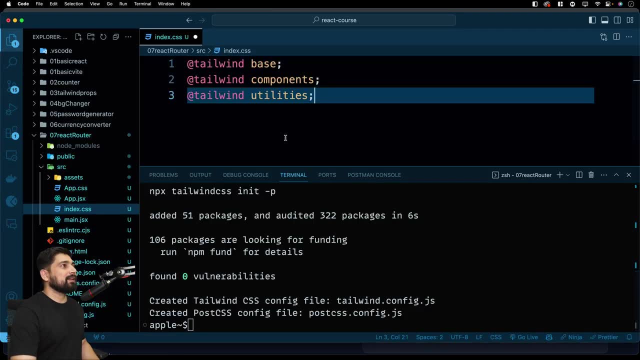 Save that and go into mainjsx- no indexcss. remove everything and we'll be grabbing these ones. Copy them and paste them up here. Save that. We don't need anything into the appcss as well, Just remove everything. 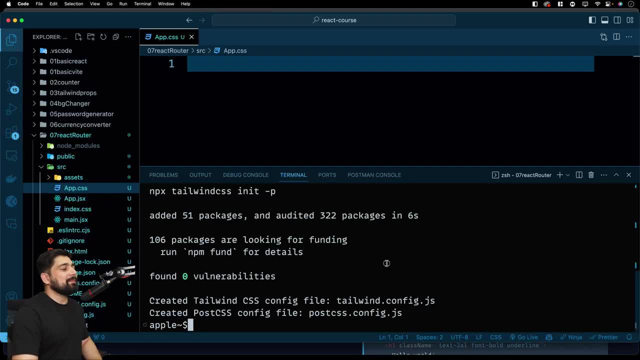 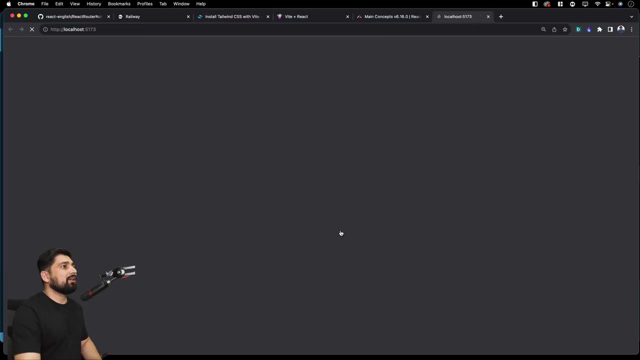 We won't be needing, we won't be using actually the app itself. Okay, Further, let's go ahead and run: npm install npm run dev. npm run dev. And that should be up and running on my system. There we go, basic. 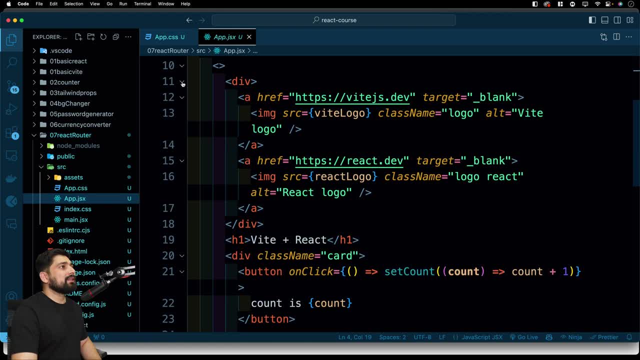 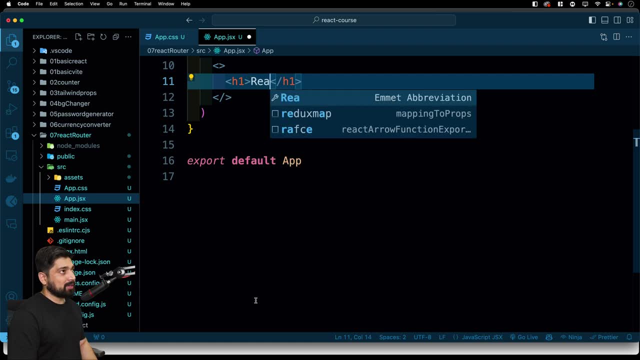 Since the appjsx is anyways getting loaded, let's go ahead and at least grab some of the values out of it. So we'll be saying h1, react-router, react-router-dom, And we'll be saying: let's add a class name. 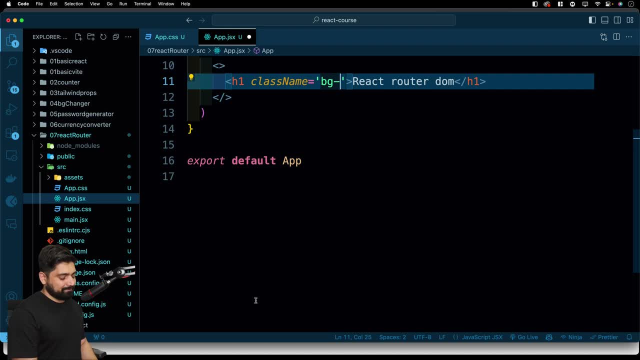 And we'll be saying bg-what? hmm, green Suggestions, yes, bg-green-300.. Let's see, yeah, at least our Tailwind is working. All right, we won't be touching this thing here. We'll be getting started with a couple of things. 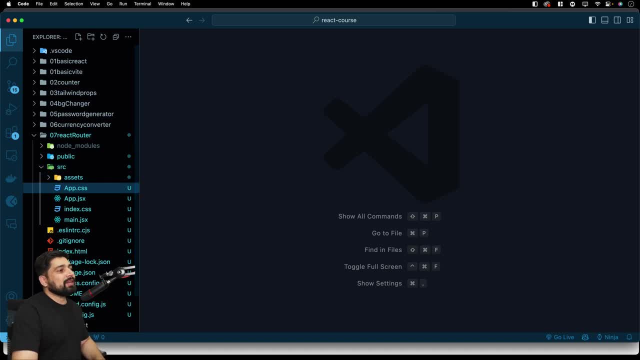 We'll be starting with a couple of routes and folders and basically trying to get a feel of how the entire thing actually works. So first thing that we are going to do is there is always components, or some people call it as pages. Totally depends on you how you want to call it. 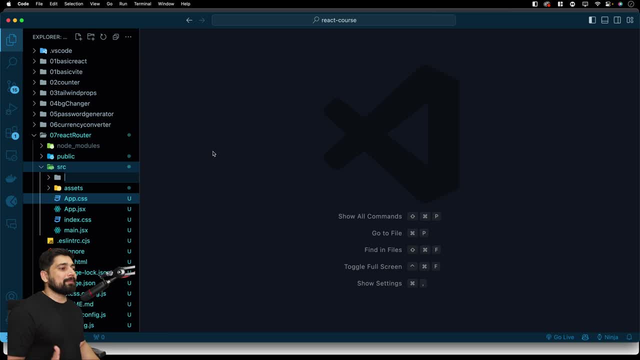 We'll start by calling this one as component. Eventually, as we go into the mega projects, we'll be designing components and pages as well. but these are just file names. Nothing really bothers us. So we'll be calling this one as components. 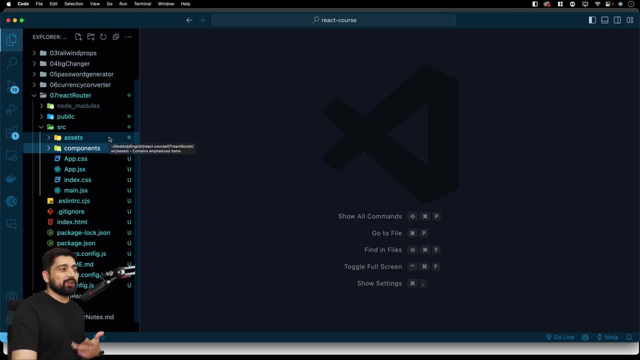 And this is just a directory structure. Each one, each instruction structure, each one, each one, each instructor is going to give you their best or their practices, which is being used in their company. We'll be creating a couple of folders first. 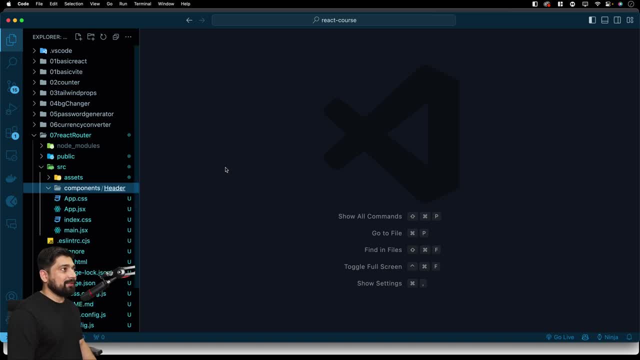 and then we'll be going through with that. First of all, let's go ahead and call this one as header. Inside the header, I will have a new file and I'll call this one obviously as a headerjsx. Now, nothing much in this file. 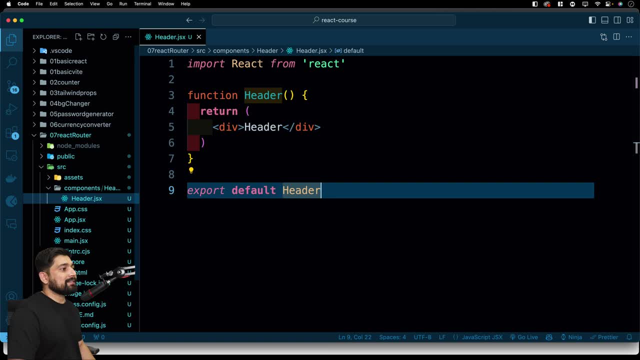 I'll just say this is a div which says header. That is it, absolutely that, nothing more than that. Now, similarly, in the component, there will be a new folder And we'll be calling this one as footer. Inside the footer we'll be having a new file. 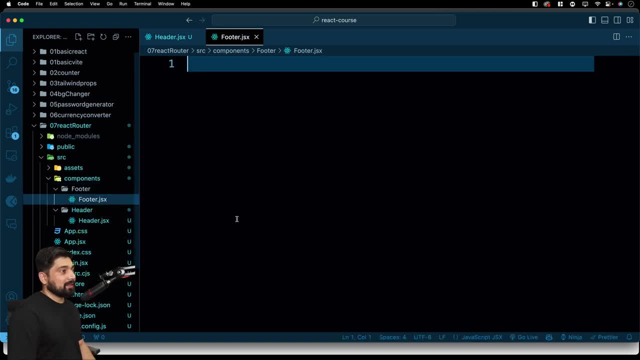 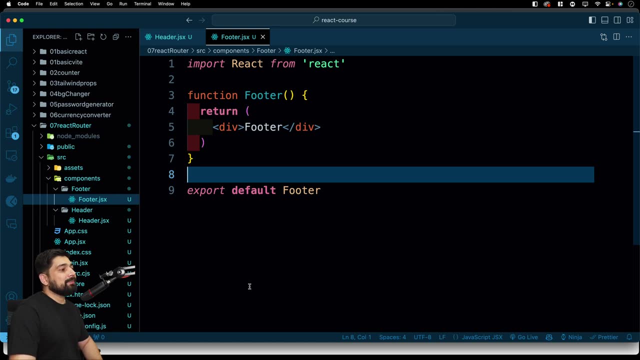 which we are going to call footerjsx. There we go R-F-C-E- we have just footer. This will help us to understand some of the main concepts of how things are actually being done or how things are being laid out. All right now, the next thing that we are going to do, 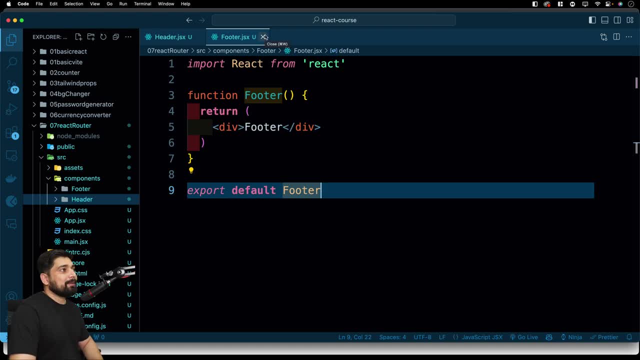 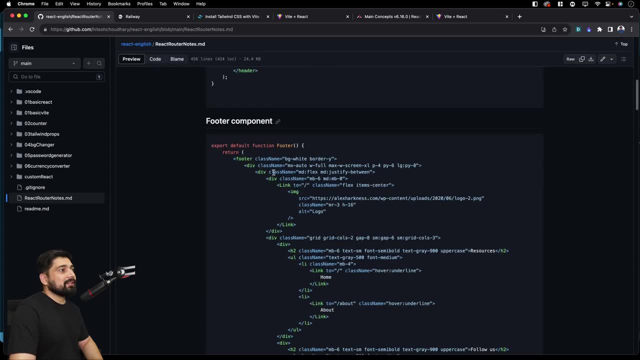 is, once we have these headers and footers, we will be replacing them with the notes that we have because, if you remember, this is where actually our component comes up. This is where the header goes, this is where the footer component goes. 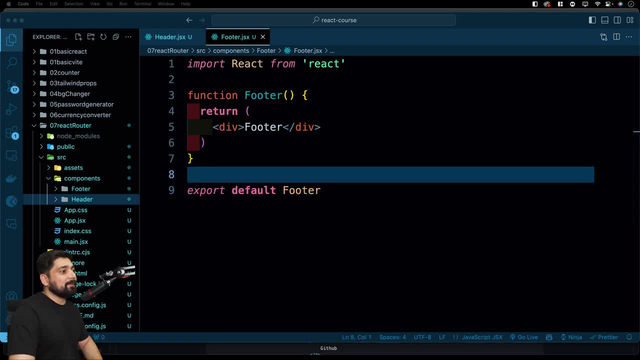 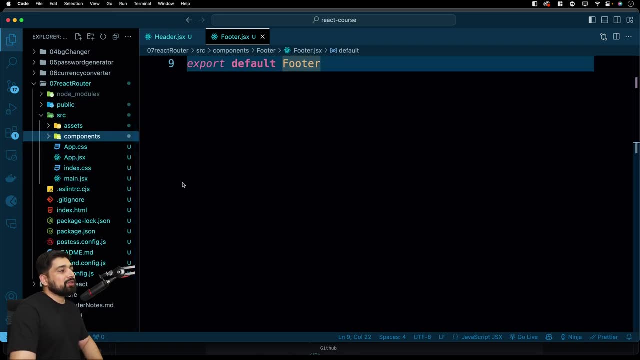 and we'll be talking about them as well, But right now, this is all what we have Now. after this, what we're going to do is this component: we'll be closing it down In our main directory. what we're going to do is: 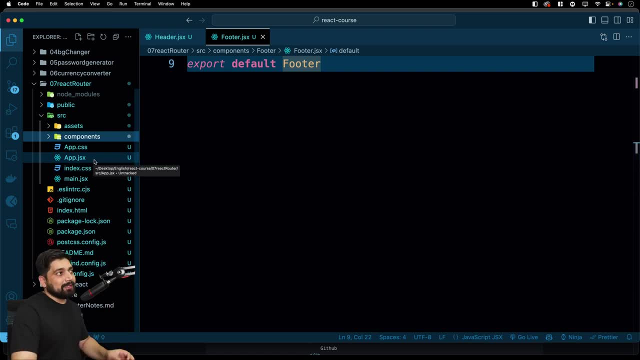 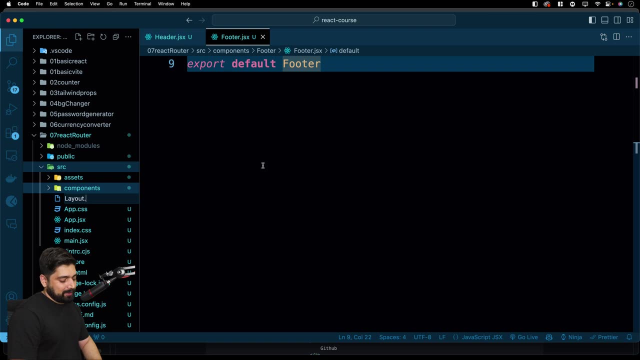 we won't be using this appjsx- although you can no big deal there- but I'll be creating one more file inside this, which will be directly known as layout, And this is a common practice. The reason for creating this file is in our application. 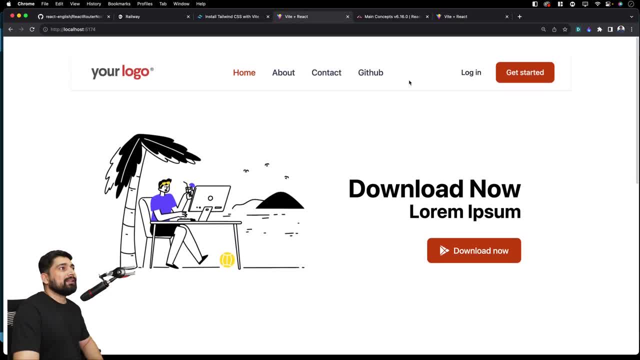 you'll see that, especially in this one, that the header always remains same, the footer always remains same, only the inner content changes from home to about and all of that. So we need to figure out a way that we don't have to repeat ourselves that often. 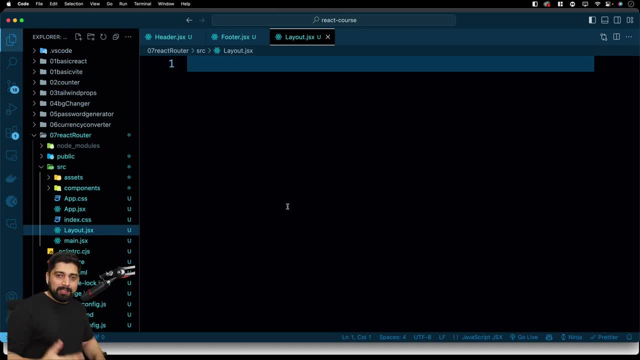 We just want to grab a header should always be there, footer should always be there and we'll be just injecting the content in between. That is a common practice. You'll find this exactly same pattern being used in the next shares and lot more stuff. 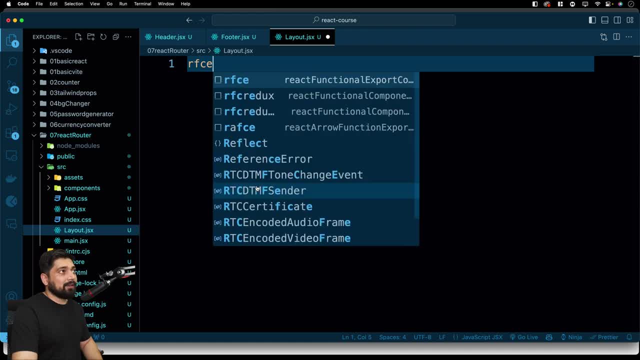 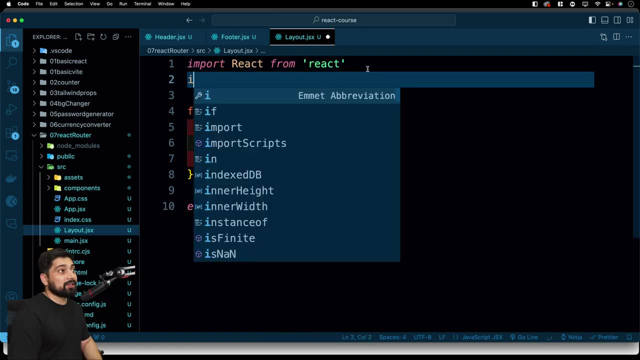 So we'll be using that practice exactly here. So we'll be using the same RFC React Functional Component which gives me a layout exported. that's it, But what? additionally? we can actually go ahead and use the first concept about this. 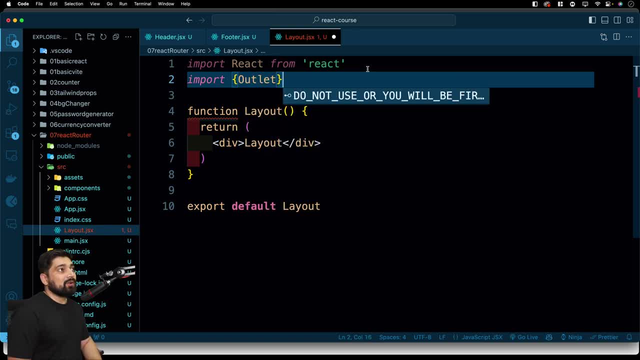 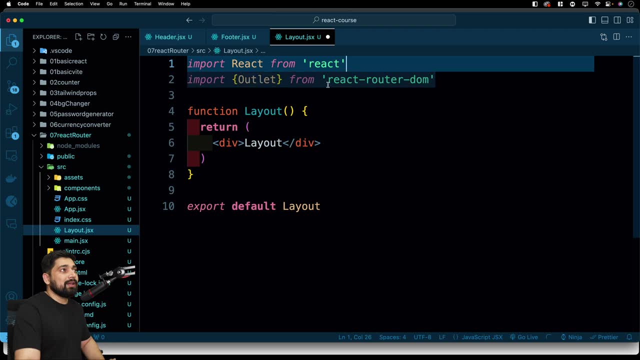 which you'll be using is known as outlet. This outlet is a special thing which is coming up from React Router DOM. Remember, so far we have been using just the React or the React DOM, but this actually comes from React Router DOM. 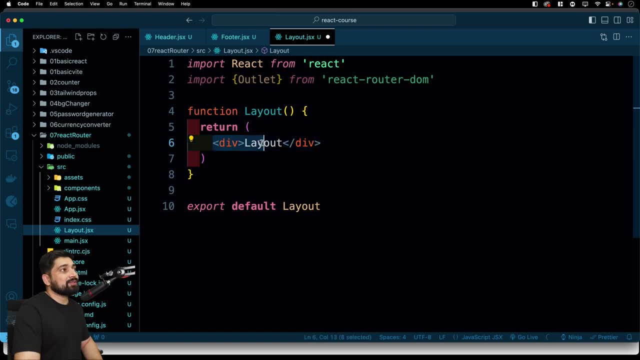 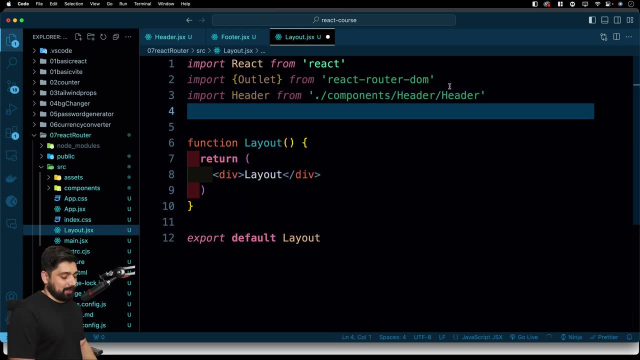 The advantage of this is that I can go ahead and return some special things. First of all, let me import them. I'll go ahead and say I need a header. Let's just say header comes up like this: I also need footer. 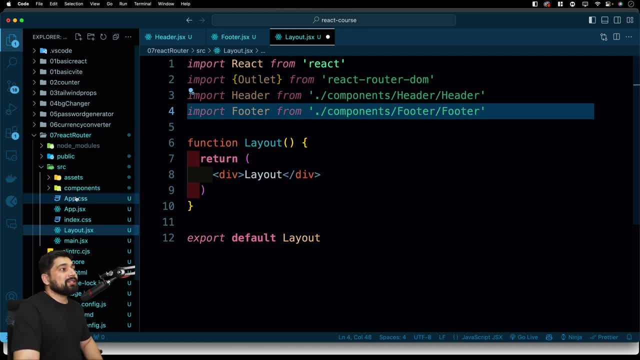 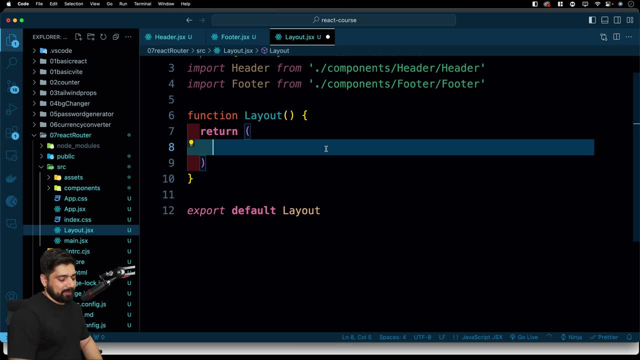 Footer also comes up like this. By the way, we can export these components into index file as well. That's totally your call. You can go ahead and do this Now here. what I'll do is I'll remove this. I'll inject just the fragments, just like this. 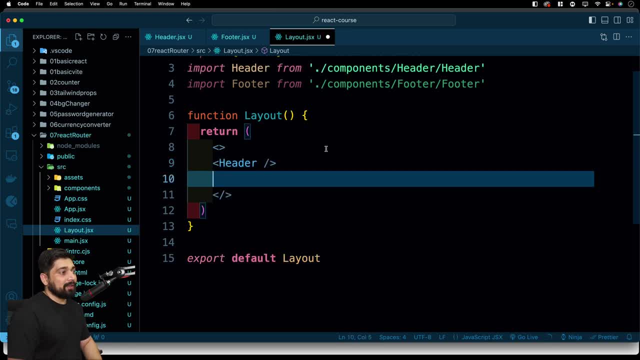 And I'll say: there should always be a header, All right, And there should always be a footer. So there we go, And now what I'll do is I'll inject a special thing, I'll inject a special element that is given to me. 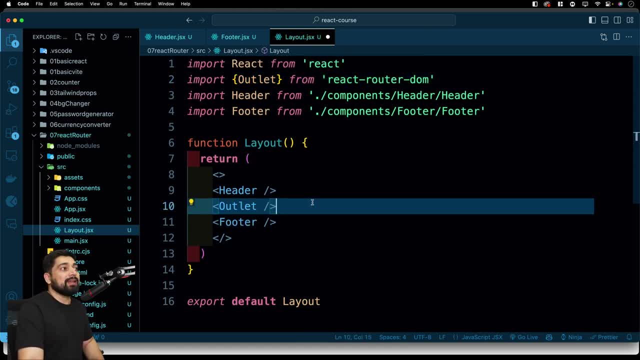 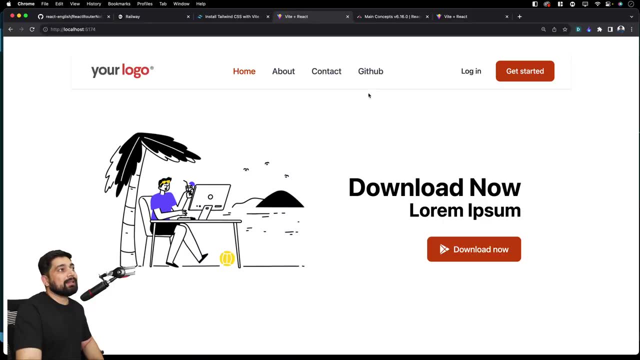 by the React Router DOM and call this one as outlet. It needs to be always called as outlet, There is no other name for it, And this is something which actually gives us this capability that, hey, this will always be on all the pages. 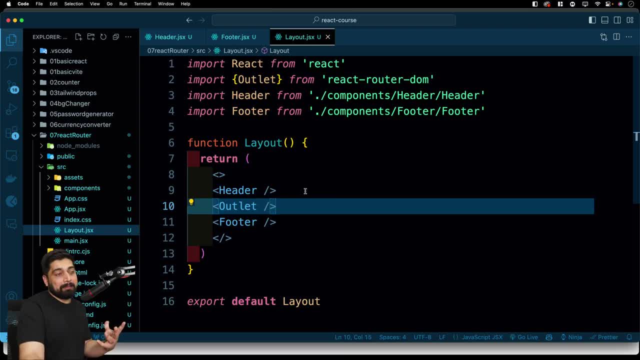 This one will be in all the pages. This is designing the layout of the application. Now, what's inside the header? what's inside the footer? that's not our call, but they will always be there And whatever the information that you are using, 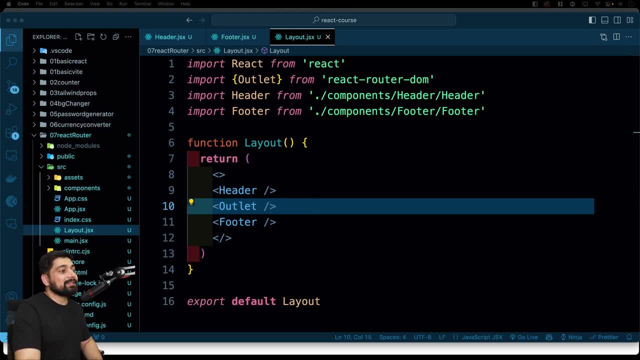 you can actually go ahead and use that. But the main question, then, is: how do I do this? And the main question that we have is that how it will know that we are actually doing this, Because right now, if I just open the application, 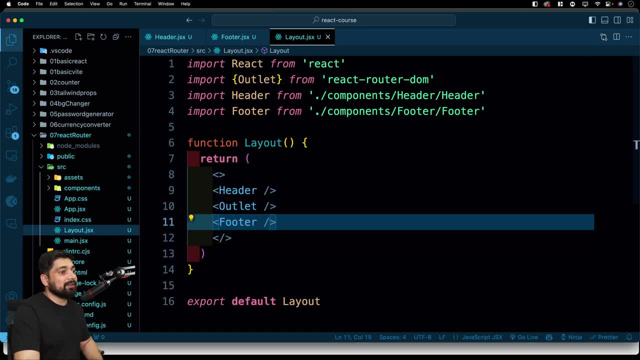 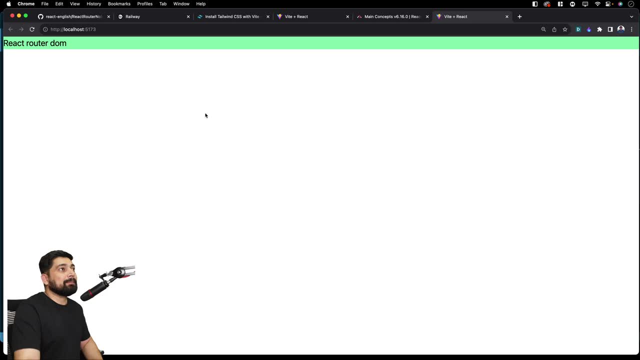 and I run this. this is not going to work, So it's already running. We don't need to worry on that part. If I go ahead and open this up in the Vite, it doesn't take place. It doesn't actually does anything. 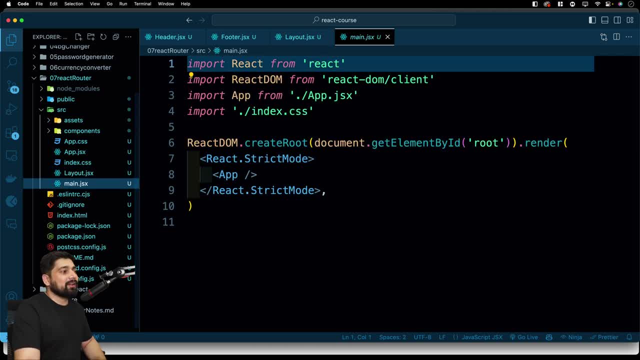 The reason for that is in the mainjsx or whatever your file is. in your case, whatever you're using, you are actually still serving app. It doesn't have the configuration which is required to actually have this router, And this router has a couple of ways. 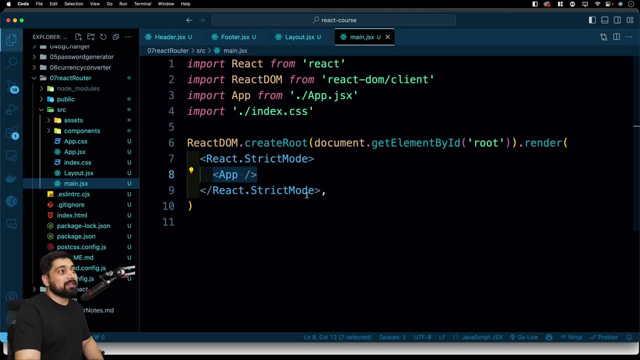 of how you can actually do the things. I'll show you both the ways which are actually mentioned in the documentation. So the first thing that we are going to do is keep this as it is. We don't want to touch it initially. 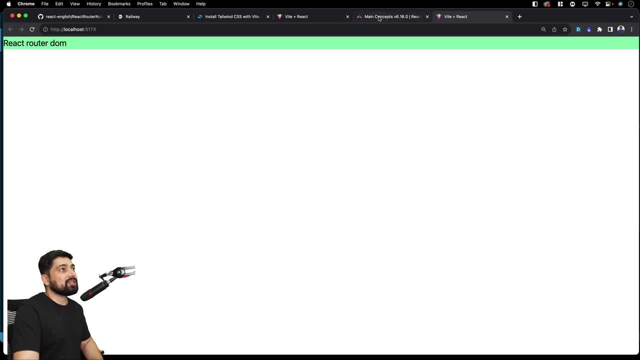 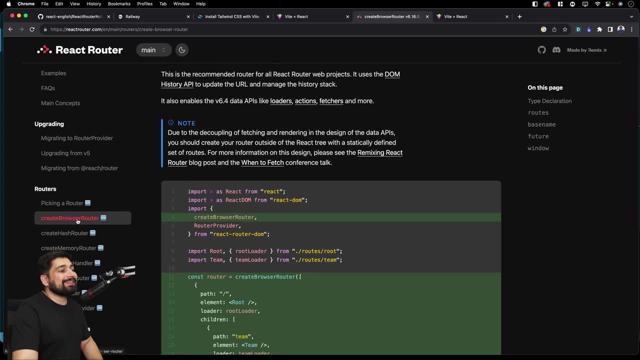 but we want to create a router, And this is the router which I showed you initially. that comes up from this create browser router. There are multiple types of router that you can use, but we'll be using this create browser router and we'll try to create a path like this. 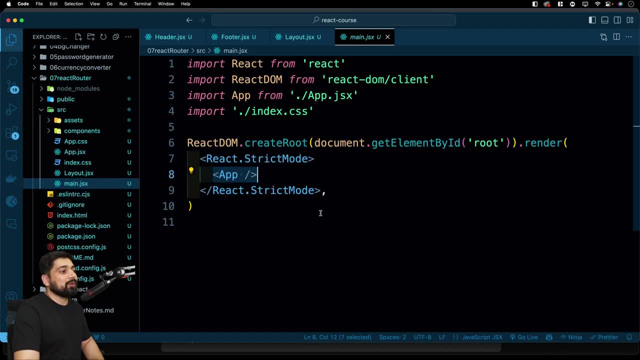 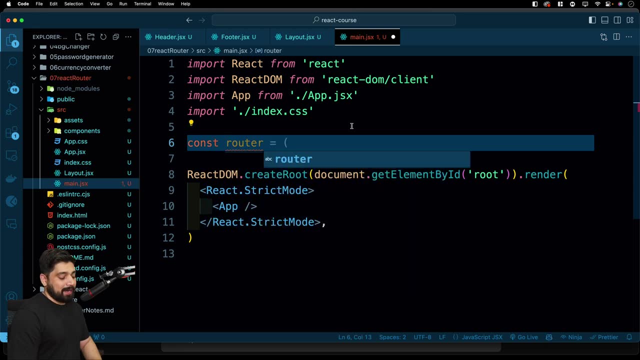 I'll show you. There's a syntax and there's another syntax as well. I'll show you the both. You can pick up whichever you like. So we can go ahead and create a router, So router and that router will be created. 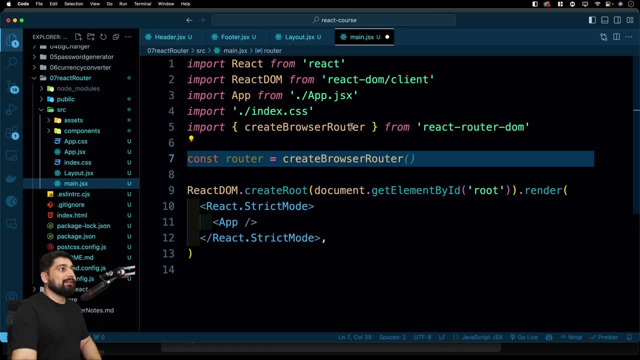 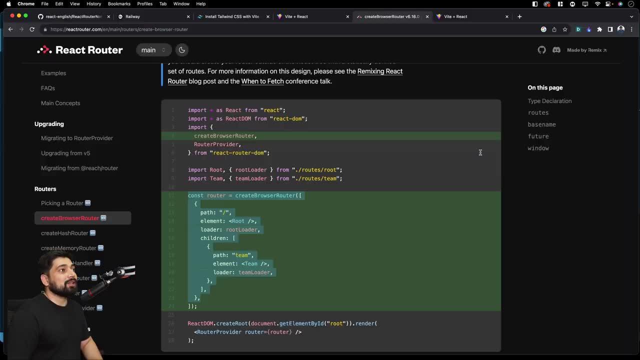 by create browser router. So again, create browser router comes from the React Router DOM. It's nothing, it's a function. But this is a function which doesn't work alone. If you look at the documentation, this function actually needs a route provider as well. 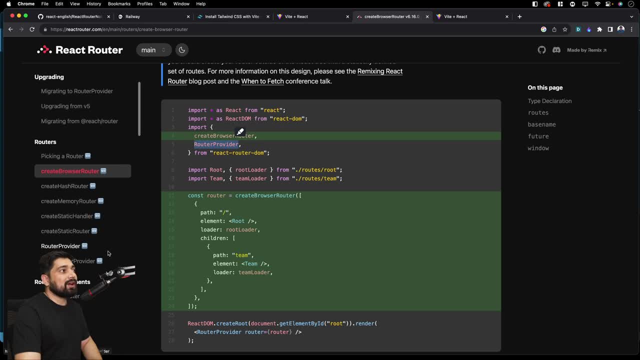 But it's not just the route provider. You can see there are lots of ways of how you can actually have the route provider: static route provider, create a static handler. There are a lot of ways- browser router. So this documentation is quite in-depth. 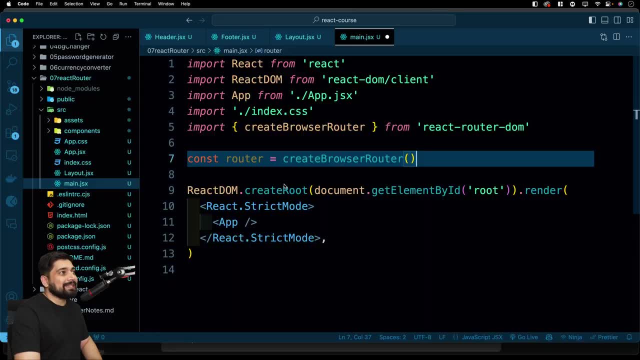 and there are multiple use cases for each one of them. I'll show you the most easiest one, that what accompanied. you need to create this one, And what we'll be doing is simply, we'll come here and we'll take this one as create browser router. 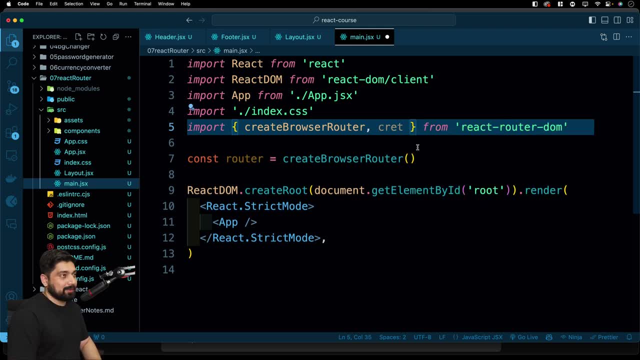 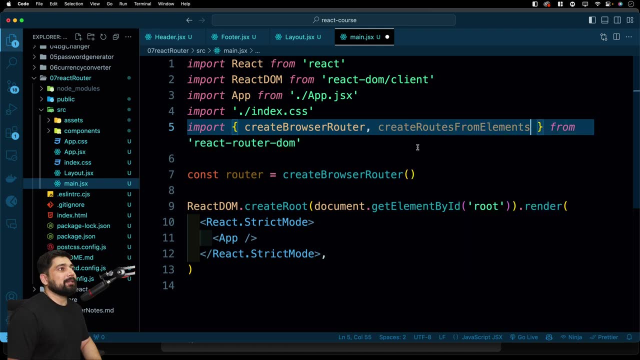 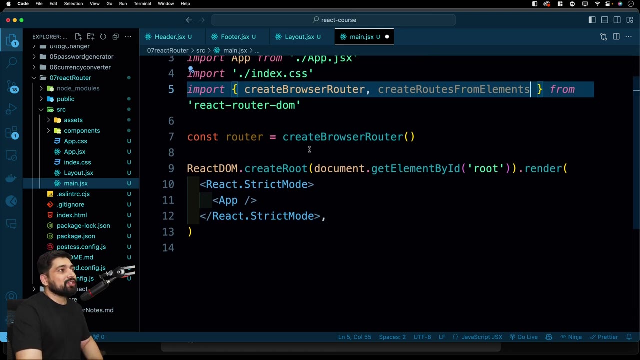 Oops, Create browser router is already there And we need create route elements. Yeah, create route from elements. yep, It's a little bit difficult to remember this one, but as you will do a couple of more projects, you will be familiar with that. 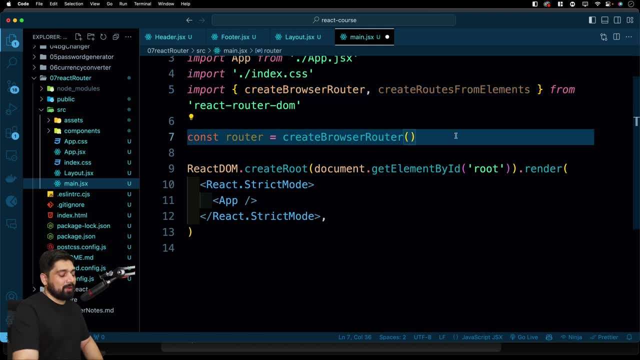 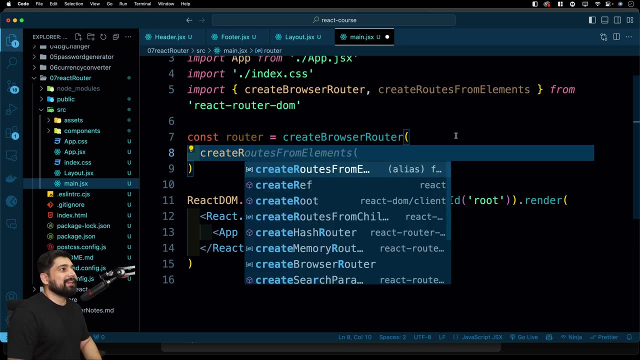 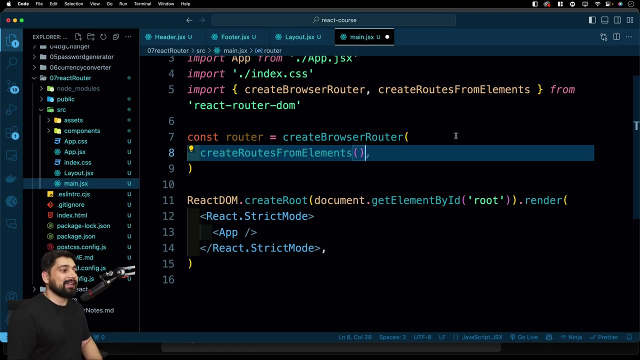 So once we have this create browser router, then inside this you can go ahead and use this, which is create browser. create routes- my bad- Create routes from element. This is again a method. No big deal there. Now, inside this, there's a syntax that you have to follow. 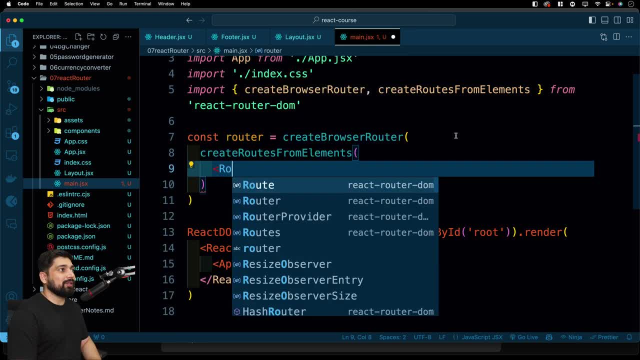 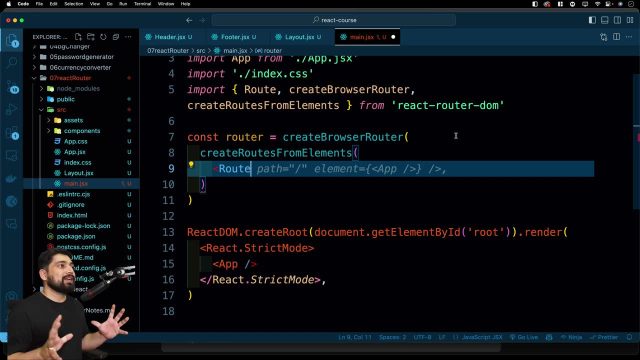 So I'll come back here. You need a special element known as route, And this route is obviously going to come from the React router DOM, And this route actually works like component itself. So, just like we saw that our empty components can have headers and footers, 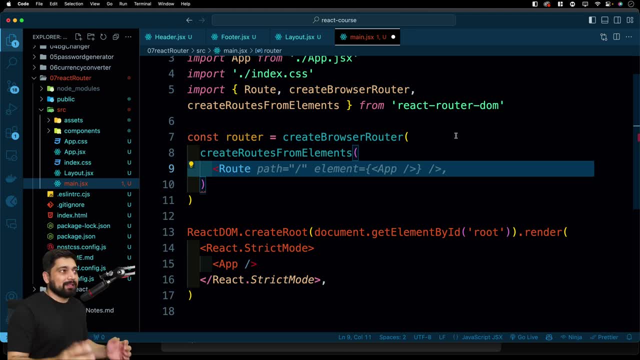 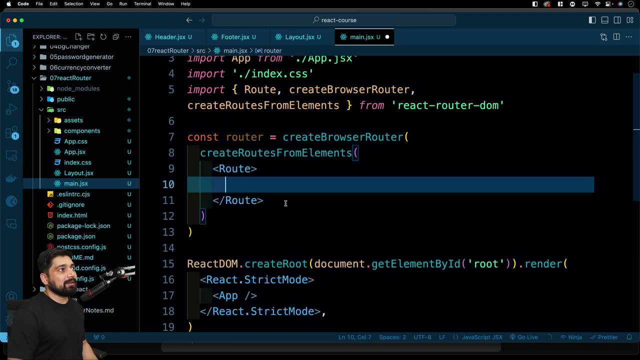 And we also saw that headers could wrap up inside footers and all these elements. So just like this route is nothing, it's just a component. So notice like this is how it works. So just a basic element, nothing more than that component. 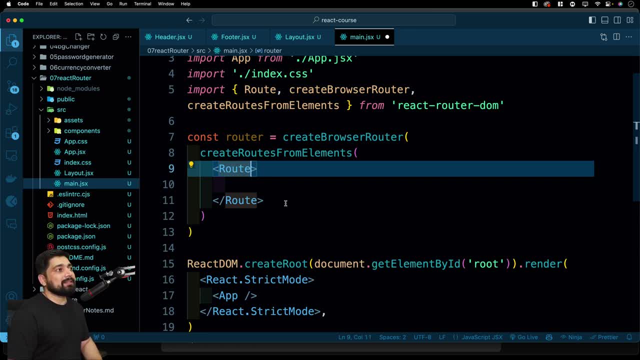 But this route actually takes a couple of parameters and, based on this, how it works. It works on this kind of a sandwich model that we have. So we'll first of all say that, hey, everything will go inside the path of a slash. 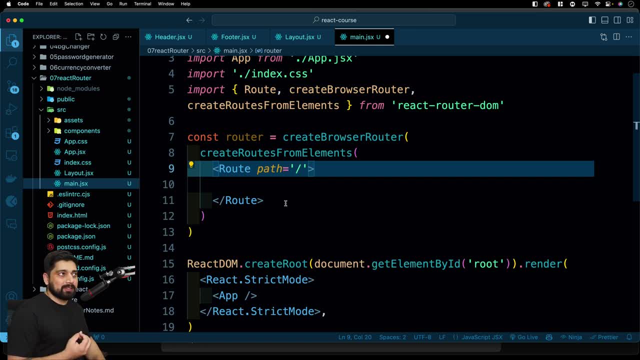 And what is the element that you want to load? Every single time you have to follow the same syntax. you have to tell it a path and what element to load in that path. Element simply means what components you want to load. In my case, I'll just say hey. 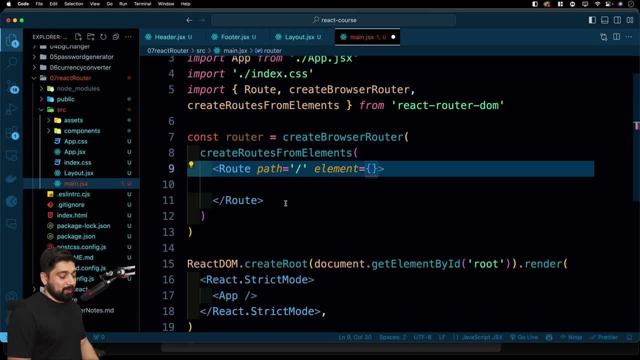 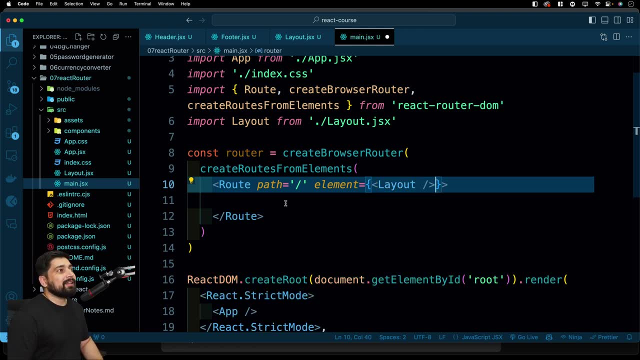 element that I want to load in this one. I'll give it like this: I want to load an element known as layout, And there we go, self-closing, of course. there we go Now. once I've done this, now things will actually take place. 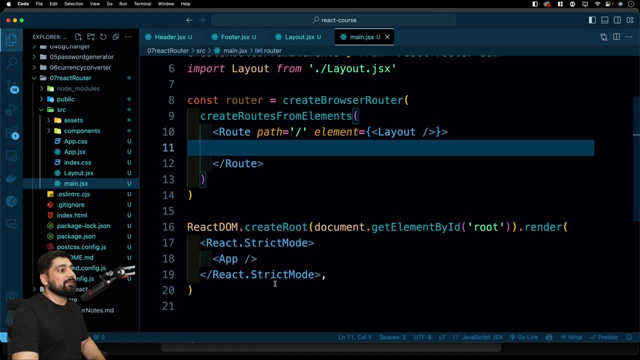 and instead of having this app, we want to use this router inside one here. So there's again a syntax, a little bit syntax for this one as well. We now don't want to use this app. We want to use our layout and want to load everything inside it. 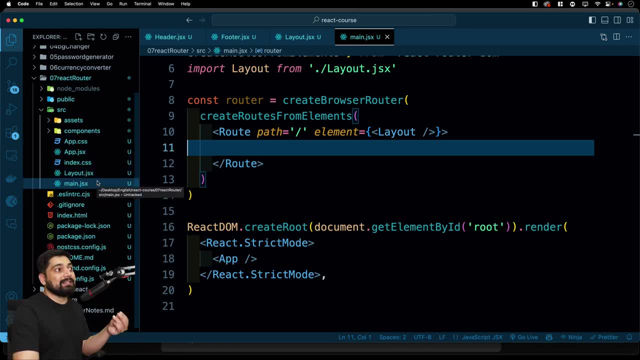 In fact, if we have the app, if we use the app, we want to load everything inside it. In fact, if we have the app, we want to load everything inside it. we want to load this inside the layout itself, so that the header and footer always remains. 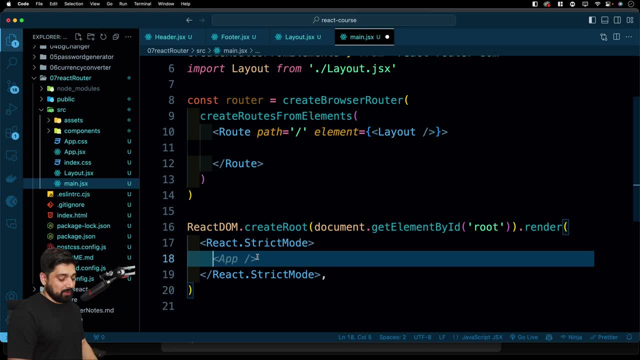 So we have to remove this here. This one goes away, This one doesn't load directly. In fact, we go ahead and use a router provider. here Again, router provider comes up from the React Router And the whole idea behind that. 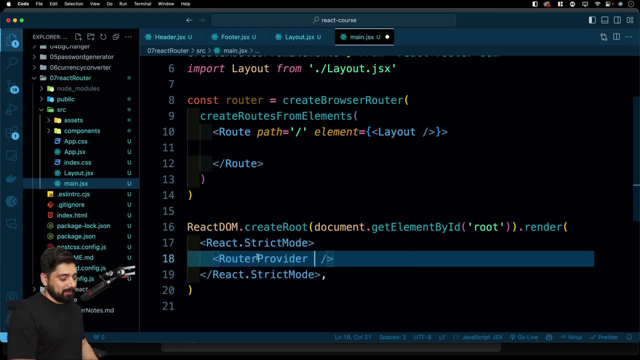 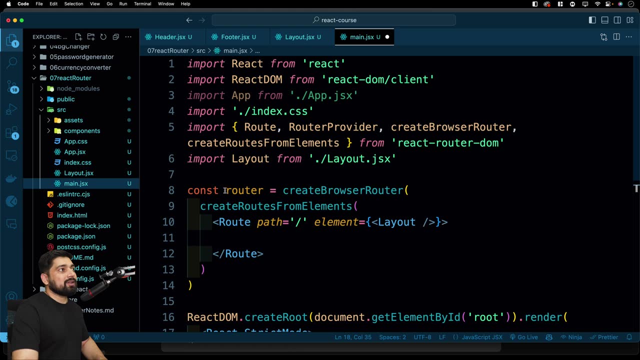 it's a self-closing element. You don't need to just have the ending one And inside this you provide just one param router, which is the router. Router is the property and is the router which we are creating. Make sure the router provider is getting operated. 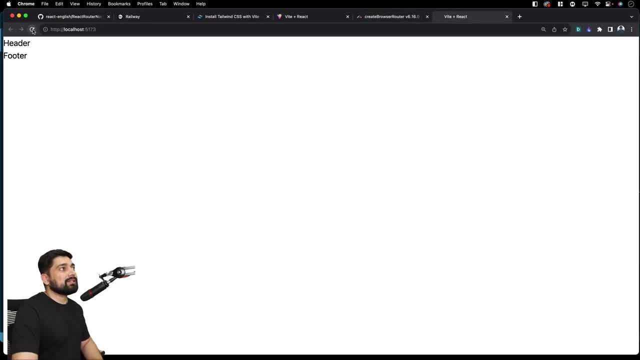 and is being taken care of. Once we have this now, what you'll notice is we have this header and footer, Since we haven't provided any outlet to this one. that's why only thing that's loading is header and footer. Now, in this one, you can add as much as you like. 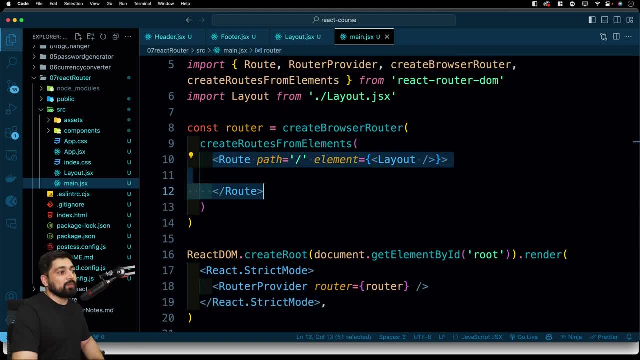 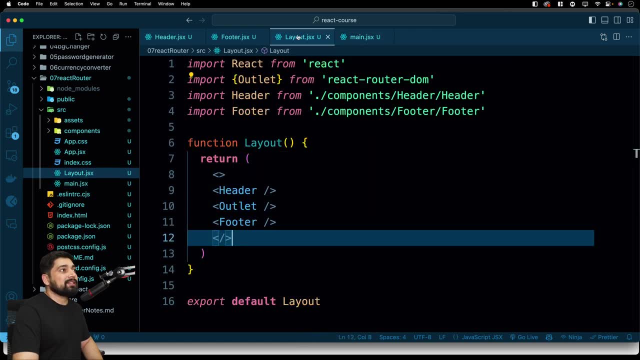 Now let's take care of this one here a little bit, since we have a couple of paths to work on with this one. So we have this route element and I told you this is like an element, like a sandwich that we have. We saw the sandwich kind of a thing here as well. 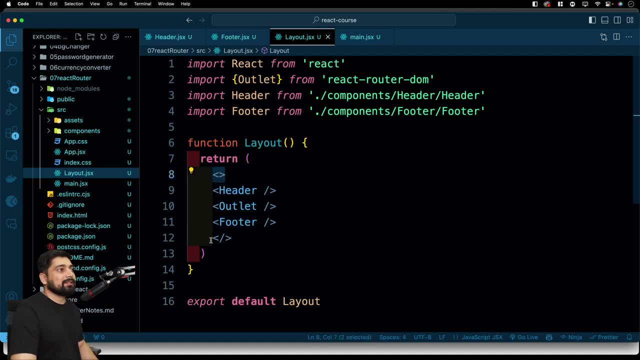 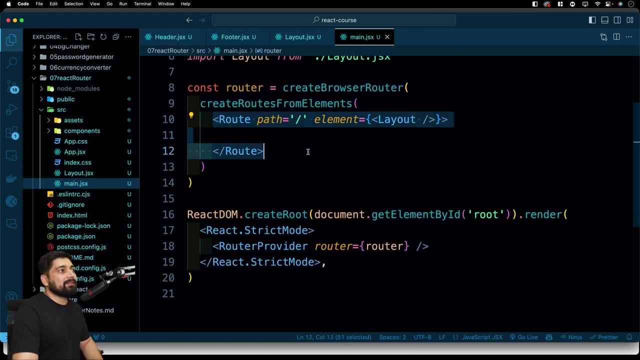 and we can actually use that. You might have seen that This is an opening. this is a closing one. Inside this, you can add as many as you like Similar to this. we have this one, but right now, the path that we are serving is this one. 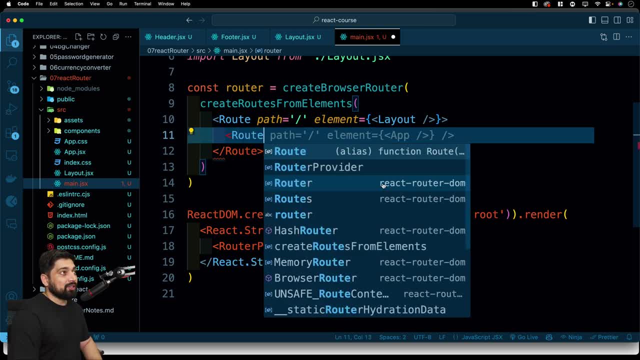 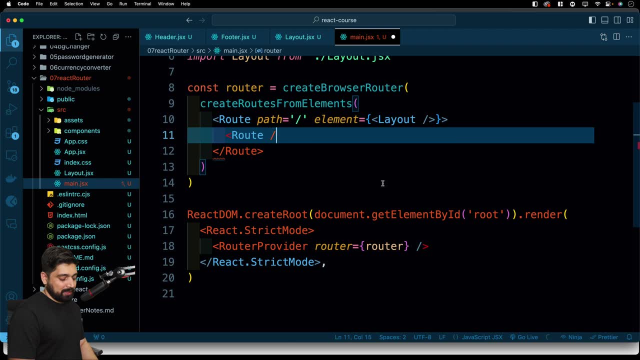 So inside this, you can have as many routes as you wish further. So these route, these route, could be self-closing or could be the sandwiching one, like this one, or you can have these ones as, like this, self-closing. 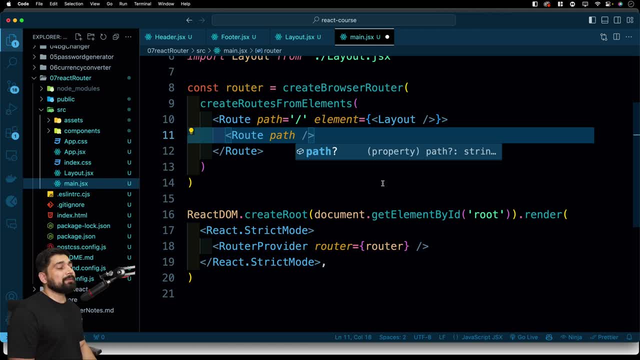 Now here's the interesting path. What path do you want to load? In this case, I want to load a path. I'll tell you in a minute what path to load: Single quotes, double quotes, whatever- But I don't have an element in this one to load. 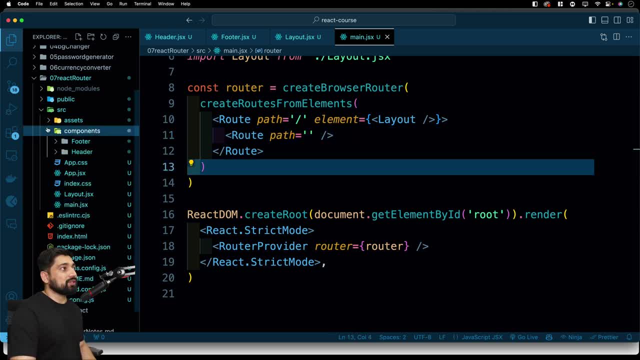 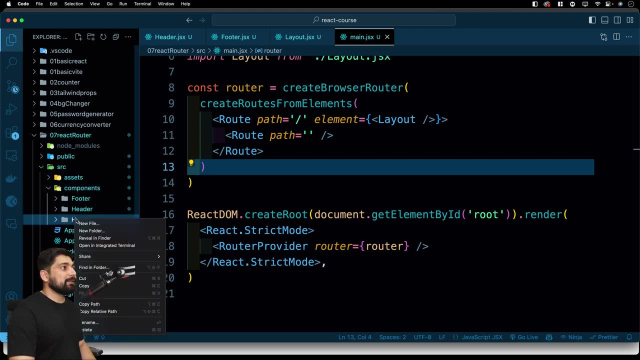 So what I'll do is I'll quickly go ahead and create another component in this one. So right click and we'll be creating a new folder. Let's call this one as home, Doesn't really matter, We'll be using the boilerplate code. 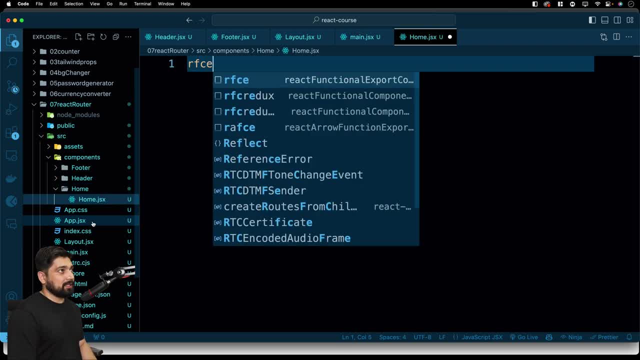 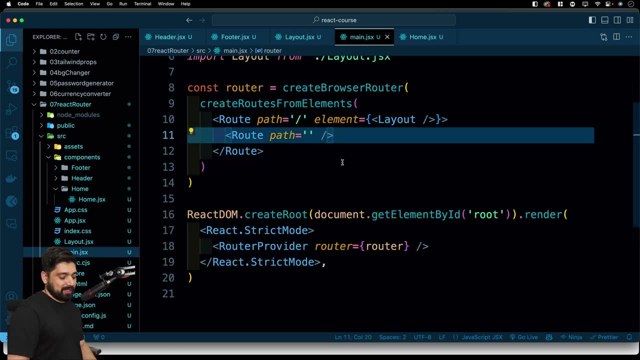 and we'll be saying homejsx And again RFC, that's it All. what we have is a home Text being literally written Now inside this. I don't say anything. I don't say a slash or anything further, because everything now happening is after the slash. 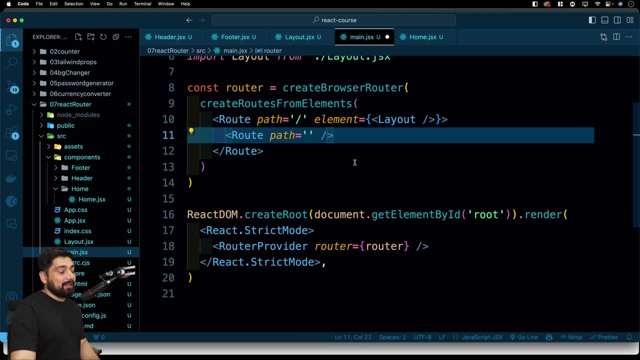 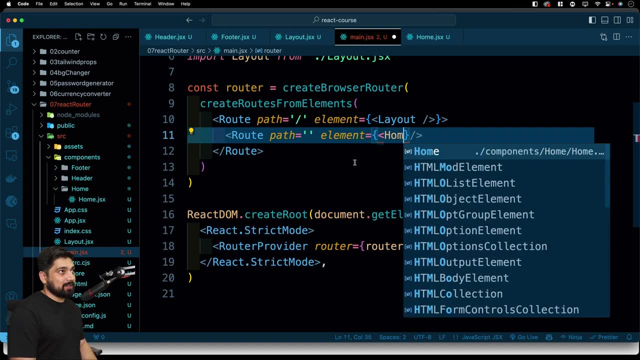 That's what the meaning of this first route at line number 10 is. Now, what element do you want to load? I want to load an element which is home. So I'll just go ahead and say: hey, give me an element which is home and self-closing. 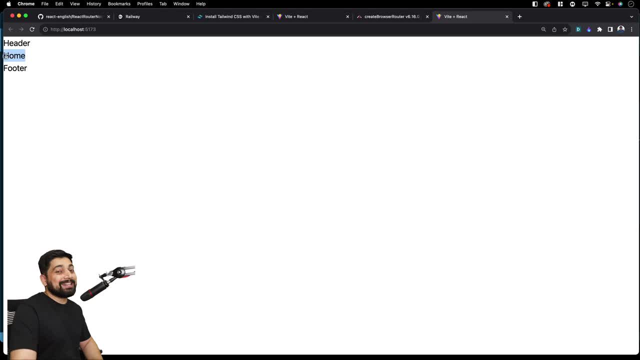 Now, when I go back- notice here- the home element gets loaded. So that is the advantage of this one. In the basic layout. notice here- I'm actually at the slash, So this is technically slash, which is where I'm home is loading. 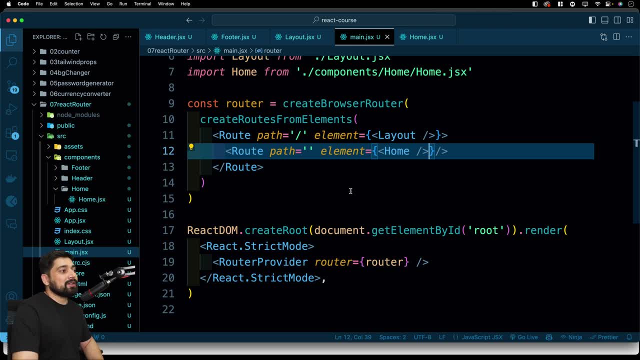 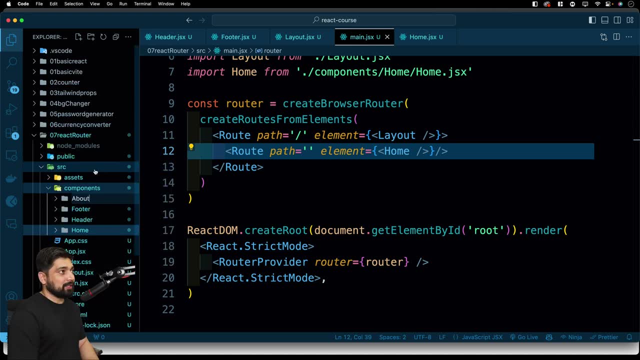 Now let's just say, for an example sake, you want to have a router which says about: So again, first create that component itself. So we'll create a new folder, We'll call this one as about, And right click and create a new file. 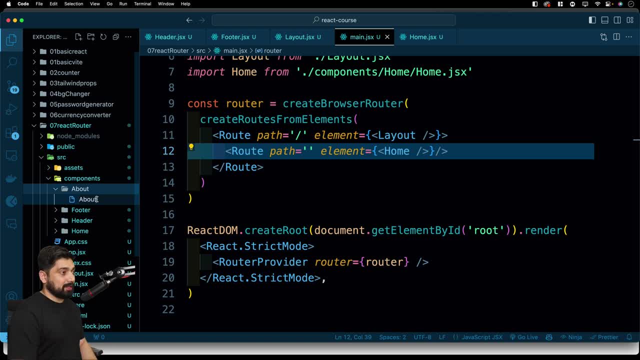 Let's call this one as about aboutjsx, of course, And RFC, nothing. It just says about literally nothing else. You guessed it right Now, after the slash on the home route, this works, but I want slash about to load that component. 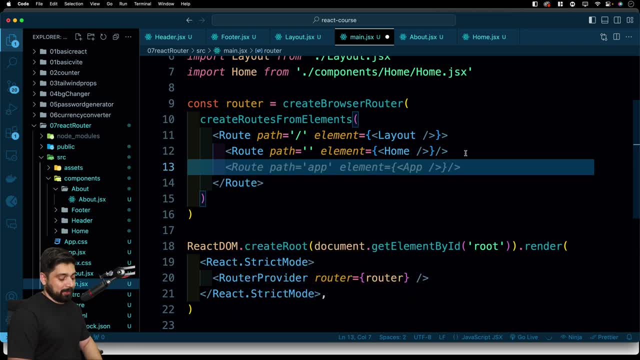 Again, go back here and simply say: route Again, this will be a component, So route, self-closing could be fine here. And then simply we will have a path which is going to be like this: This one is going to be saying at this time: 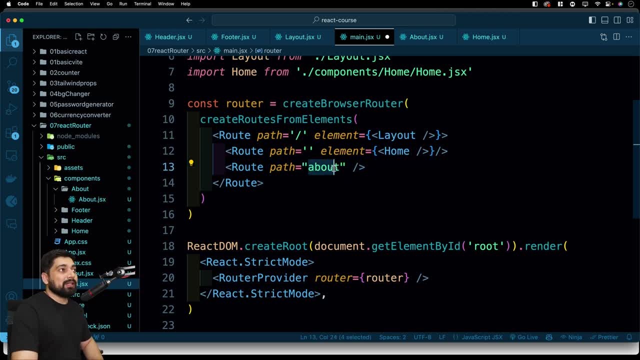 we need to change it. as about, Remember we are saying about here, but this about is after the slash, because it is sandwiching that one, So sandwiching concept comes up here. So on the homepage we have given a layout, a layout, a route here too much difficult to spell. 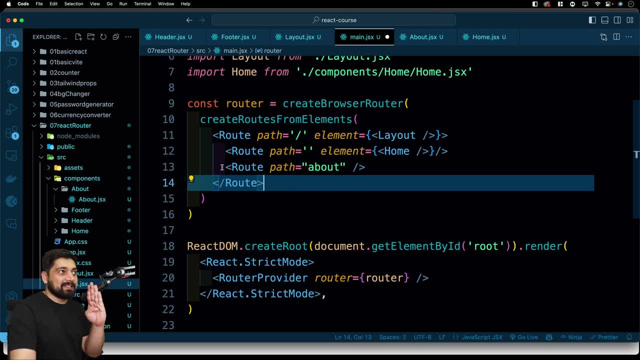 Here we are saying that on the same level, on the same hierarchies. after the slash: if I write about, remember I don't say slash about, otherwise it will be twice. I just say about what element do you want to load? 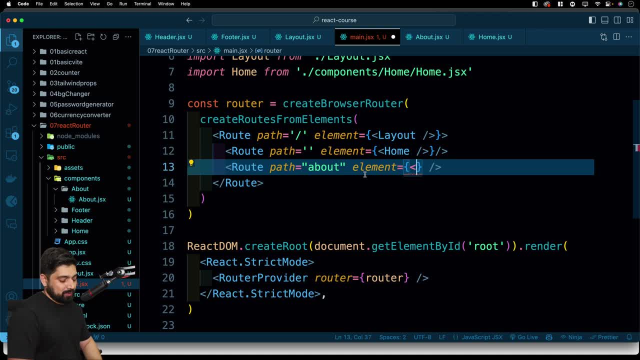 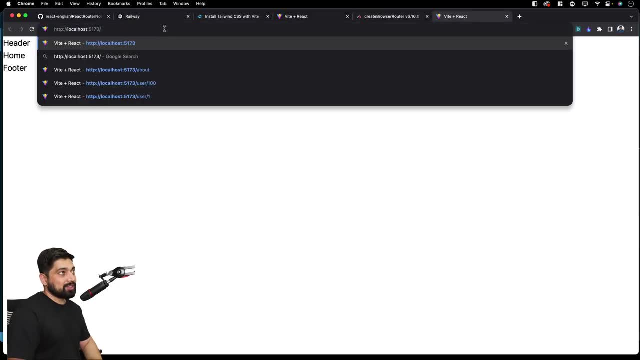 The element that I want to load is going to be like this, And this one is definitely going to be about: And there we go, self-closing. So now, technically, I'm going to say about aboutjsx. So now, technically, I can go on to slash. 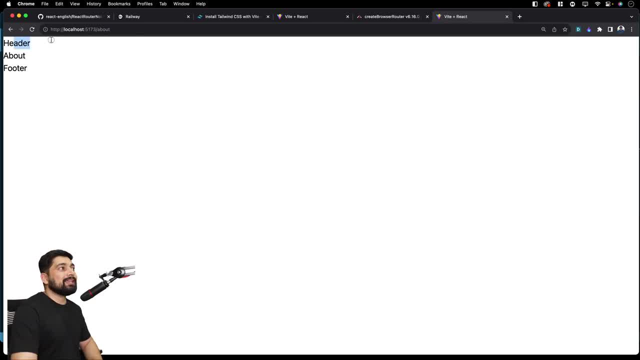 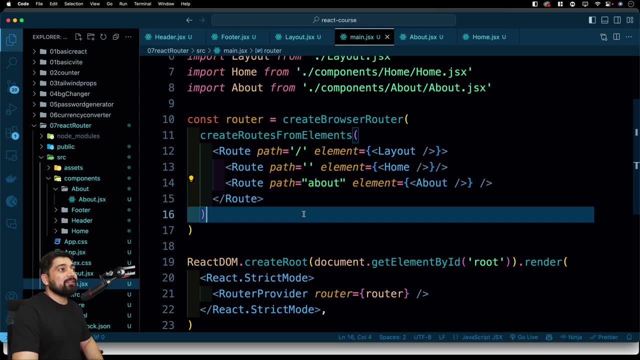 and I can just go ahead and say about Notice here, header and footer remain same, but my about changes. So I can go back. this is home. So this is the whole idea, whole concept. If you want to go further into this, 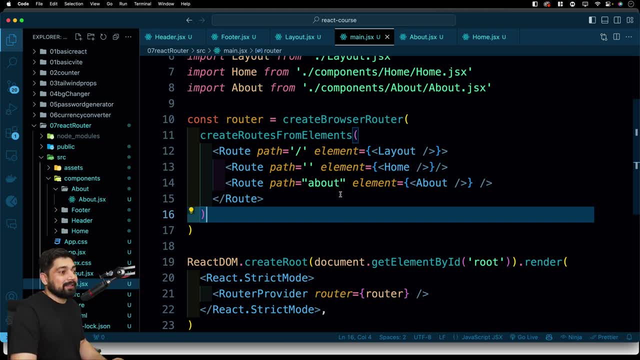 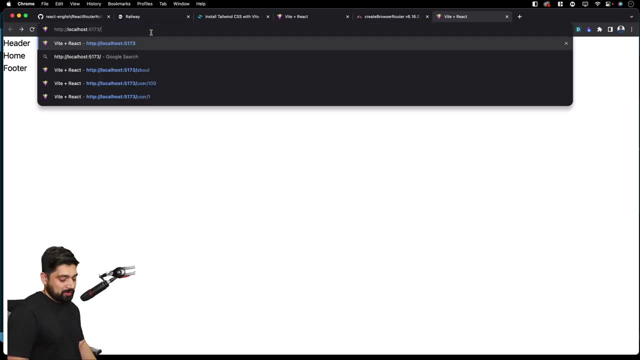 that I want about, and then after that some slash or something like that. then obviously you can go ahead and say that, hey, this is my about and slash, This is where I'll be loading this one. So notice, here I can still go on to slash about. 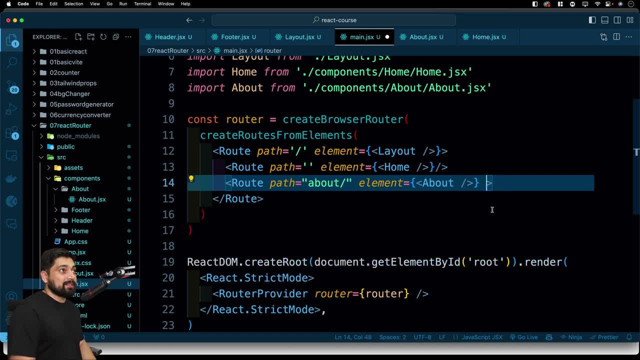 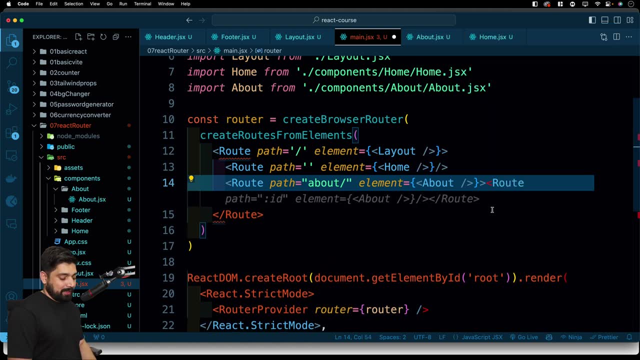 and it still works. If you want to have it like this again, use the sandwiching concepts. So in this case, I'll just go ahead and say: route, There we go And we'll end this one. Oops, my bad. 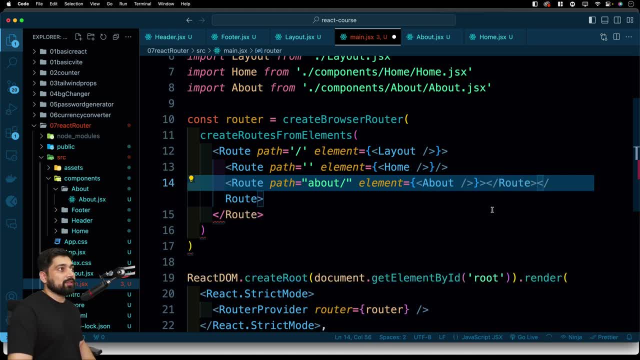 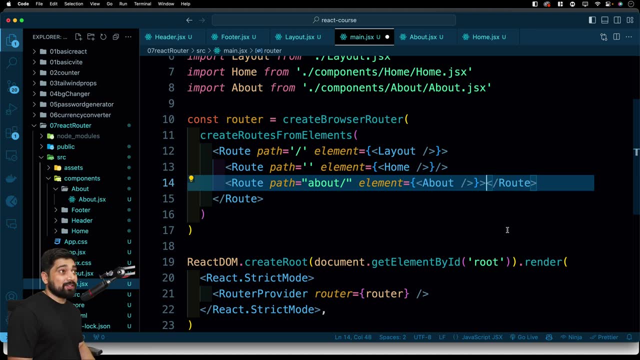 This one needs to go like this And we don't need this one. My bad, There we go. So now we have a closing one, closing partner of this one. Now I can go back and again start writing the elements, whatever that element is. 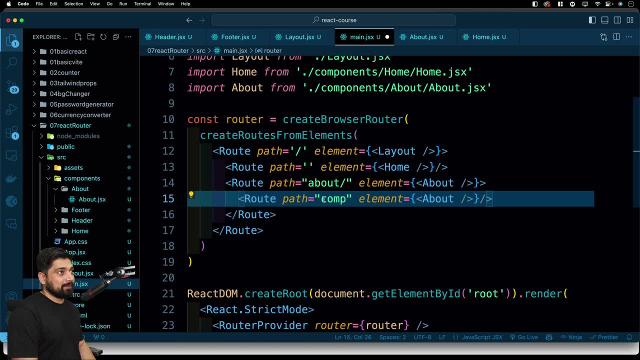 This could be about and this could be company, And I can load any element whatever I want. So just remember the concept of these sandwiching. So one things can be inside it. Whenever you need a further drill down path, you can do this. 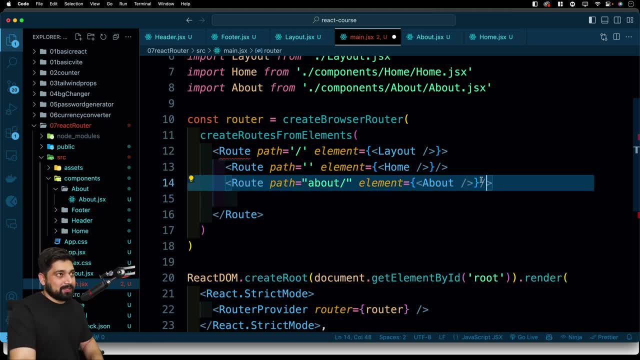 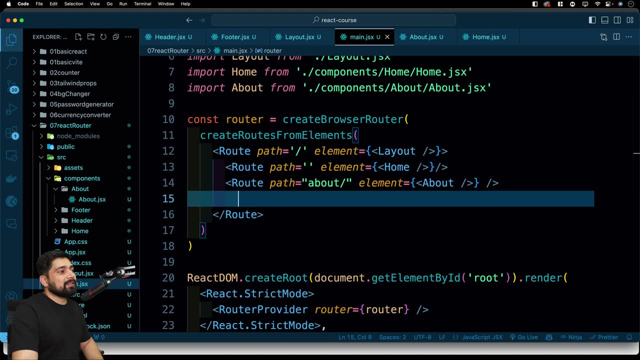 If you don't want to do this, just use a self-closing one. That's also the same. So you get the idea how the concept actually works. All right, So now we know the basic principle of how the things are there. 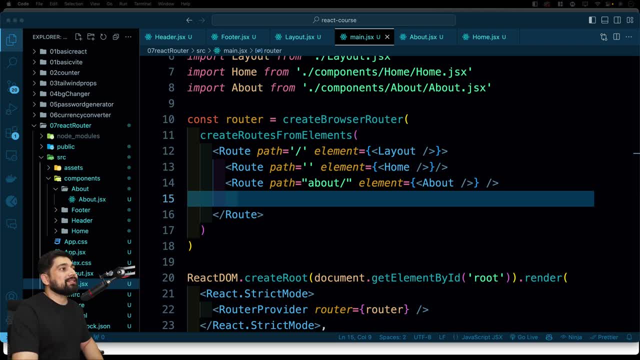 There are a couple of more principle that we need to actually go ahead and work on with this, And we need to have a small discussion on this one. Let's go on to the home, not home header. Let's go on to the home, not home header. 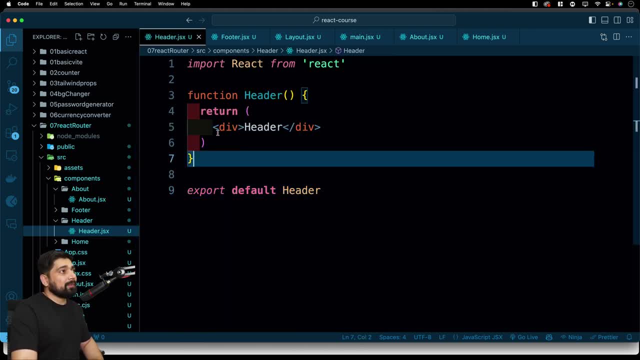 Let's go on to the home- not home- header. This is where we'll be working on, So again, we need to copy paste some of the CSS for this one, So we'll be grabbing all the. we can just go ahead and grab directly all of this. 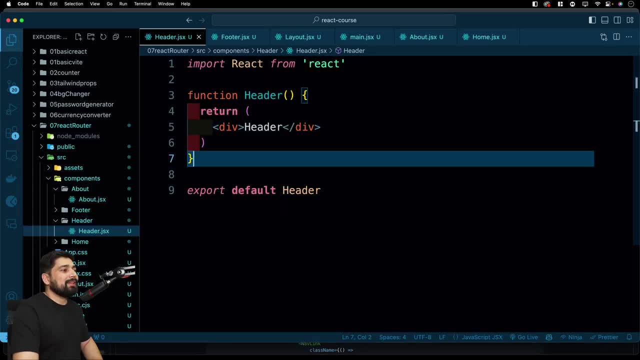 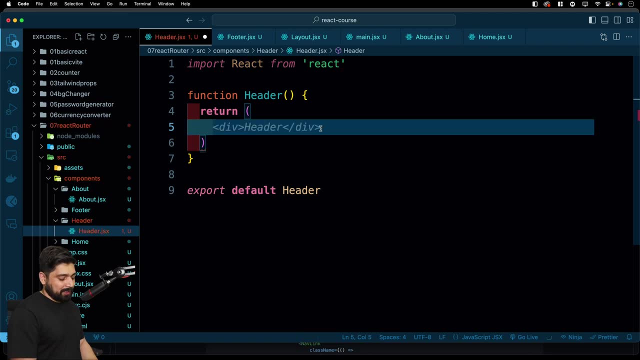 We have the header at the very top. We'll be doing that, but there are some elements which actually requires your attention into this part. So let's go ahead and grab, remove this one And we'll be having a simple header, just like this. 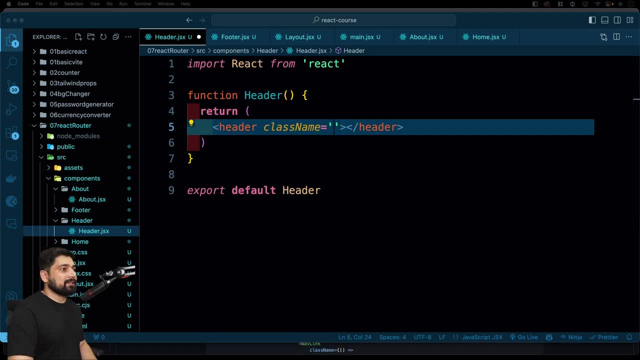 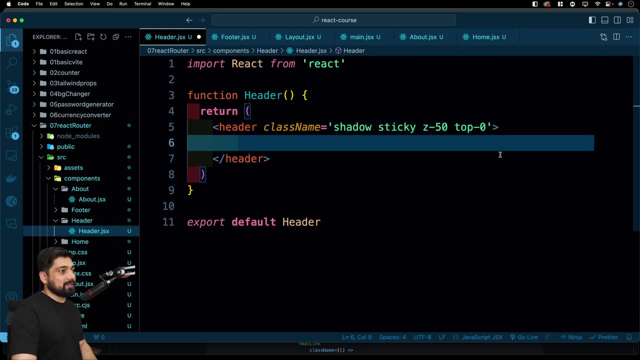 It will have a class name and I'll obviously copy and paste the class names. This is the part where it's a little boring, but don't worry, There are some interesting features here which we want to discuss. Then we have a nav which we are writing again: class name. 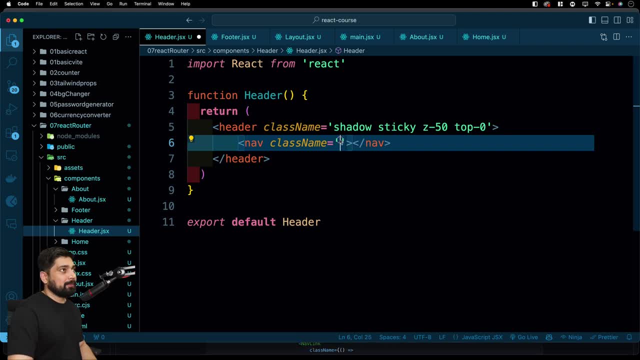 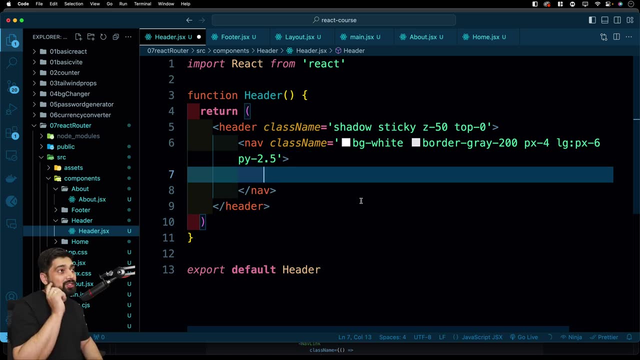 And again, the class name will remain same. So copy and paste that. So now that we have nav, inside the nav, we will be writing variety of links. Now your first intention would be just to use a tag. This is where things can go actually wrong. 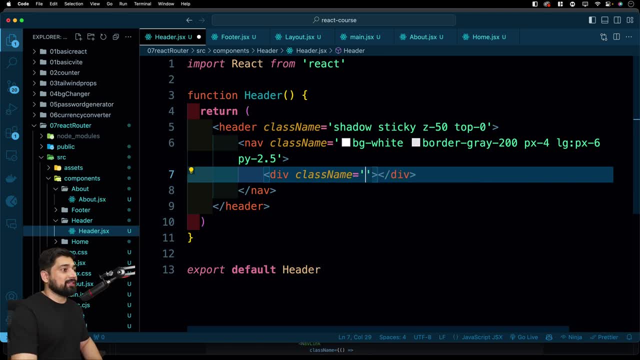 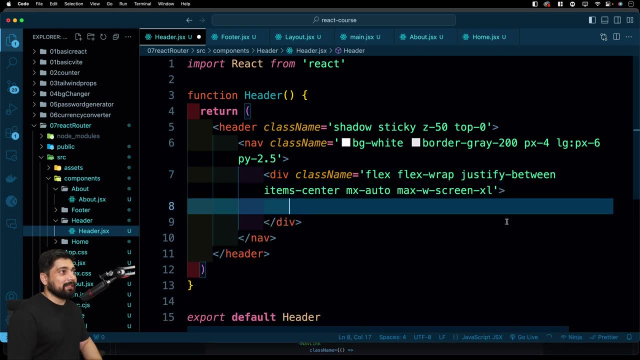 So I'll just have a div, another one here, because that's how we laid out while designing this. So I'll just have the class names, copy that, paste that up here And inside this div we have all the links. 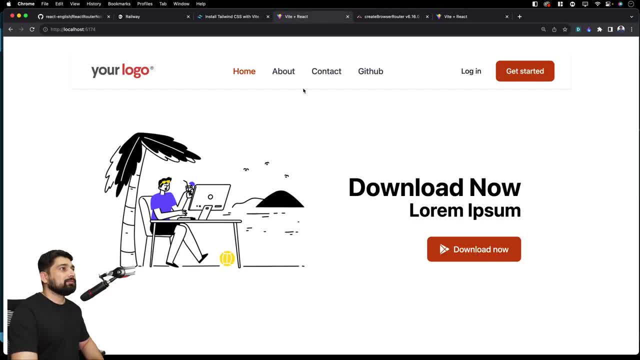 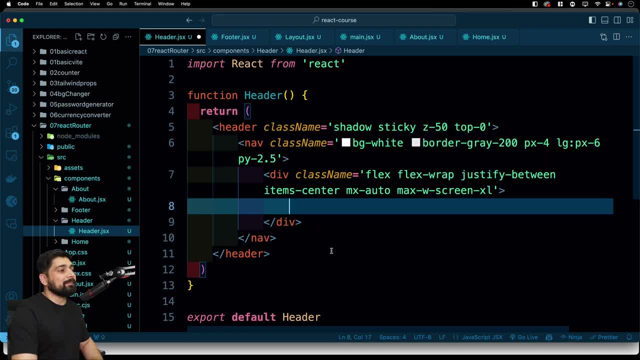 What you saw earlier on the webpage like here home about and all of that. So they are just, obviously, they are just links all inside this one, So we'll be using that. Now. the first intention is always go and use the a tag. 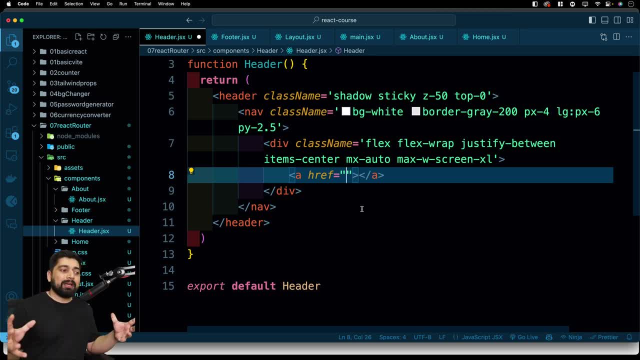 and just write this: Remember the a tag. the whole idea behind using the anchor tag is to move on to different resources. When you use a tag, the page actually reloads. it remounts because the control is given to the browser. 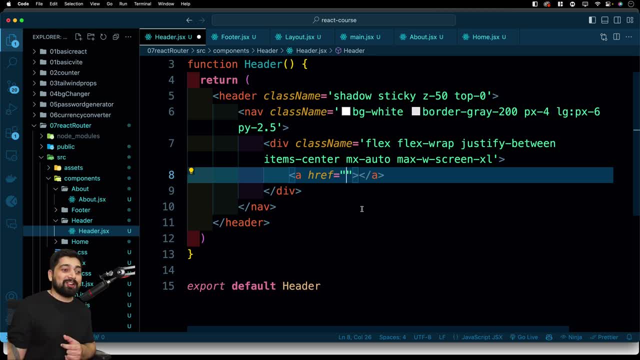 and the dom which is in the browser itself. We don't want that because page should not reload. It's a single page application And that is why every single router, no matter it's in Nextjs or React or wherever it is. 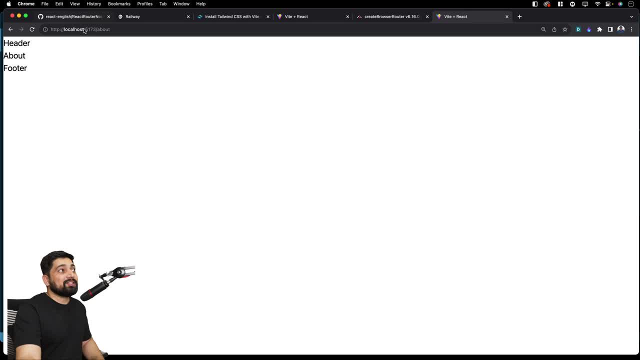 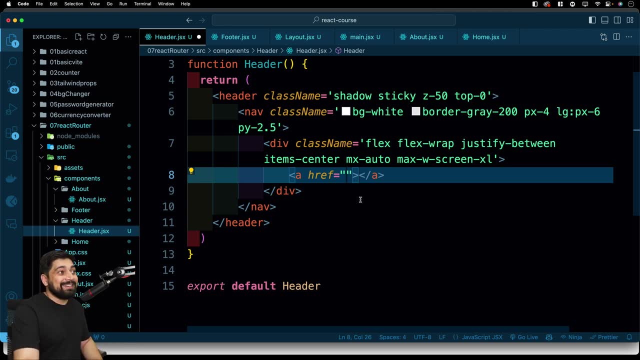 it is giving you some ways of navigating things Because, remember, this is all a facade, This is not real, This is just a simulation of moving, to slash about and wherever. It actually never goes there. So that is why, in every single time, you'll find: 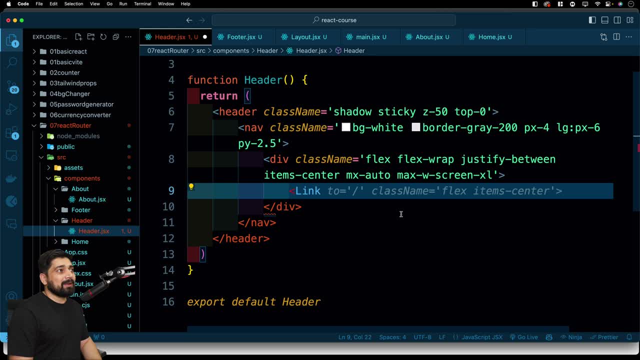 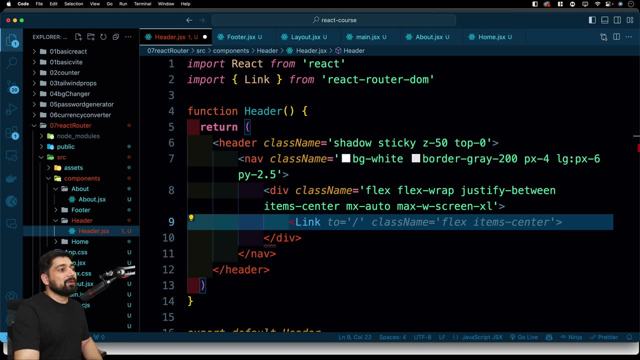 something known as link or somewhat similar to that which is actually coming up from, as you noticed here, React router dom. Remember, it always comes from React router dom or something like that, And we work through that. So in this case, we'll be just saying that. 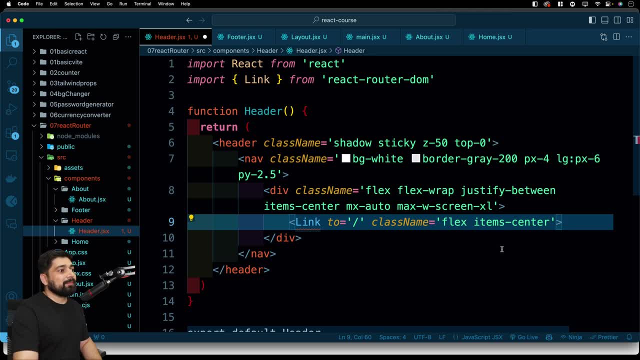 hey, we'll be having a link, And again this could be a self-closing one, or you can just go ahead and close it like this, So I can just go ahead and say slash link like this. Again, it could be self-closing. 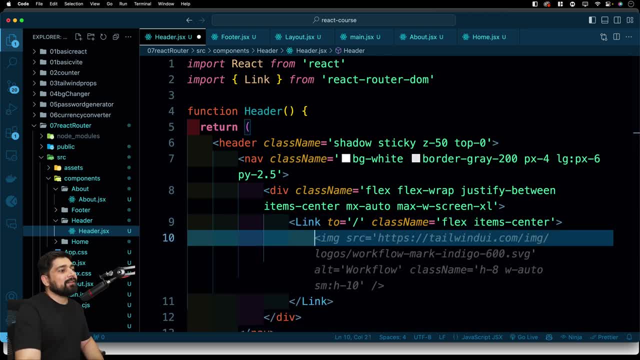 It could be like this: totally up to you. Now, in this link, what do you want to have? We have just an image. We have an image with the logo or something like this. So in the image part we are not talking that much. 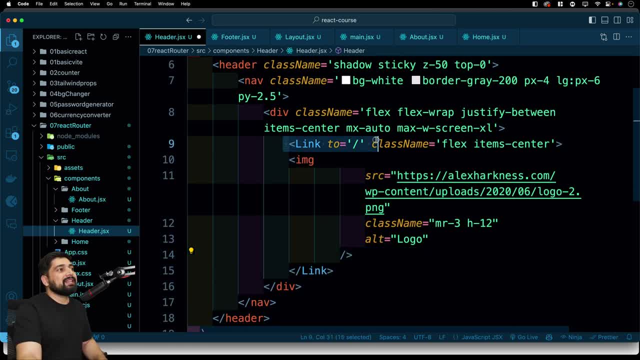 but yeah, we just added an image or something like this. But notice here, this link is pretty interesting. This is not your A tag. It doesn't have an href. It has, rather a tag of, known as two, and this two will take you wherever you like to go. 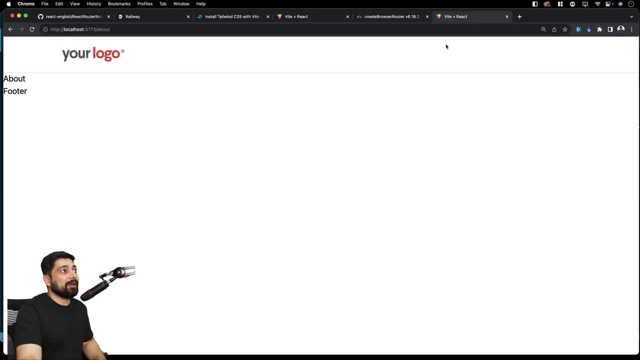 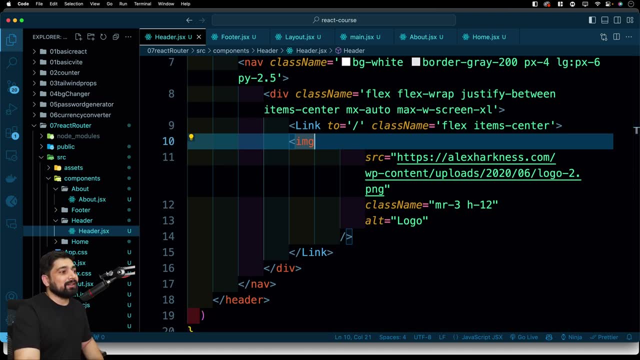 So this is the interesting part where you should pay attention. So if I go back up here, notice here, this logo comes up here, So simply go ahead and works on with that. We just found this random logo on the internet and we worked on with that. 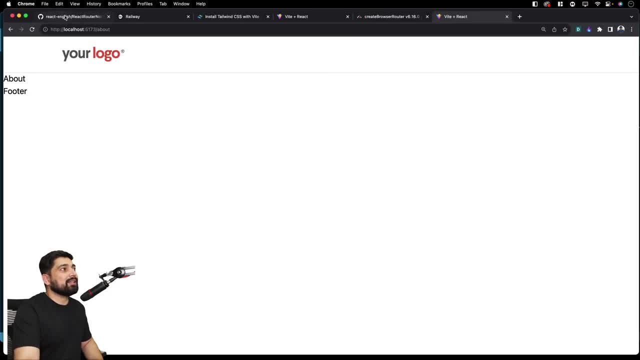 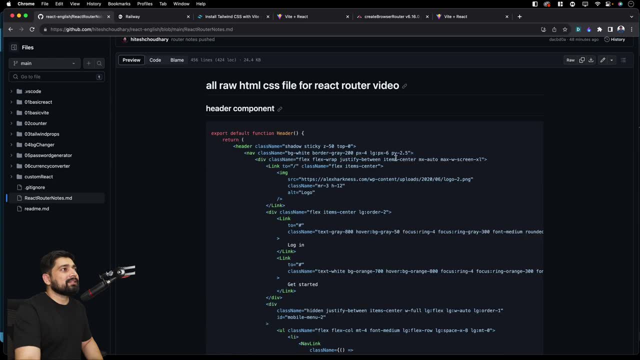 Now similar to this. you can actually have more of this. In fact, now I can go ahead and bring all of this header component up here. So if I just go back here, copy this exactly same thing, So I can just now replace and talk about it. 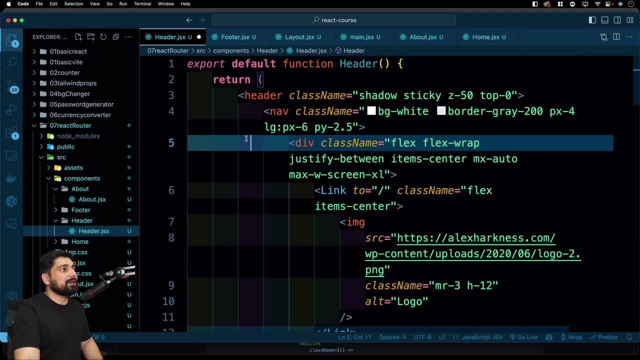 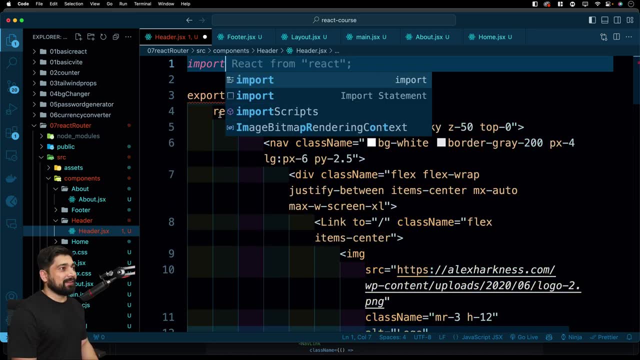 Paste this and we have exported default all of this, but the only thing that is still required is to import the links and all of that, Otherwise it will yell at you. So go ahead and import React. Do we need React? I don't think so. we need React. 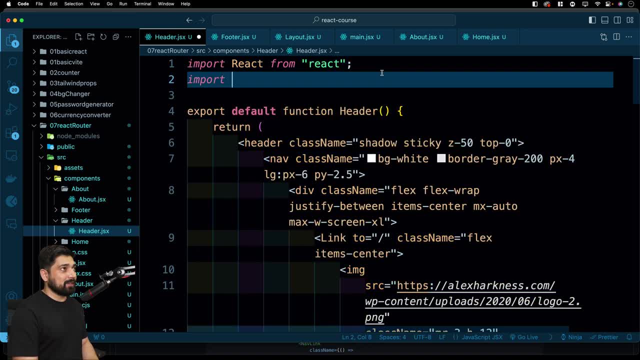 but still, if it is saying, I'll just grab it. We need link. definitely, because we discussed about it And the link is going to come from React router DOM and not only link. let me show you a couple of more stuff, So the link is actually one way of navigating. 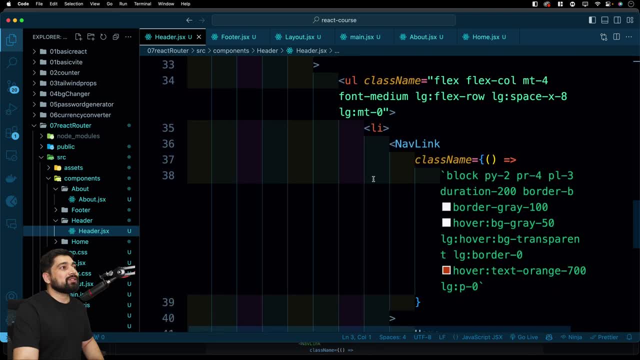 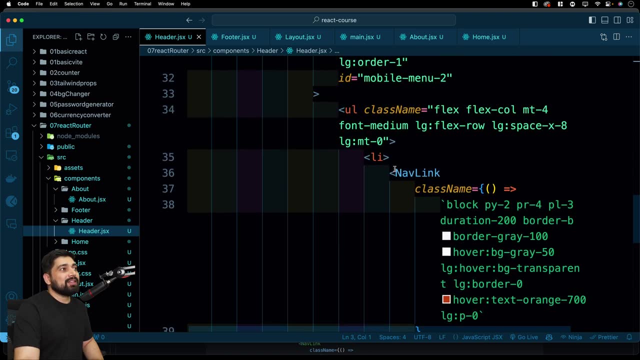 from one place to another place. So notice: here mostly the link is used, but there is also a nav link being used. So nav link is also a part like that. So navigation link: Right now we are just using it as a basic. 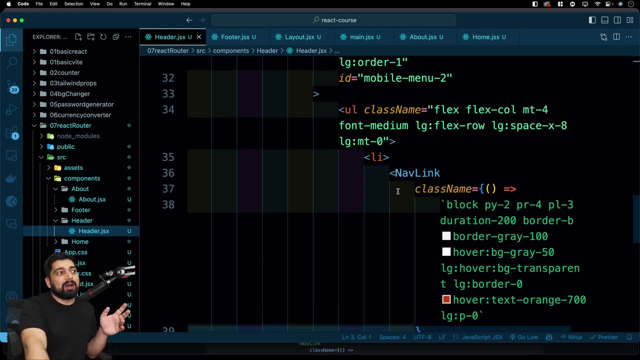 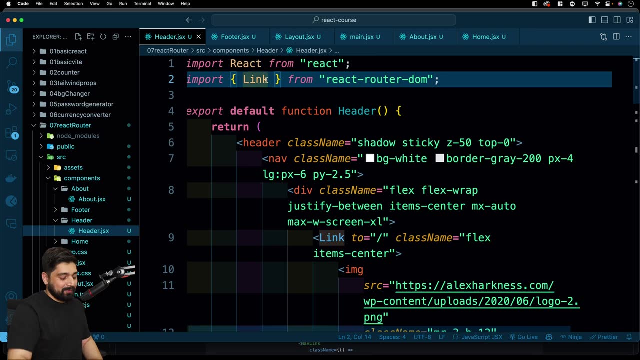 but nav link actually gives you a couple of more features, like on what page you are and what values you can actually use. So we'll see some of the variations and versions of that as well, But right now we'll just import that and leave it. 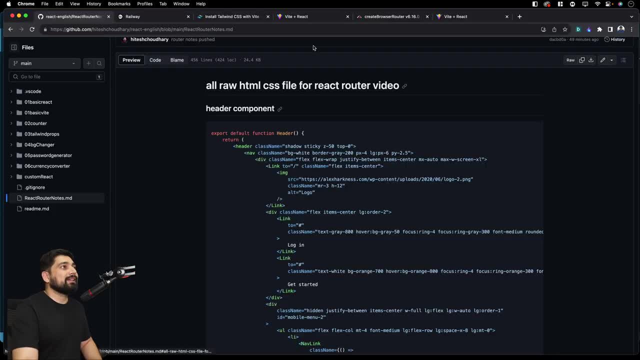 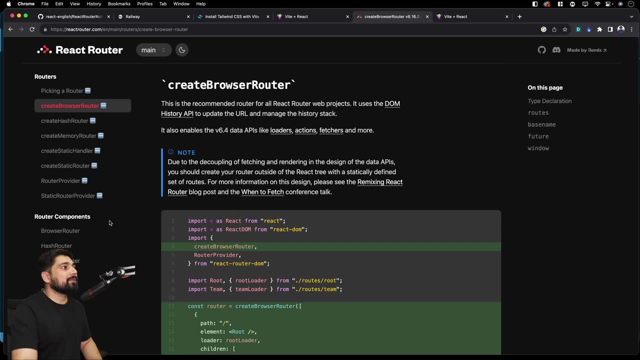 Remember, link is not the only way of navigating. We have the nav link as well, And we can read about the documentation of this one. if they have any global search- I don't think so- Let's just say components. You can see the nav link here. 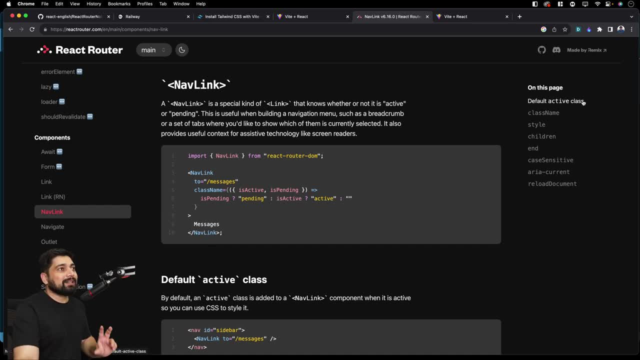 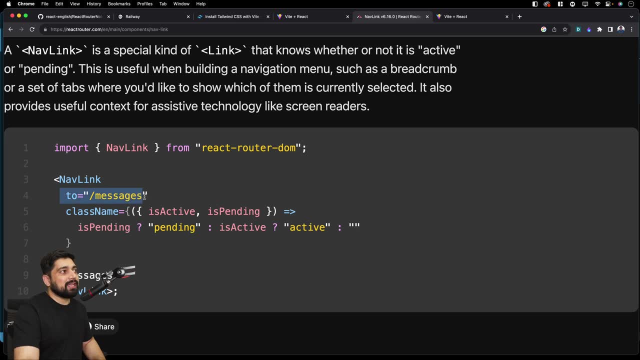 And what you'll see in the nav link. you can find out pretty easily what class is active and what ends and all of that. So notice here it says to messages: so the link and nav link almost same, the two section and everything is almost same. 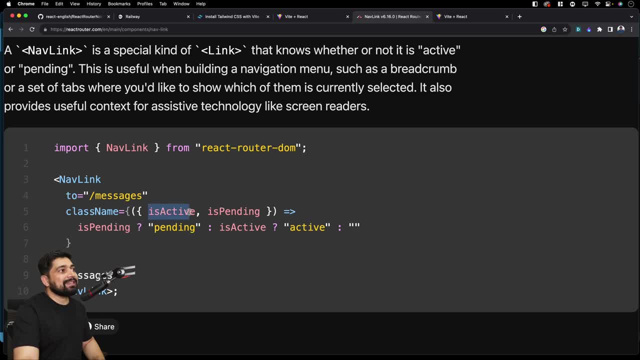 The only thing additional with the nav link is you actually get this is active and is pending and all of that. So why are using this is active, which, whenever you use any class name or any arrow functions like this, it is available to you directly? 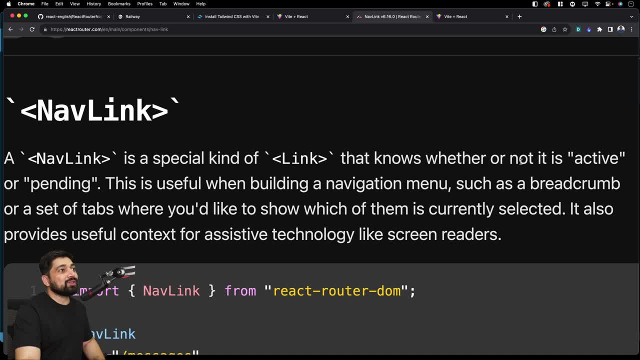 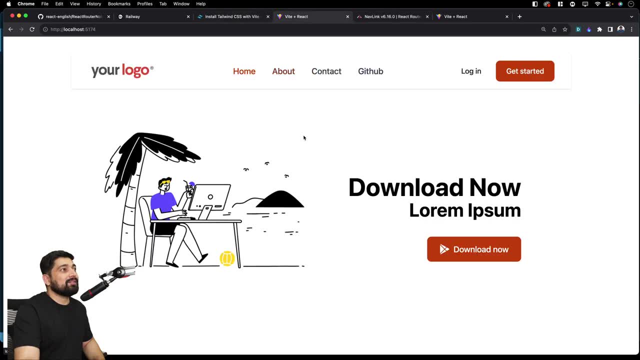 And notice here they also say this: a nav link is a special kind of link that knows whether it is active or not. So when you go up onto the applications like this and when you say that, hey, this page is active, 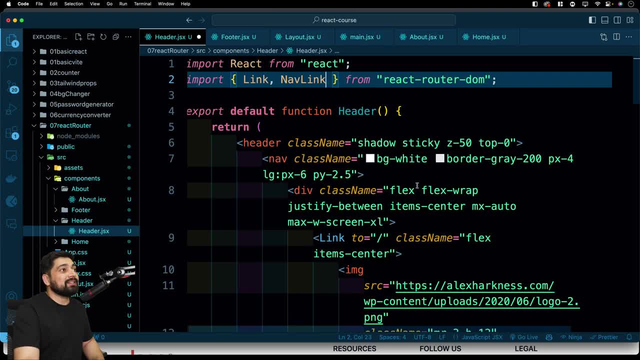 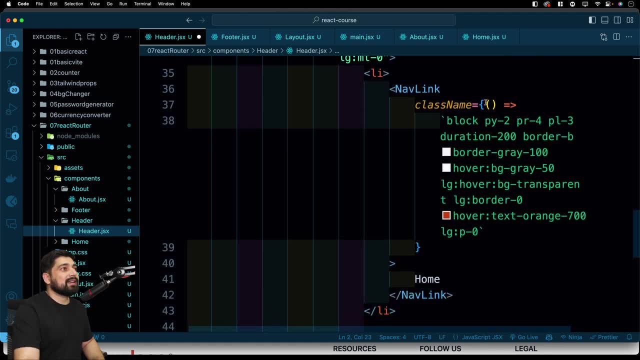 or this page is active, just like that. that whole functionality can be done via the nav link, So that's why we have this nav link, All right, by the way, notice here: this is exactly what we are doing, whatever the values are active, and all of that. 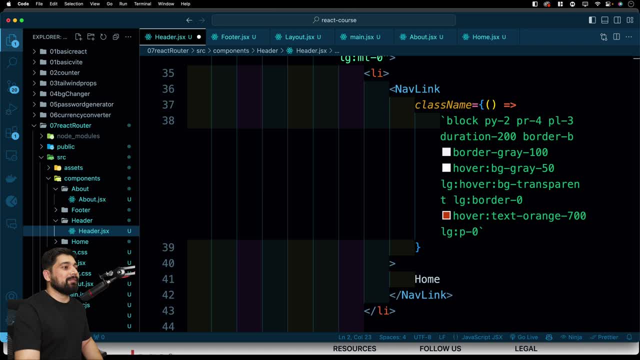 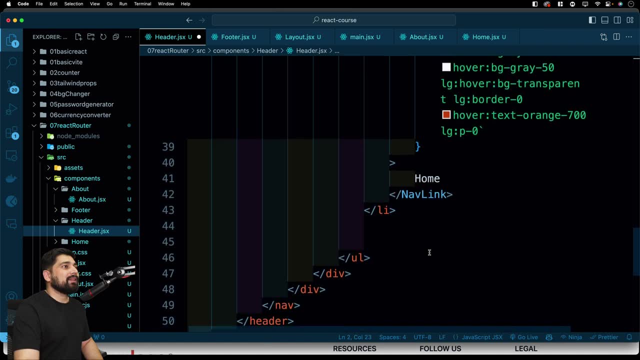 We'll talk about that later on in the some sections where we'll be having. In fact, we can actually talk about this into about whatnot. So this is get started. Then we have a couple of nav links on the home. Actually, we have just one on the home. 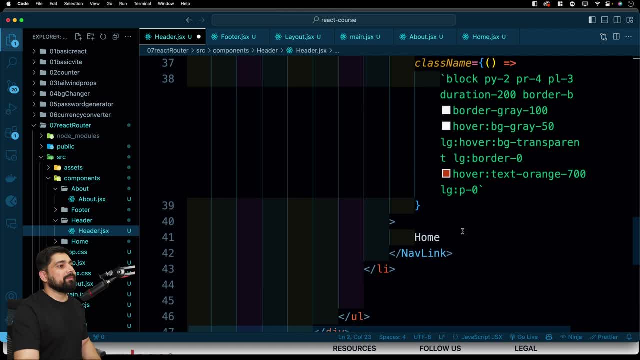 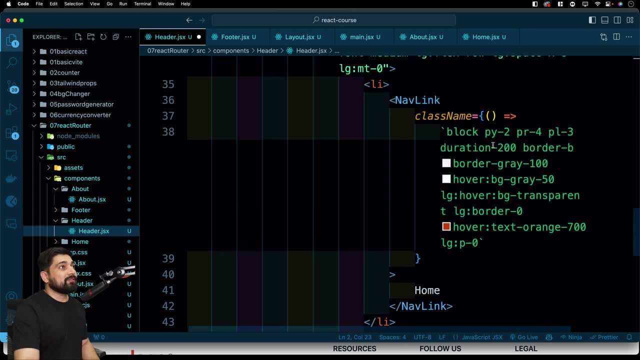 We can design it right now itself. So let's just say on the home, what you can do is you can just add a couple of more practices and what the text you want. So, for example, now we are in the nav link in the class name itself, since we are using a callback. 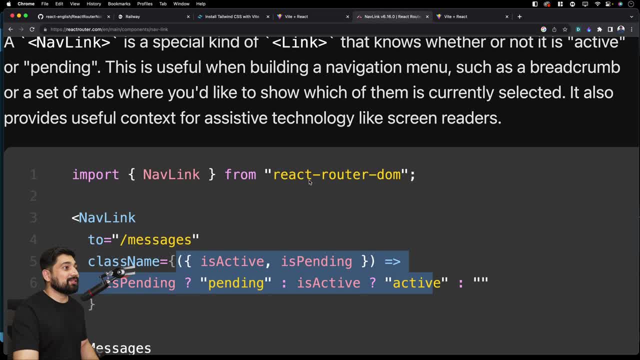 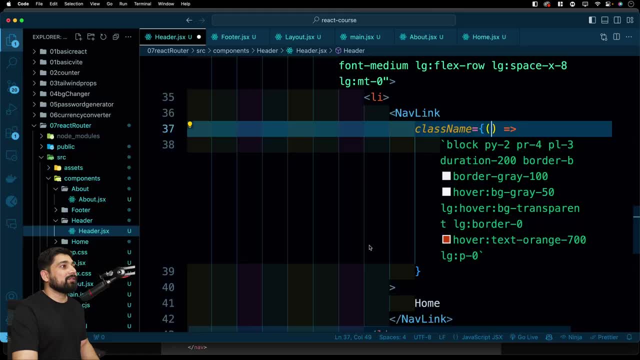 this is the syntax exactly. they are also mentioning it, So we are not doing anything special In the class name property. we have the access of this callback and then we can write all this. So this is exactly what we'll be also doing. 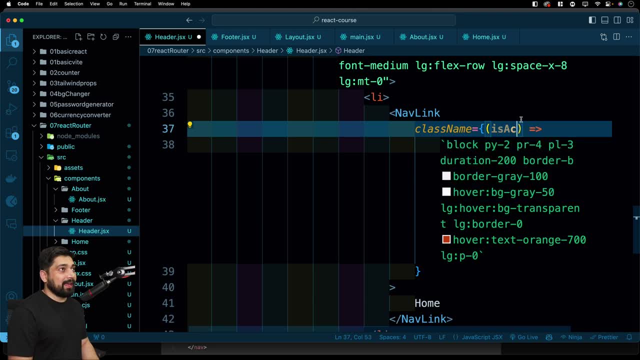 So in this one we have the access. to this is active. Remember, this needs to be exactly as is active or is pending, So we don't decide the variable name in here. So we have this is active. And, by the way, one more thing which usually I also forget: 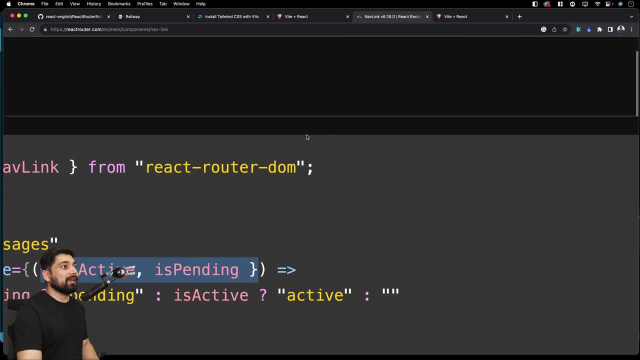 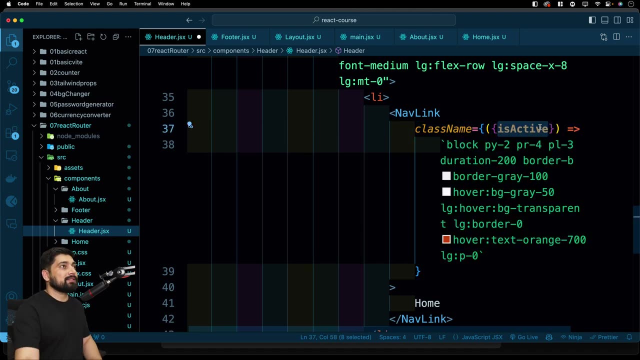 this is active needs to be extracted as a property, like this. So yeah, I also make sometimes this mistake, So let's go ahead and keep it up like this. And now you have access to is active. Now, based on is active, we can decide whether the color is going to be gray. 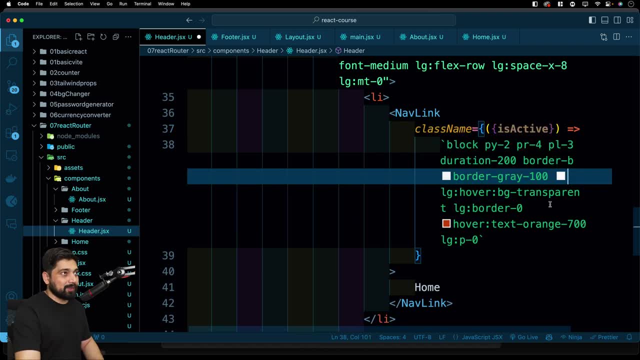 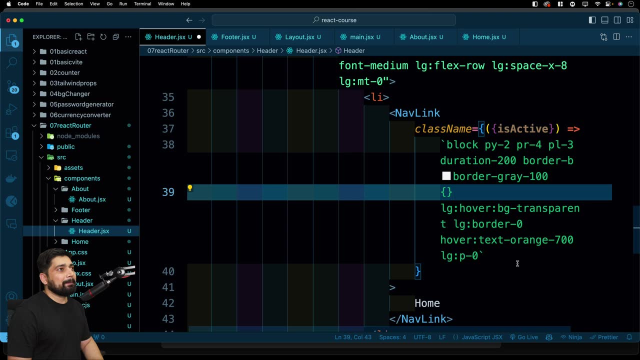 or this one. So we'll just actually cut this out. We want to cut this one out, And once we are cutting this out, we can inject the JavaScript again. And, by the way, dollar sign is missing. Yeah, now we are happy. 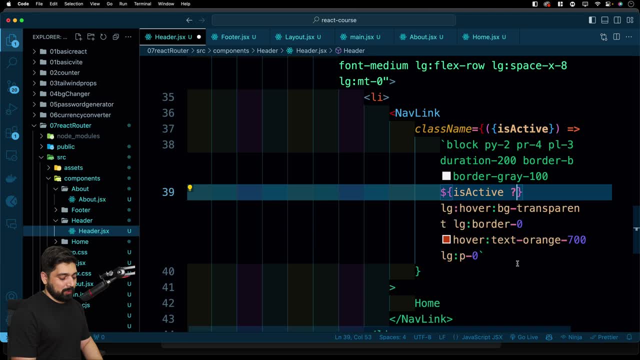 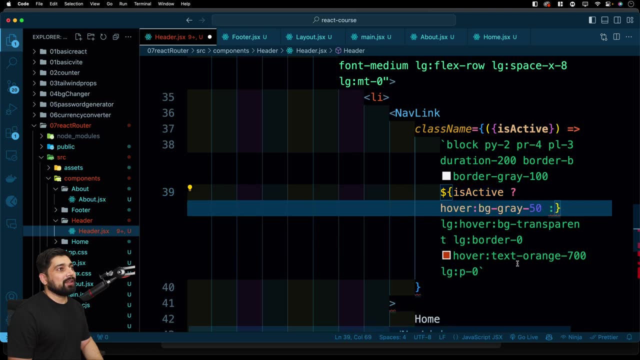 Okay, now, based on, is active, we can do a question mark and a ternary operator here. If it is active, then we can go ahead and use a text of, not this one, text orange. So we'll just say text Dash orange. 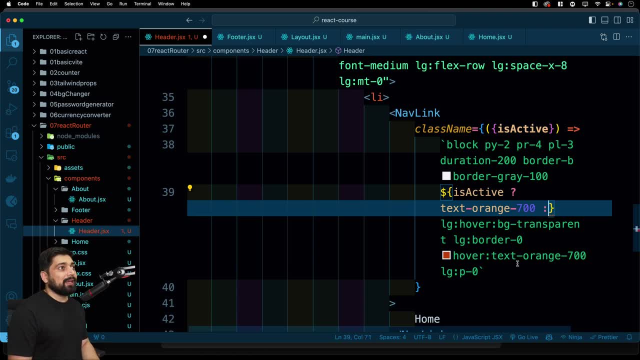 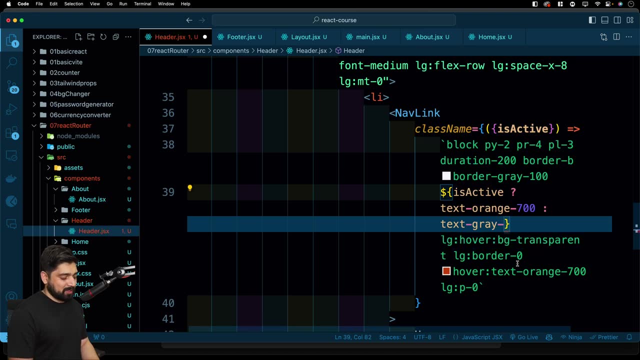 We'll be probably using 700 version of it. That's what we used, And here we can use a text dash: gray 700.. Gray 700, no suggestions. There we go, No suggestions. strange, Anyways, we can just find it out later on. 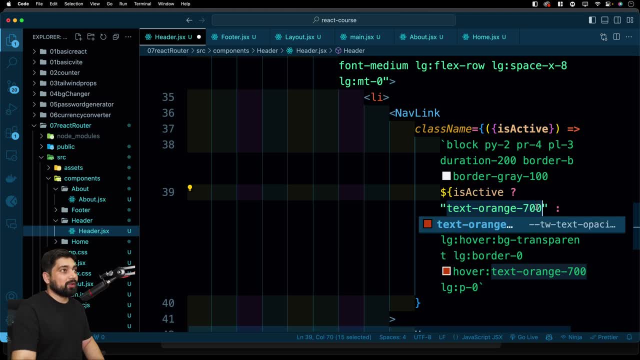 if we are doing any mistake And, by the way, this needs to be wrapped inside the quotes because it's a class, not a variable Class. I mean to say tailwind class. So that is all what we have And, based on this, we can have a nav link. 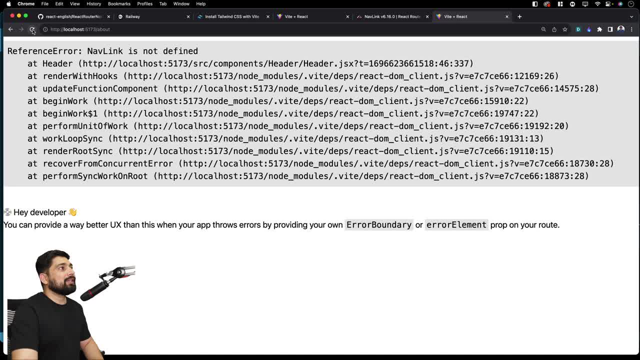 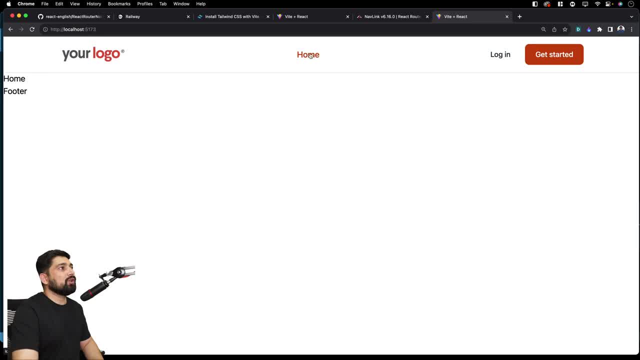 which can provide you, whether you are active or not, onto this one. So nav link should be defined. So now we are on home. But if I go onto about, so we have the home And if I go onto slash about, this should be technically going away. 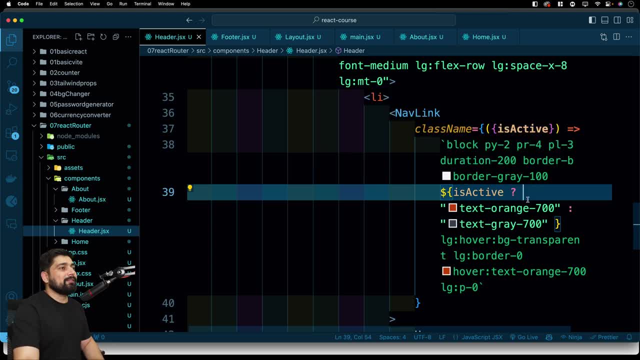 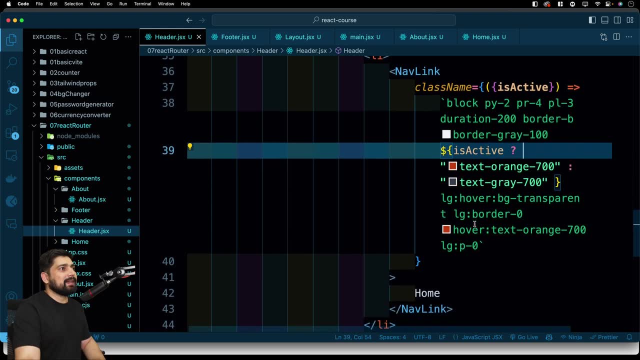 We shouldn't be having this link, as if it is true, then it's 700.. If it is false, it goes like this: border gray. We'll see that, how this actually works and how we can actually have more links onto this one. 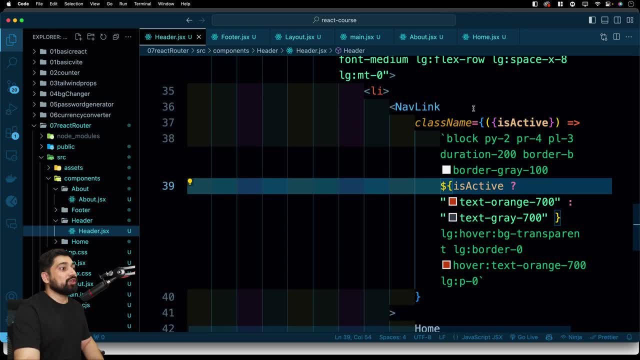 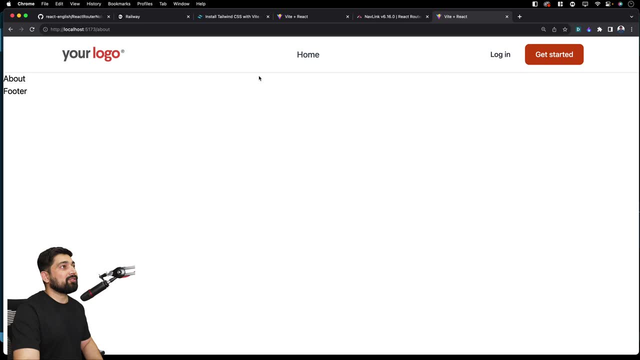 This one is nav link. We haven't mentioned the two. We have to mention that, otherwise how it will work And we'll be saying that, hey, you will be on slash, So now it will keep a track of there we go. 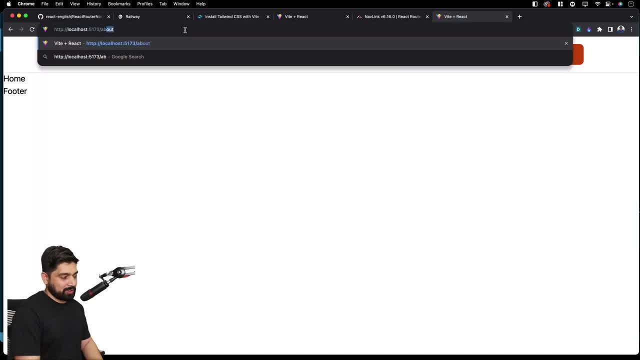 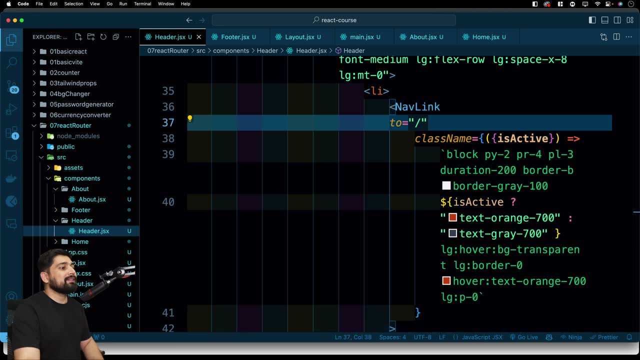 Now, if I go back to home, it's orange, But if I go back to slash about, we are not active, There we go. Told you Simple. Okay, now we can have multiple of these allies and can define a home about whatever you wish. 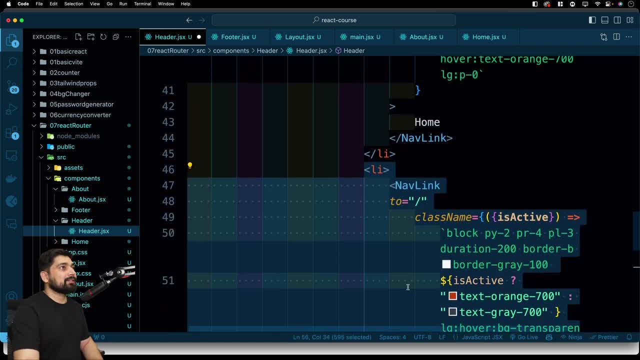 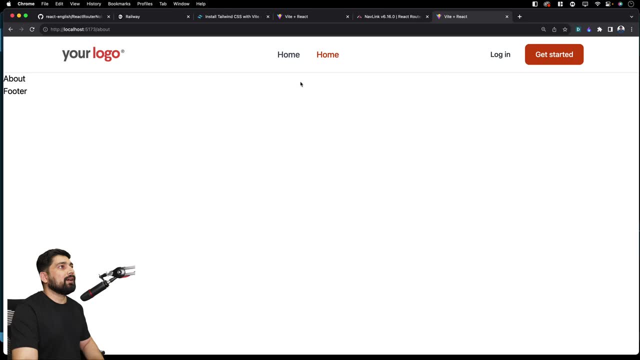 So I'll just copy and paste from ally. I'll just duplicate this, And this one is going to be slash about. And there we go Now I forgot to change the text About: save that Now we can travel to home. 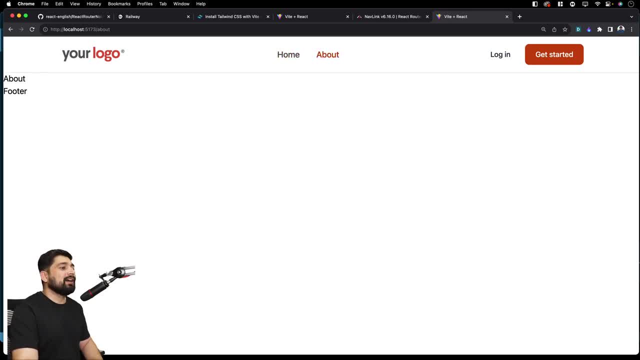 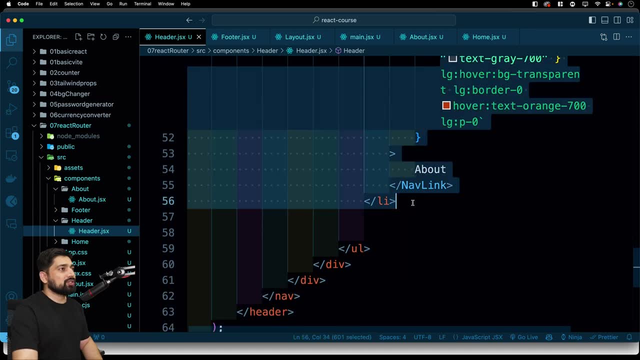 We can travel to about And similarly we can have more of these. So, if I remember, we have home about and we will also have the content Contact, So I'll just duplicate this one. I hope you remember the shortcut for duplicating in VS Code. 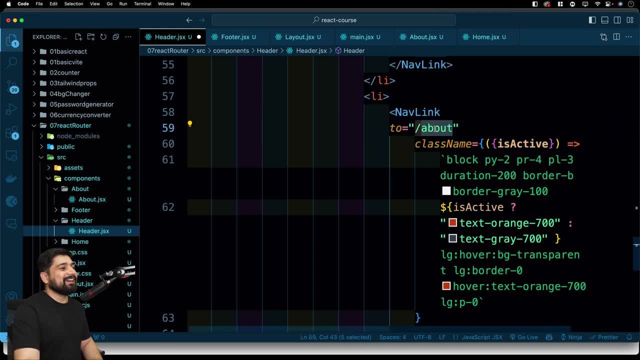 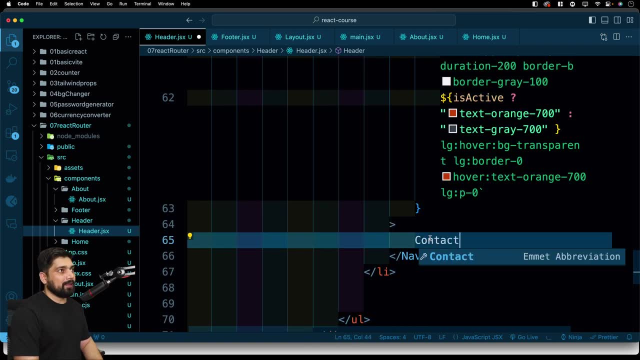 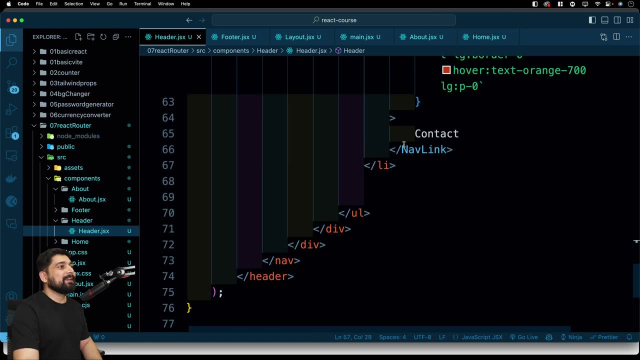 If not right now is a good time to find it out about. Okay, home contact Contact. This one is going to be contact. We also will have probably GitHub as well. We'll be having some fun with GitHub as well. 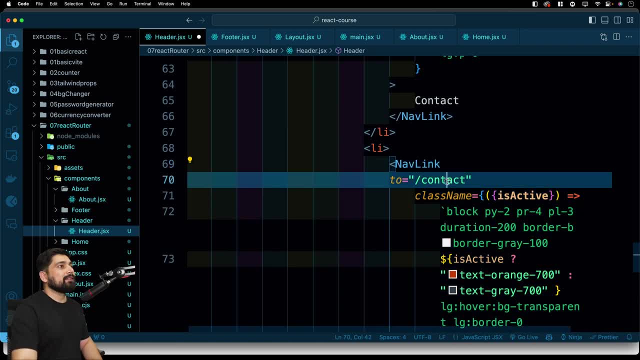 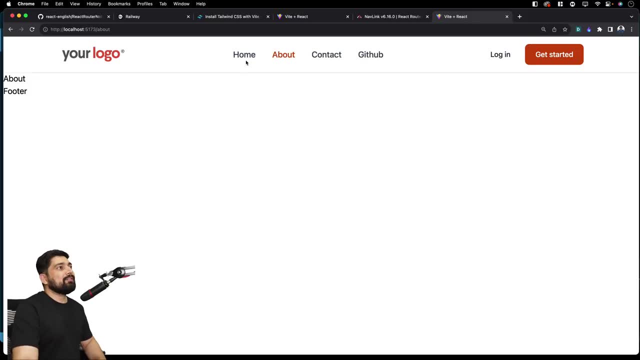 All right, copy and paste that. This one will say: I'll go to GitHub component wherever. that is All right. So now we have home, We have about, Although there is nothing inside the contact, So this route doesn't is there. 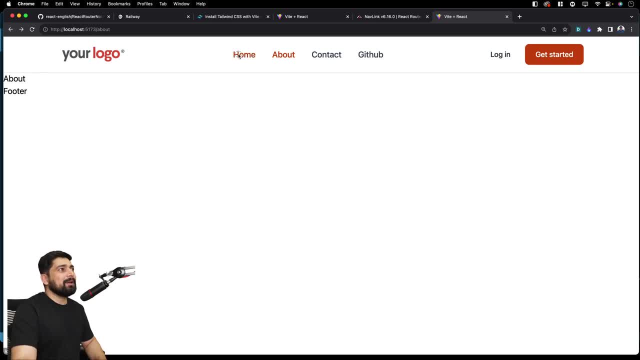 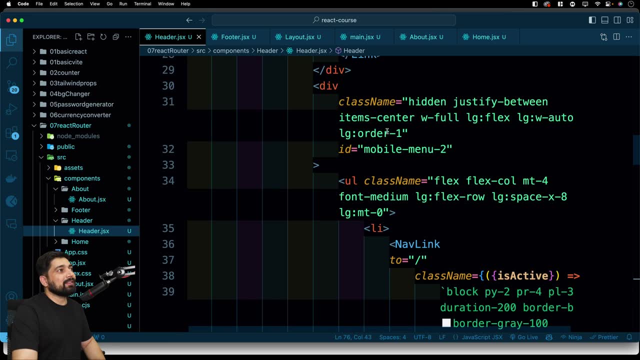 So we need to actually define our 404 route as well. We can work on with that, But at least our home and about component are there And we now know about the nav link, which is a special kind of a link, And we are aware of how things are there. 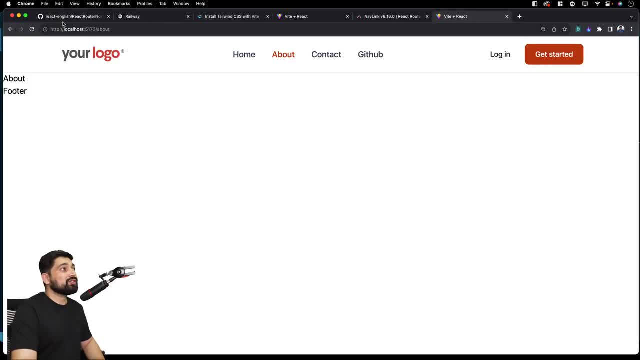 Now, with this, we can actually go ahead and move on and work with the footer, which is super easy. Now you can go onto my notes, and this is the footer. Just scroll it on the all the way to the right And you'll find this copy button. 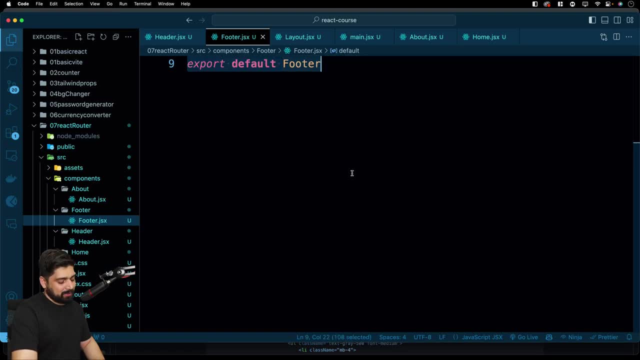 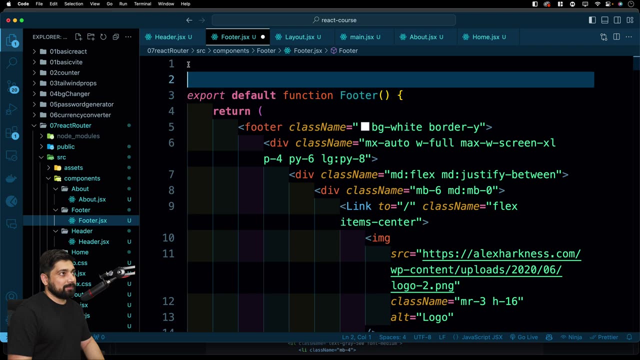 or you can manually copy and paste that, And all we have to do is paste this all here, Since we have link in this one. So just go ahead and fix the errors. Let's first import the React, Import React, and then we'll be importing the link. 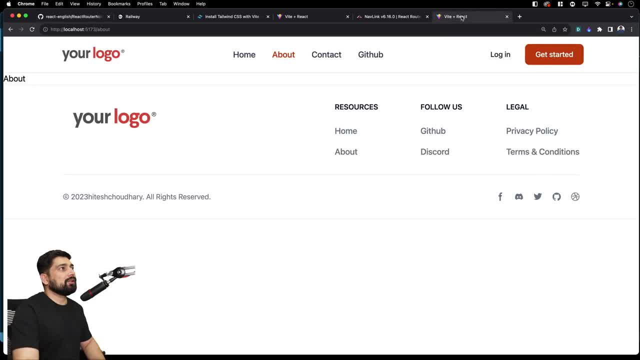 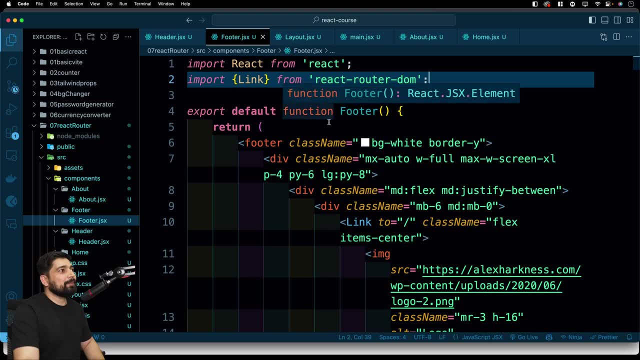 And that link is from React router DOM. Technically we should be all good now So we can see at least a home and about, but our footer is coming, So it's looking nice as well. Apart from this, there is no big deal and no facade about it. 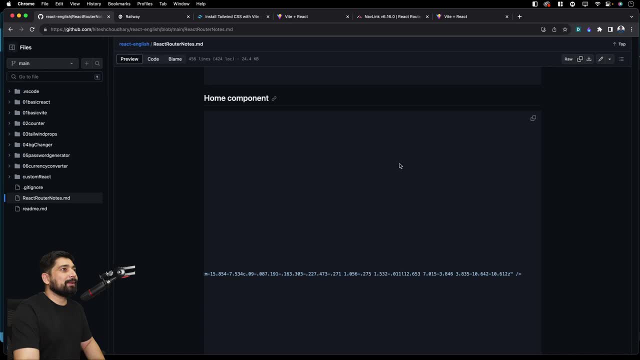 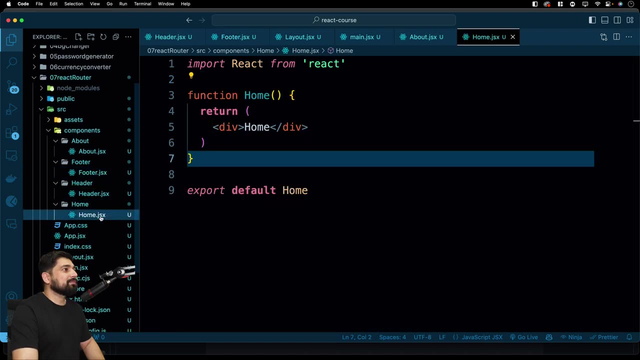 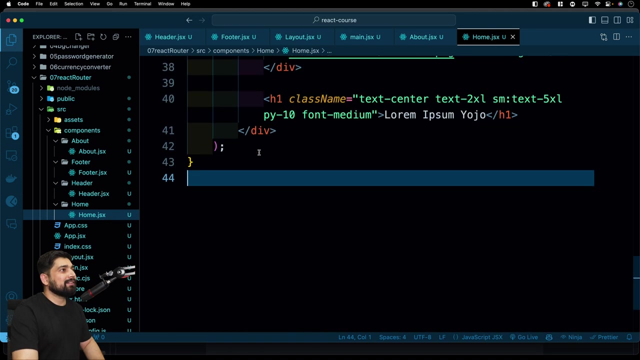 Similarly, we have a home component as well. We can go back and replace it with the home. So again it will look just a little bit beautiful, nothing more than that, And home select all replace it. I don't think so we have anything in this required. 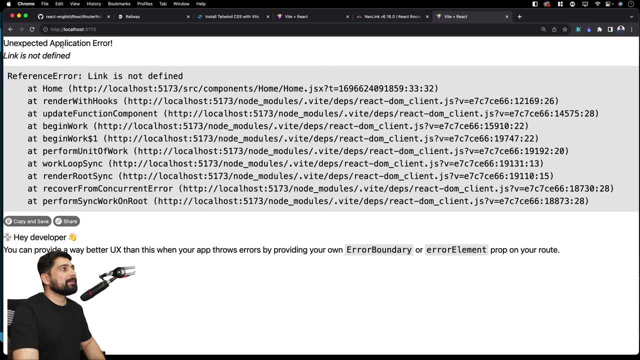 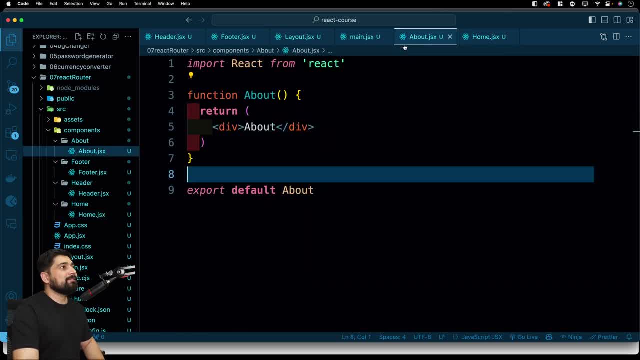 Let's just try this, Save this and go back And do we have some links? Yep, we have some links in the home as well, So let's import that. no big deal. In fact, we can actually copy paste footer. 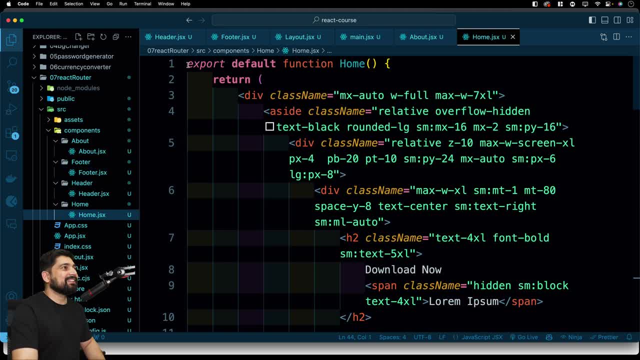 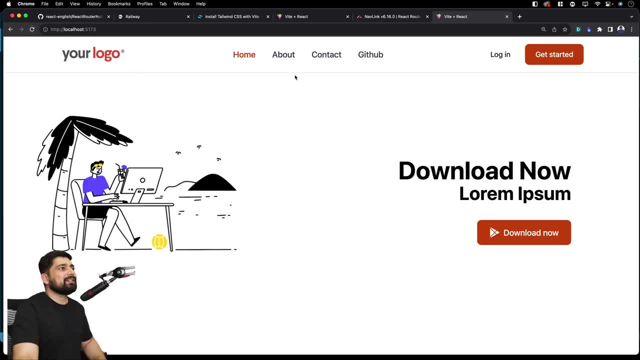 Yeah, and let's just copy and paste. All right, let's come here And there we go, should be all okay. now, There we go. so we have home page. So we have learned how we can design that home about and what not. 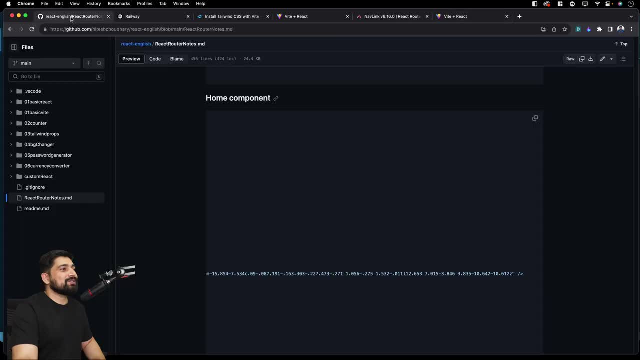 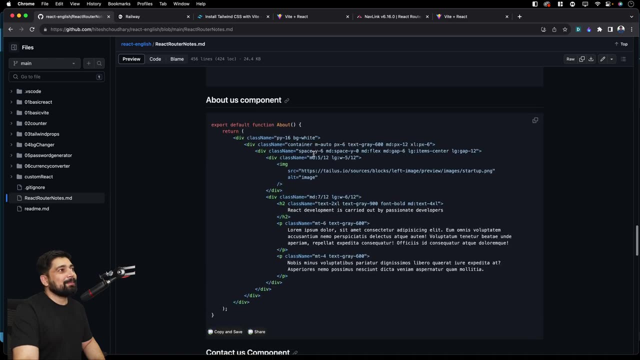 So I'm leaving this contact page to you as a simple exercise. All you have to do is go up here- Now we have the contact us page as well- And go ahead and work on with the contact us page about, us page About. I can do this fun for you. 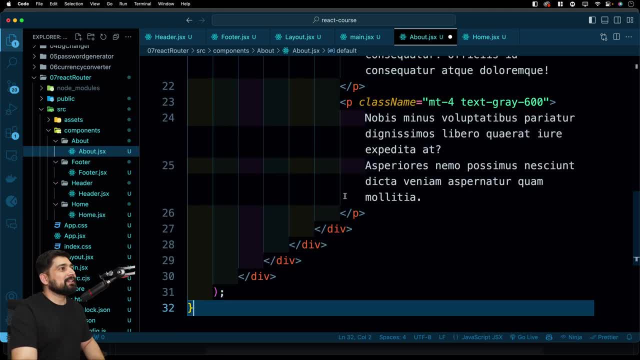 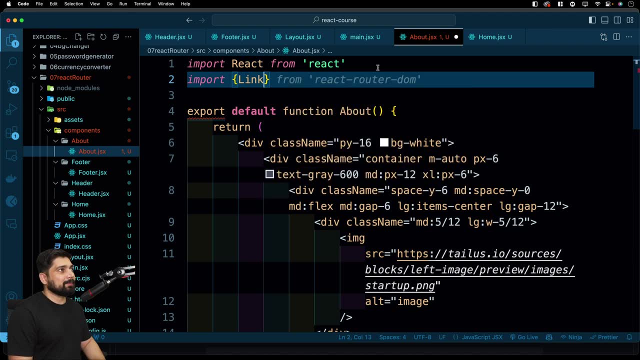 Okay, so about is here. We'll be replacing it with here and we'll be importing the link if we have. I don't think so. we have link from react router down. Let's see if we have about. yep, home is looking good, about is looking good. 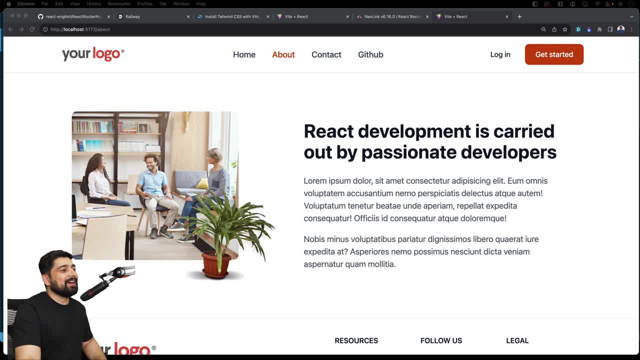 Contact is for your exercise. maybe, maybe, I don't know, We'll try to have some of the work. We'll try to have some of the work with the contact and user and what not. Okay, one more thing that we'll be doing is we'll be creating another component. 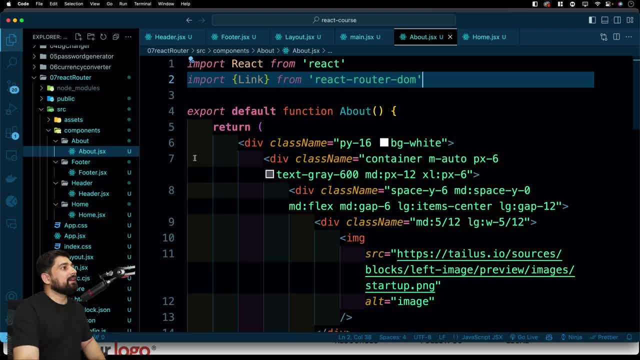 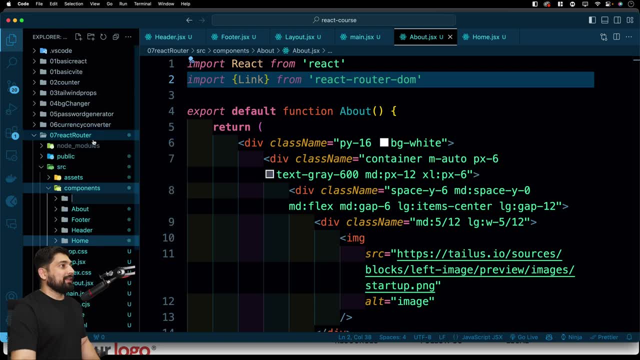 Let's go back onto the code side of it And we'll be creating another component. Let's call this one as user, because I want to show you some more ideas that you'll be using. Let's call this one as simple user. 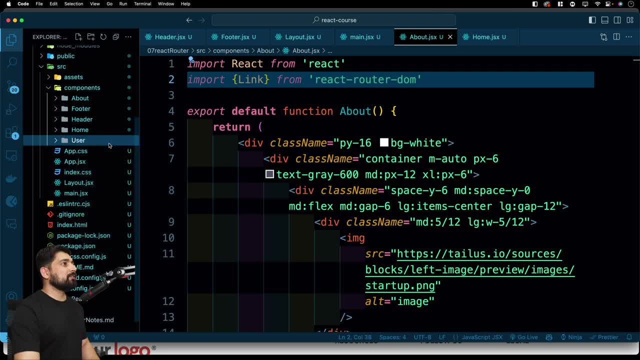 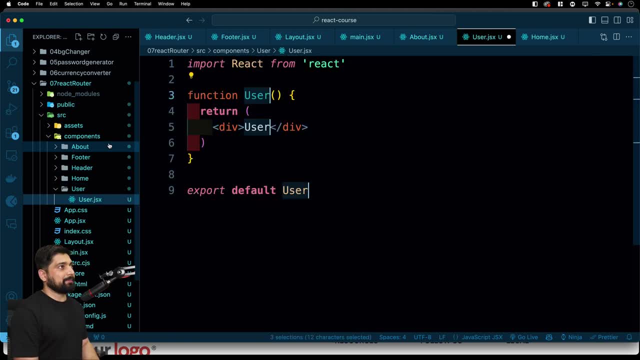 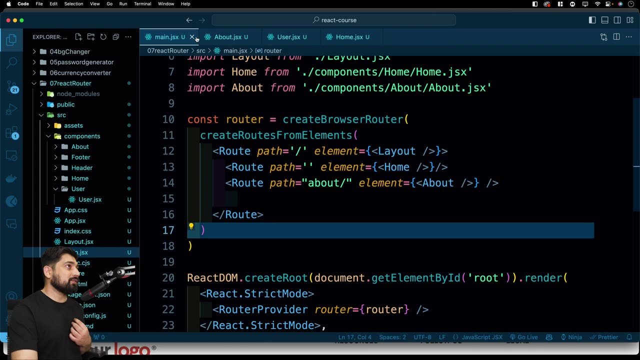 And we'll be having a simple layout here. new file That will be userjsx And just the basic RFC. So we have a user Now in order to make sure that this component loads somewhere. we have too many files opened up. I would love to close that. 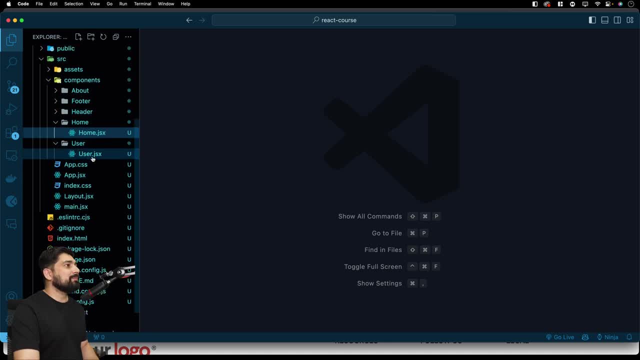 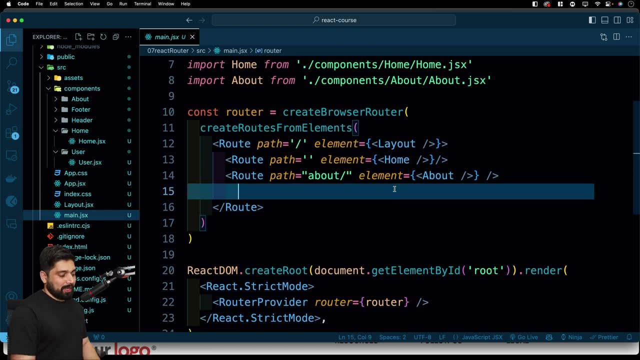 In order to make sure that I have a really huge code base into the user. in order to load this, I need to go into mainjsx, And how can I load a route which actually loads this one? So I can just go ahead and say that, hey, I want to have a route. 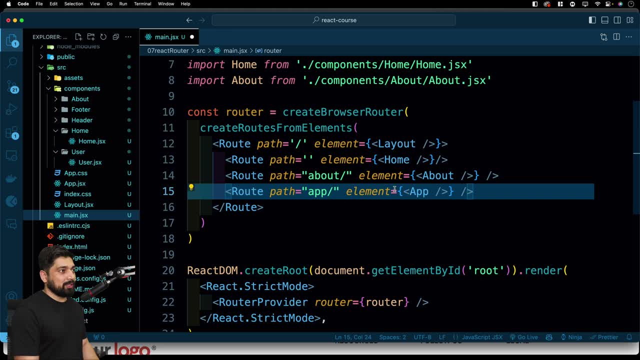 And this route will be ongoing to whatever the path you ask me to do. So I'll just say hey, go on to user, And the component or the element that I'll be loading here is going to be a user. User. it doesn't suggest me user. 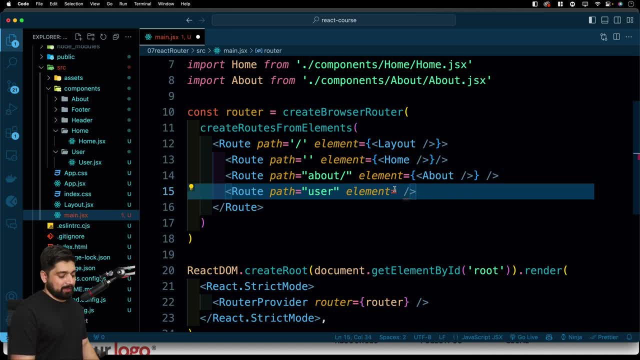 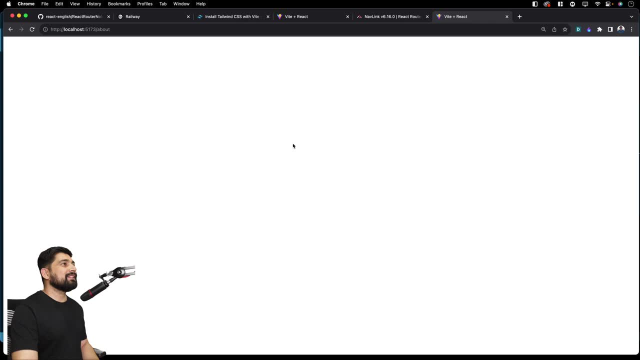 Okay, I'll write that again. I want suggestions. Okay, there we go And here we'll be saying: hey, give me user, It doesn't give me user, Save that. and probably this will give us issues, It surely will. 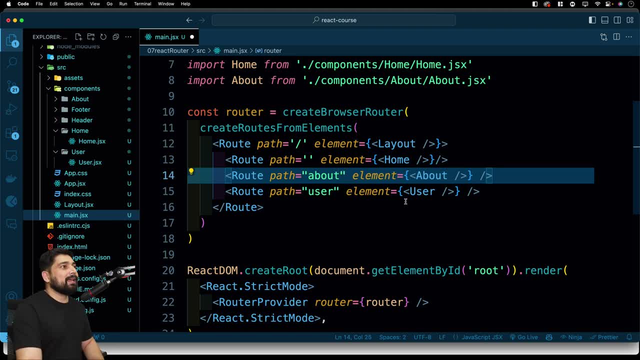 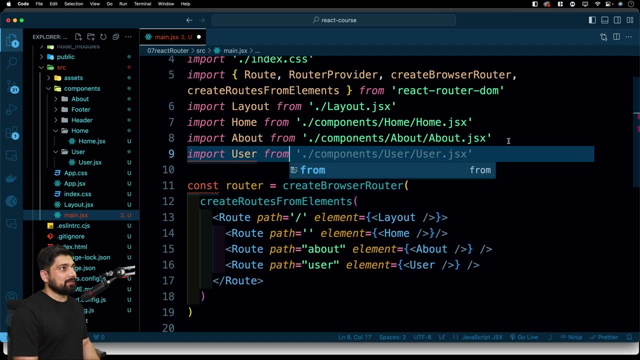 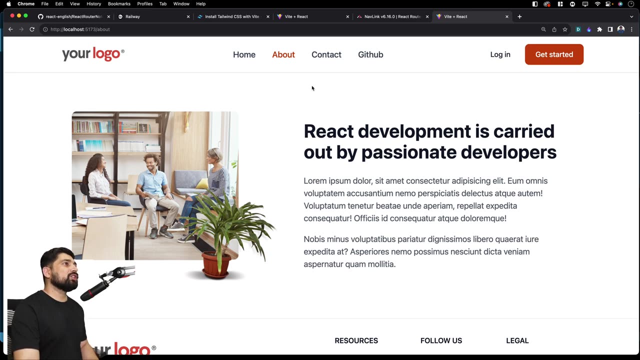 I will just first remove this about, because we don't want that. The element should be user, It should be auto-importing that And we'll be saying: import user from component user userjsx. Okay, all happy. Now can we have another link for the user itself? 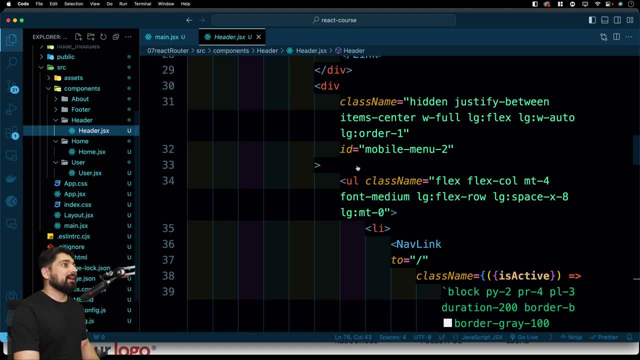 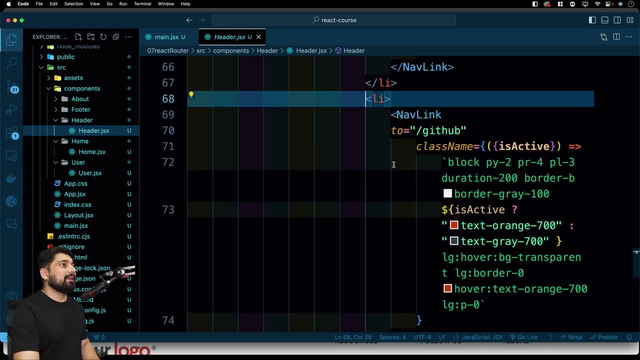 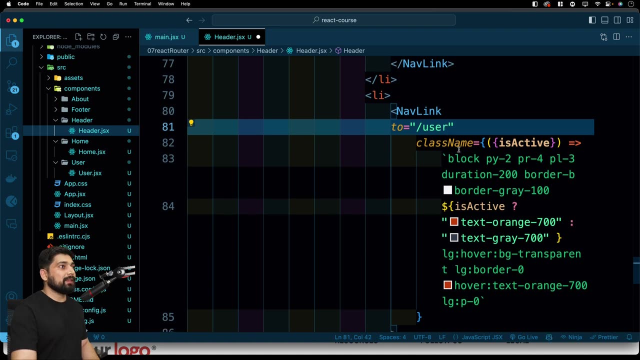 Probably yes. Let's go into the header Header. and can we have another li for the user itself? Let's try this. I think go ahead, copy and duplicate that. This will be going to user and we'll be calling this one as user. 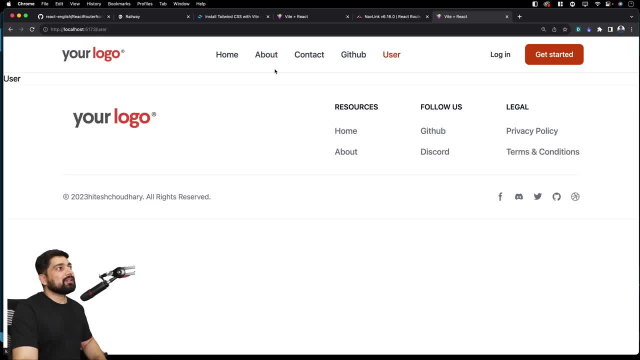 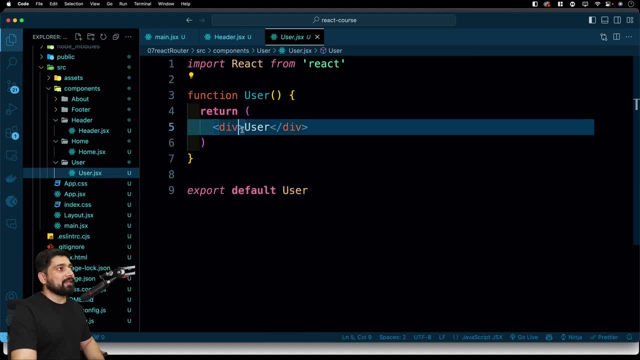 How easy that was. Okay. now, if I go back to the user, okay, I get the user Now in this user. first of all, let's just central line some of the stuff. We don't want it like that, So we'll be adding some of the class name. 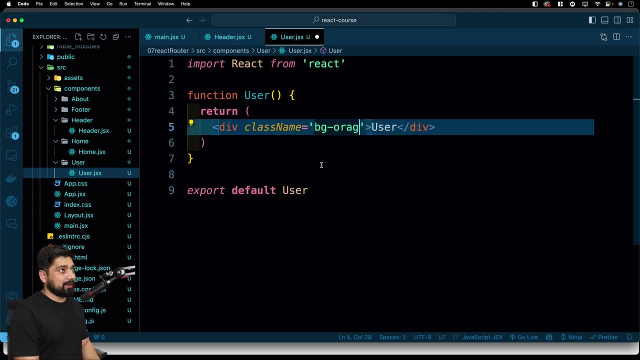 We'll be adding some of the background bg-orange suggestions. We'll be using orange like this And we'll be saying: text dash black and text dash three x three, xl. text dash three. come on suggestions. three x no suggestions. 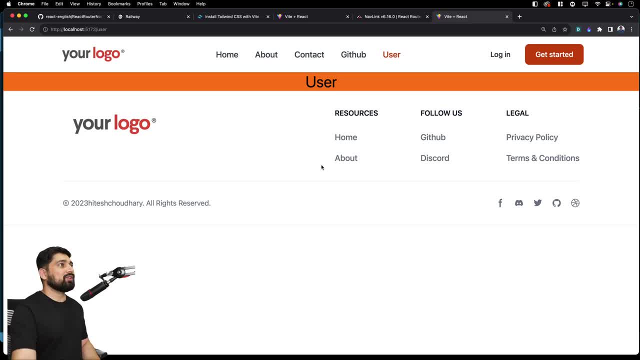 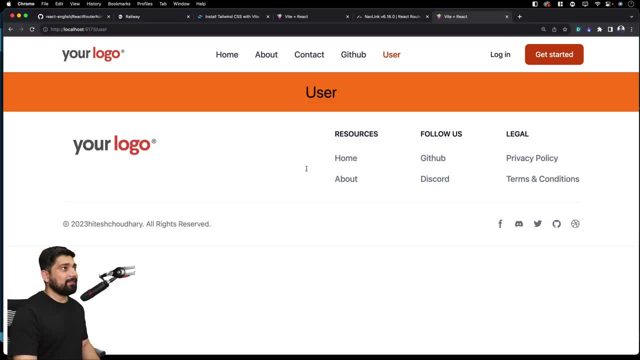 Yeah, text three, xl, And we'll be saying text center, just to make sure things are all good and okay, at least they are visible. We can even add a padding on y-axis of five. Yeah, better, Okay, so so far we are all good. 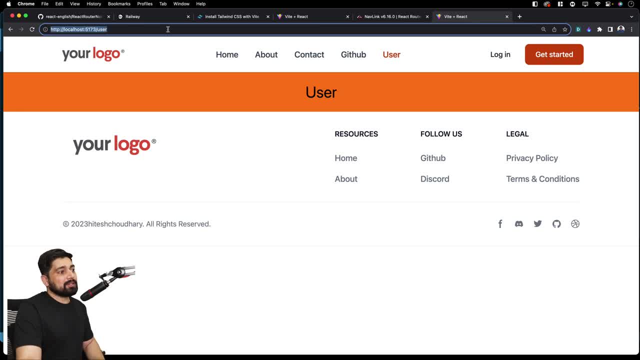 and we understand this part is there. but there will be cases in your situation where the user will be dynamic. So dynamic routing is a very common scenario. So, for example, the user ID is: why cannot I write it here Something like 123, or maybe username? 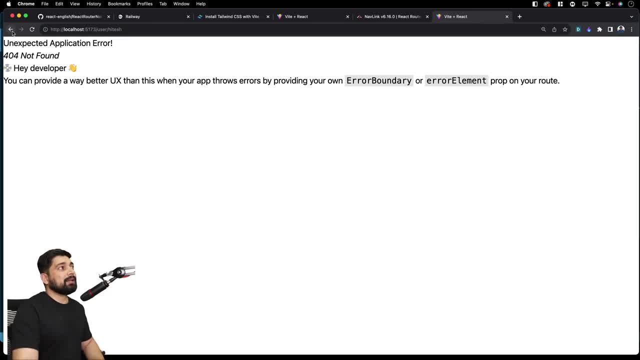 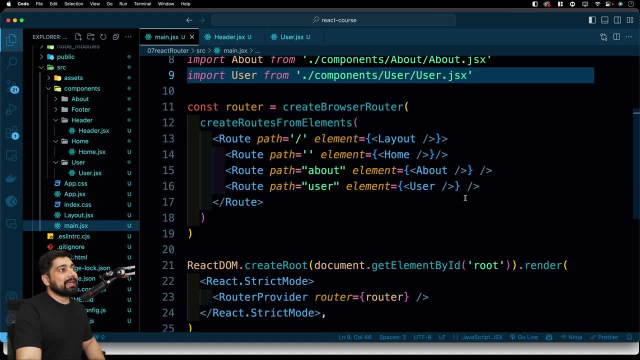 with a username of Hitesh. So I want to grab this path and this URL So that dynamic capturing is one of the core essence of how you will be using the route. The way how we use it is actually simply go ahead and simply write something here which is slash, and then 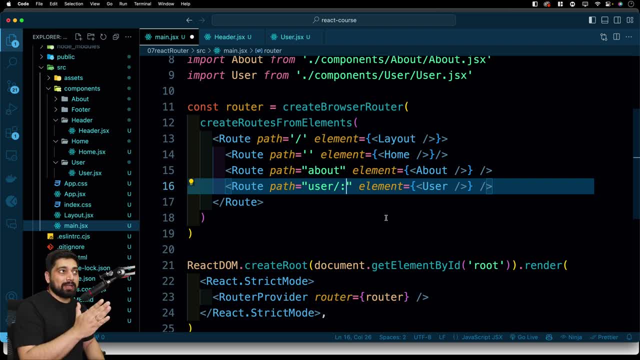 the colon is important. This is how you capture anything after the user slash Whatever comes next to it. you'll be able to capture that And then carefully name this parameter. This is a placeholder user ID. This could be just ID. this could be product ID. 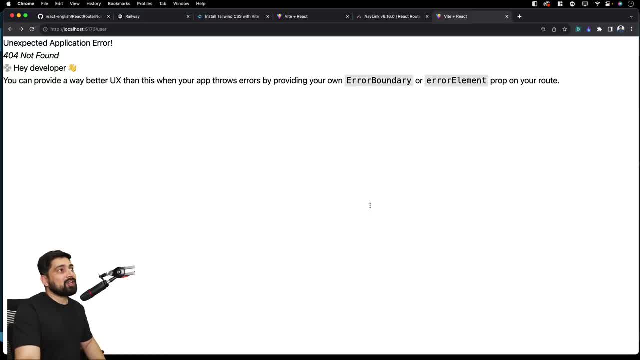 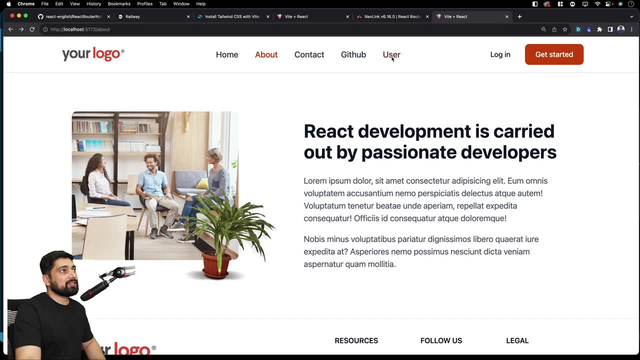 whatever you want. this could be anything like that. But this is not job done, because if you go back up here user, definitely that's all good. But if I go back, so notice here the user. now we are saying, hey, this is not happening. 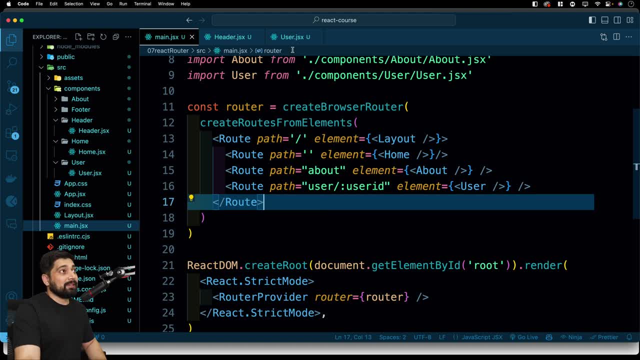 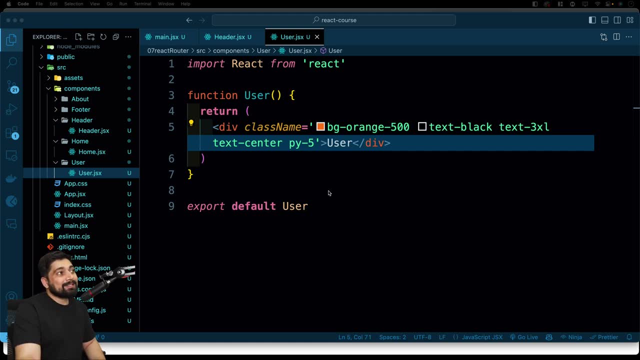 Because I don't know what to do with this. This obviously will give us error. Now we need to go into the user and figure out a way that we accept all these things Now, in order to make sure that we have defined that this path is actually accepting the parameters. 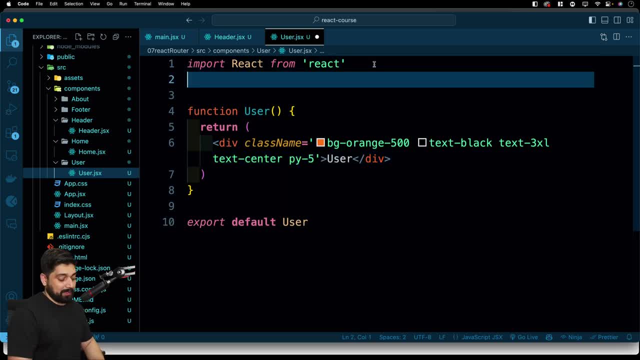 and what not. we have to use the params And, yes, this is literally the name And we call this one as: use params, no suggestions. Use params, no, no suggestions. Yeah, that's bad And that actually comes from. 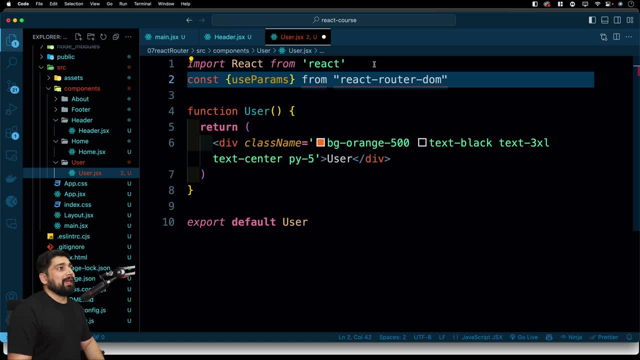 from react router DOM. Okay, and why are you having issues? Because I wrote const import. There we go. Now all you have to do in this case is this: use param is actually a hook. We studied hook quite a lot. 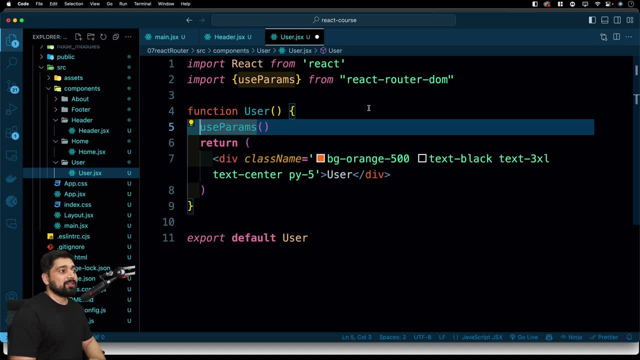 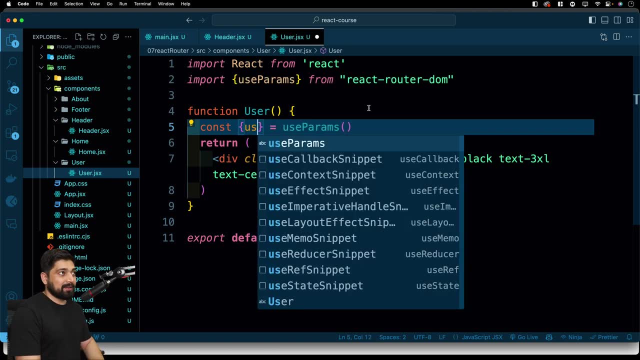 And this is a hook. that means it's a function, nothing more than that. But what this function gives us back, that is important for us. So it gives us a lot of things. We can extract some information out of it. What information to extract? 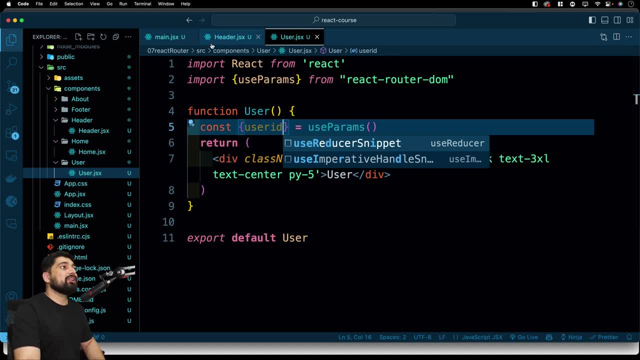 Yes, exactly, user ID. Why user ID? Because we call this as a user ID in this place And after the colon, the colon is a symbol that hey, this will be going into use, param, And you'll be able to extract this. 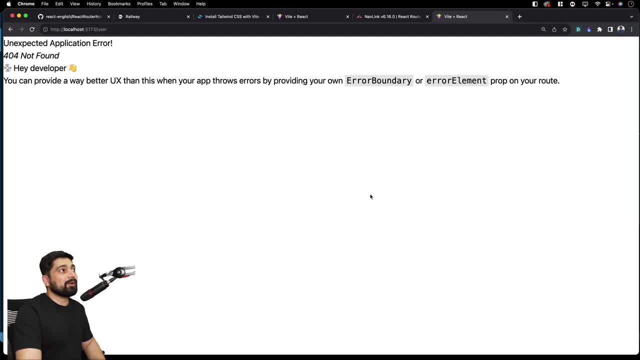 with a key ID of user ID, just right here. Now let's just go back. what happens if I go ahead and get back? It says: hey, prop on route error boundary. Okay, looks like this one is okay, but my mainjsx is having some issues. 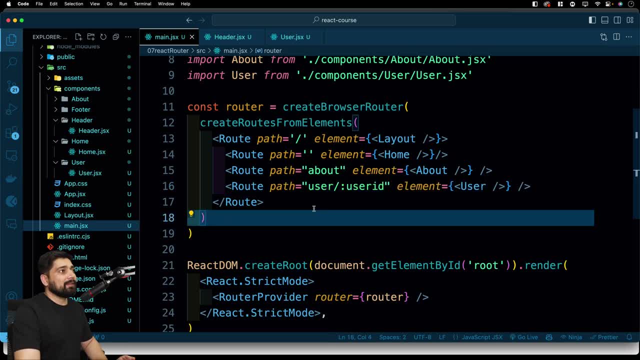 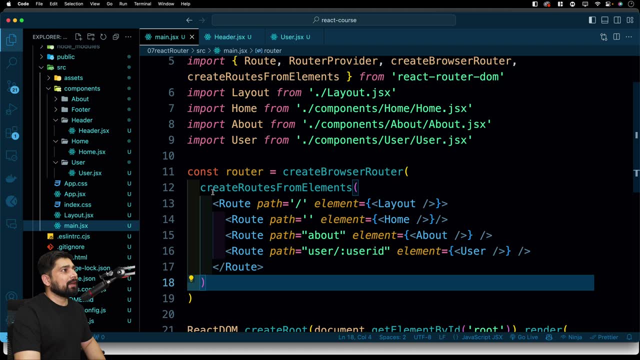 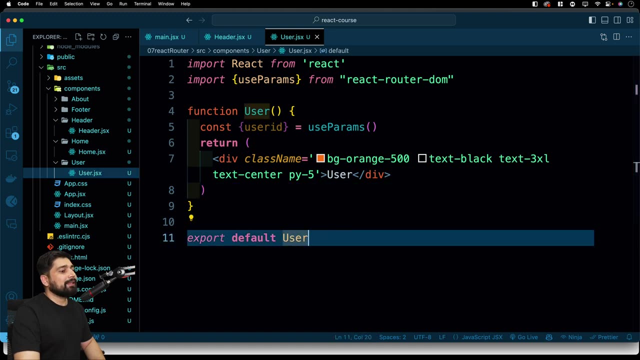 Let's go back onto mainjsx. This one user path element is all okay, Should be all okay. And let's also check the user. I'll be exporting that. export default user. We are exporting that. Let me quickly check that. why this is yelling at me. 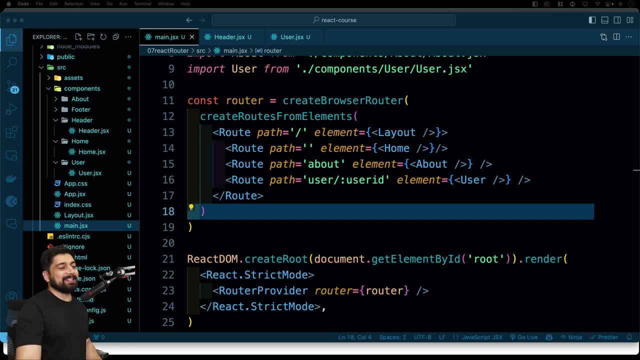 All right, so found the bug a pretty easy one, Probably because it's late night sometimes these things happens. So again, we are actually good in this case. already The issue that we are facing is pretty easy. actually, If I go ahead and refresh this, this page works. 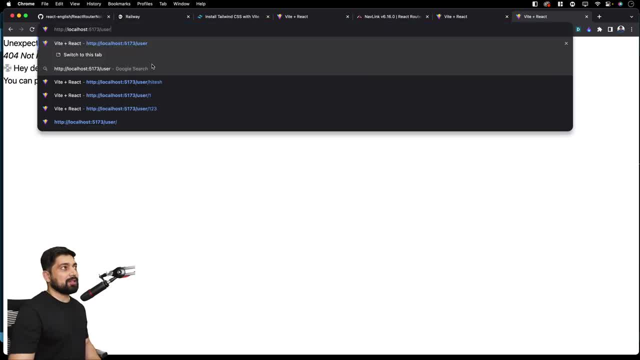 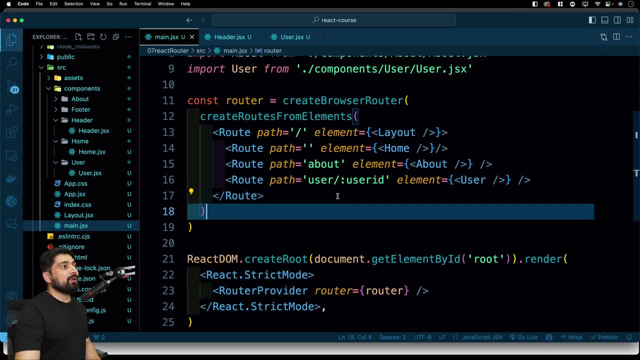 but if I go on to the slash user or this one, this doesn't work because we never defined the route that what happens when the slash user only comes. We are only defining and are talking about what happens when the user slash and some parameters comes into that picture. 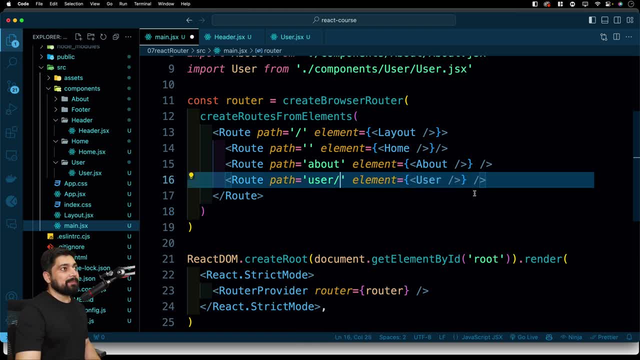 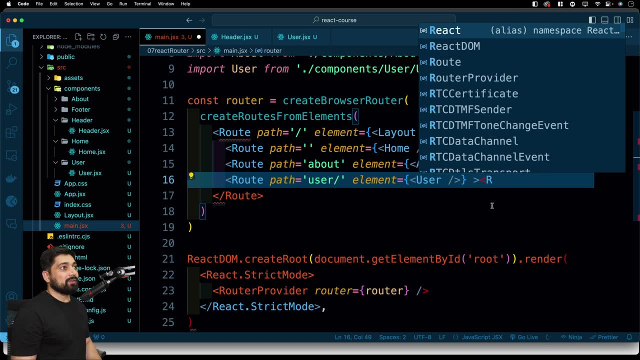 So the easy way to fix it is actually to remove this. Let's cut this out And let's not make this one a self-closing use, the sandwich of concept that we studied about. So we'll be saying that, hey, let's just go ahead. 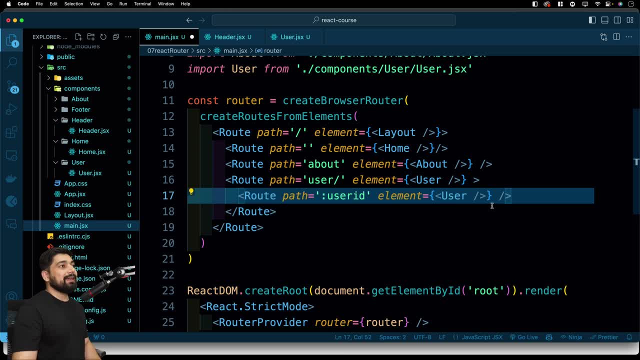 go ahead and close this route. Now we can use the sandwiching concept And then I can use the inside the sandwich route, which obviously will make it as slash. Everything is inside slash. Then we have user On the user. we'll load the element user. 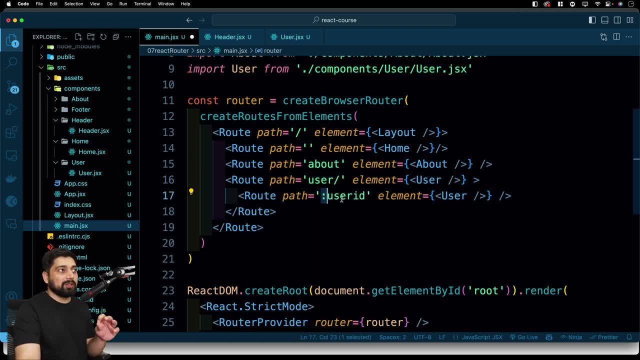 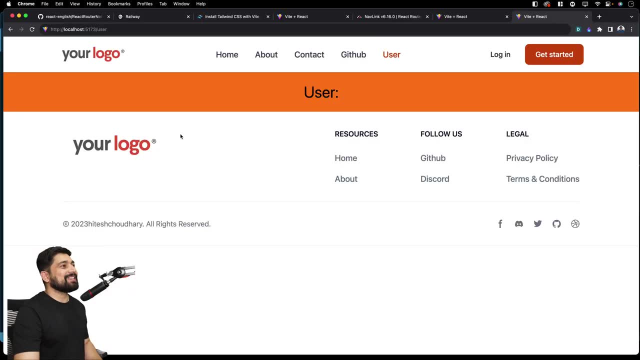 And after that, if there is a colon which technically makes user slash colon user ID, we will load again the user element. So very basic, but again, sometimes these things do take some time to debugging. So there we go, We have this user. 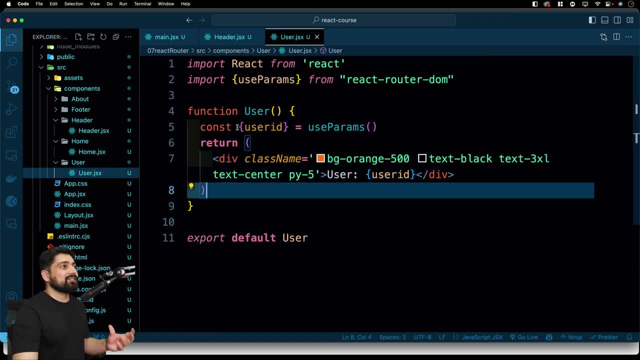 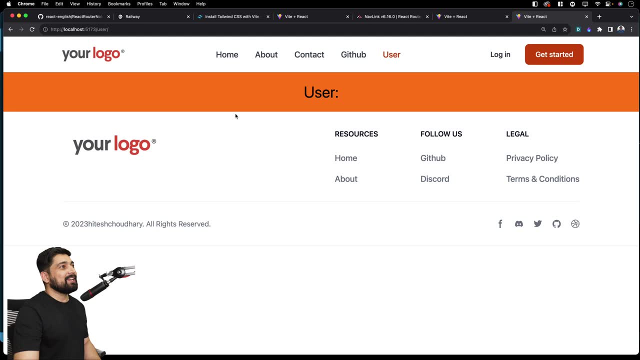 And what? additionally, what we did is inside the user one. we have this user And since we extracted this user ID, I just placed it here. It's just a variable. I'm displaying a variable in JavaScript. I'm not doing any magic here. 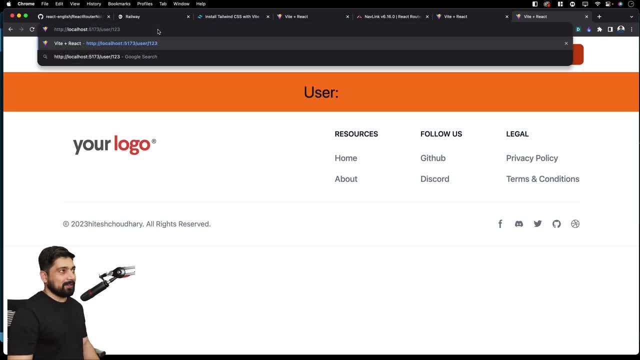 So when I go back here, the advantage of this is now anything that comes up here in the URL after this: whatever the dynamic route, I will be able to catch this dynamic route. For example, if I just have something like Hitesh here. 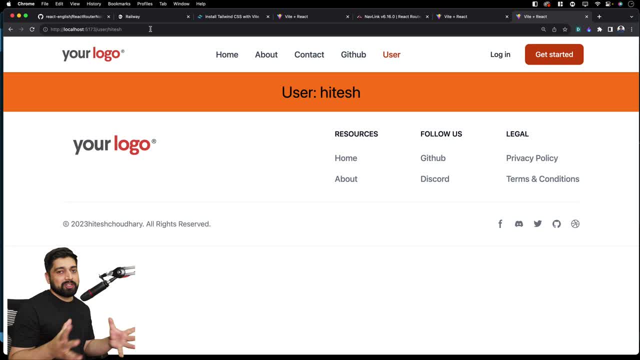 I can grab this. Maybe this is something on the user page where you have some clickable elements. and why clickable elements? you are coming on to some GitHub user ID, some blog or anything, So I can grab elements from the URL itself, make a fetch request and get the data. 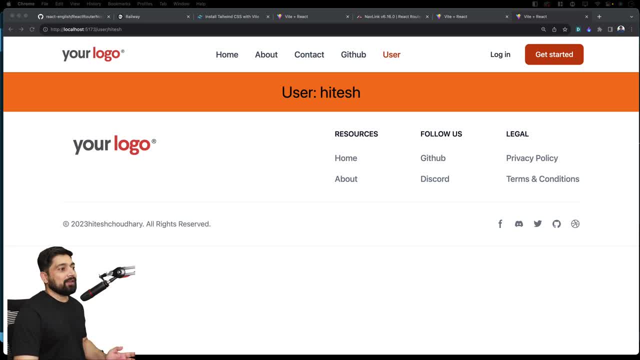 So this is the whole idea of doing everything that we are doing up here. All right, so now let's go ahead and work on with some more stuff, which is also pretty interesting, and a new concept in this one. Actually, Nextjs also uses this same concept. 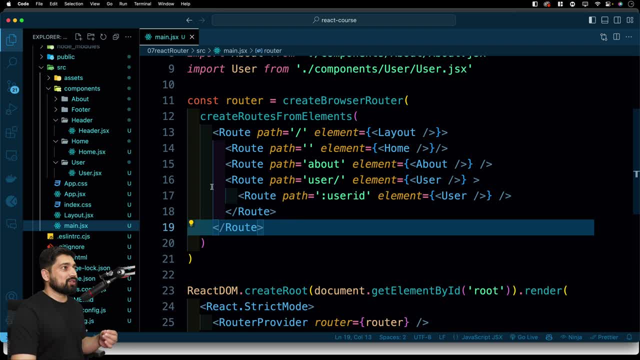 So we'll be working on with this one. I hope the center element of this one, how the routers and the dynamic parameter- comes up. this is all clear to you And, by the way, even if you don't put this one and directly put up this, 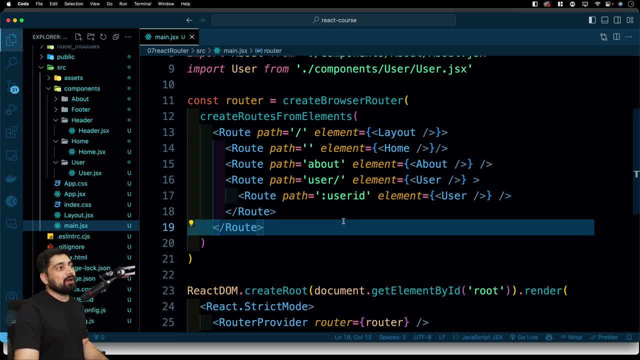 then the user route will not work, but user slash, whatever, something will also work. Okay, going back, we need one more route to work on with this one, So we'll go out of the sandwiching. We are not interested in this one. 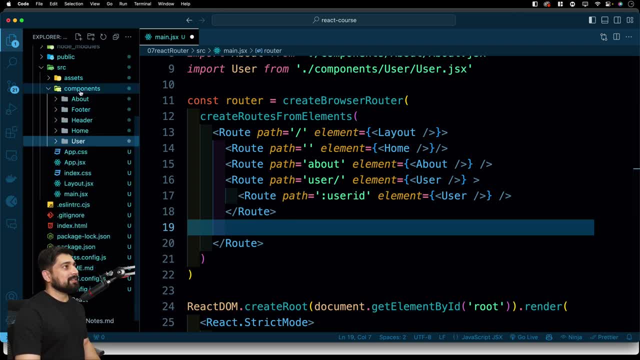 First, let's create a new component. That component will be again very basic, but very interesting one. actually, Let's go ahead and call this one as GitHub, And inside this we'll be creating a component known as GitHubjsx. of course, 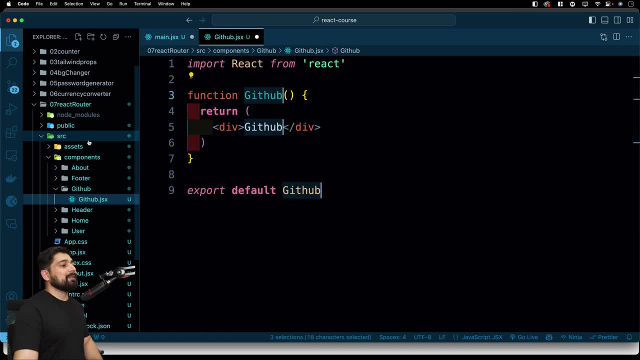 So we'll call this one as githubjsx- Again, RFC. that is it Now in this GitHub and all of this. what we want to do this here is just simply show some data into this one. First, let's go ahead and create this route. 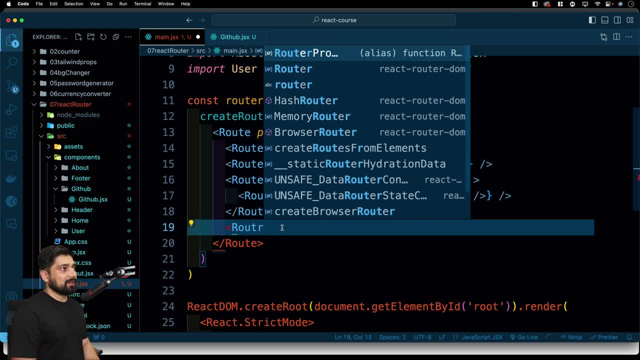 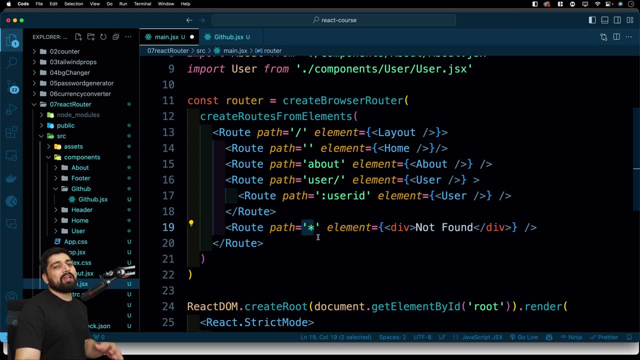 that would be super beneficial for us. So we'll be having a route, a route and there we go, And we don't want this path as strict. This simply means when you have a strict, that means all the 404 found. 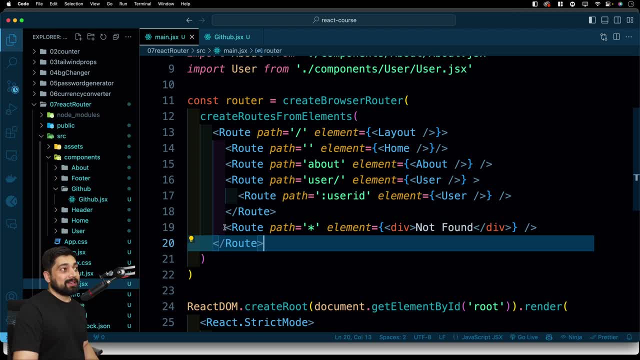 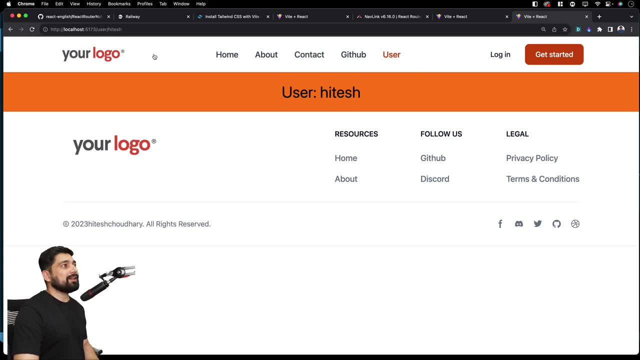 you can just put this element up here. So now, if we have this element, make sure this is at the very end of it, because they are evaluated on case-by-case basis. Now, if we reach out to something like contact, which we don't have defined, 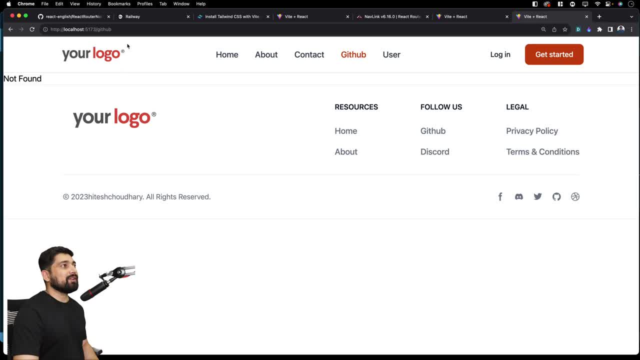 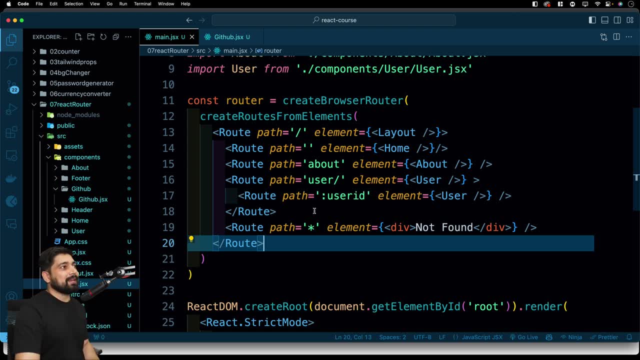 it just says not found. GitHub, which is not yet defined, so it says not found. So this is a classic example of if nothing cases. So have you studied? switch in cases? Yeah, this is almost like that. But before that, make sure it is always at the end. 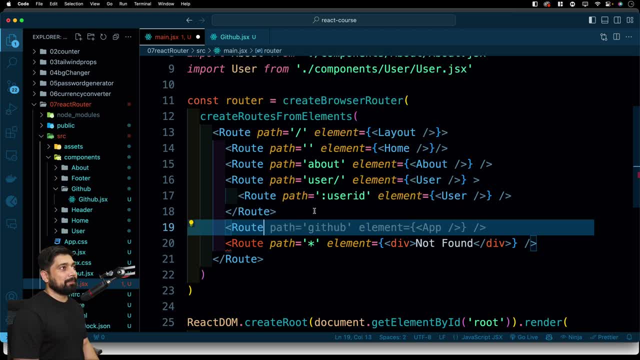 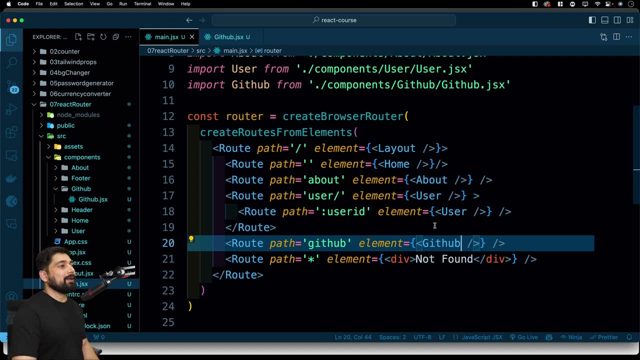 We also want to have this GitHub, So we'll be having a route and then we'll be having a route. a path will be GitHub and the element that we'll be loading is going to be GitHub. Yep, bring this one in here. 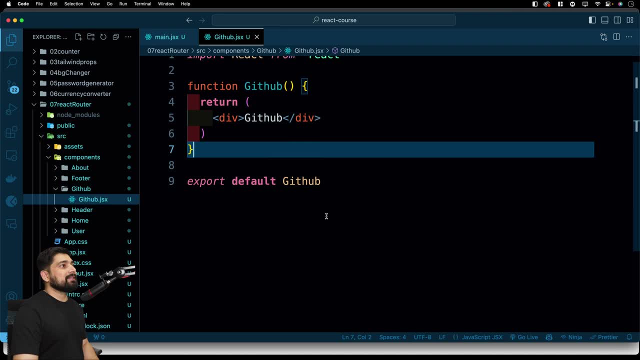 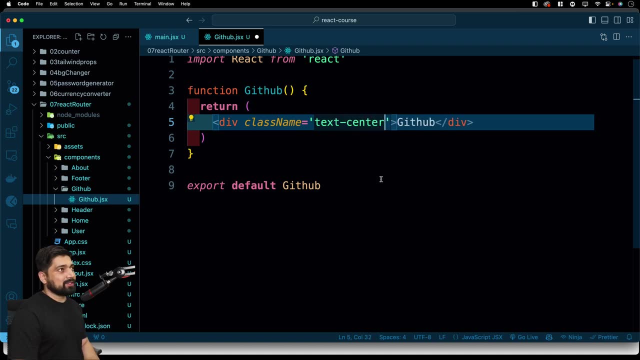 And now we have this GitHub and let's modify this a little bit, not too much, but at least bearable. So we'll have some of the class name. Let's grab first of all text to the center. I will be having a margin of four on all the sides. 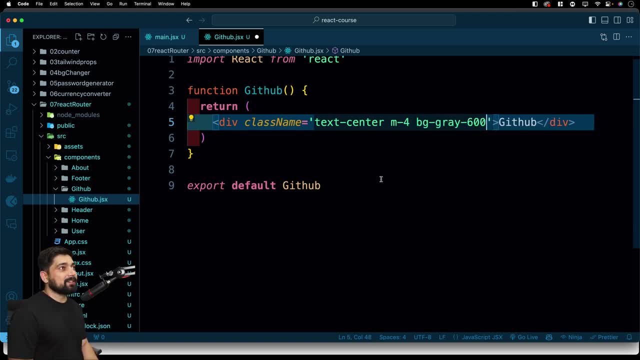 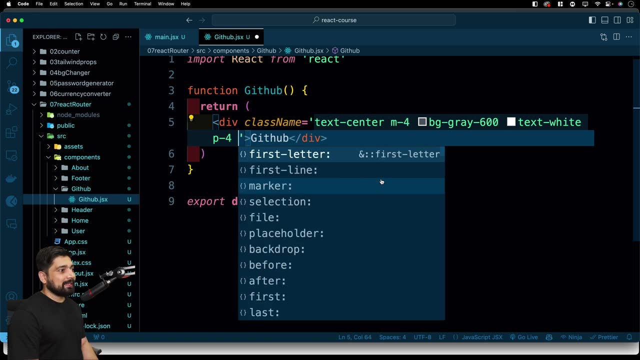 Background will be gray. How much gray? 600 is good enough. Text can be 100. White and what else? Padding would be four on all the side and text would be large. So three Excel would be good, And there we go. 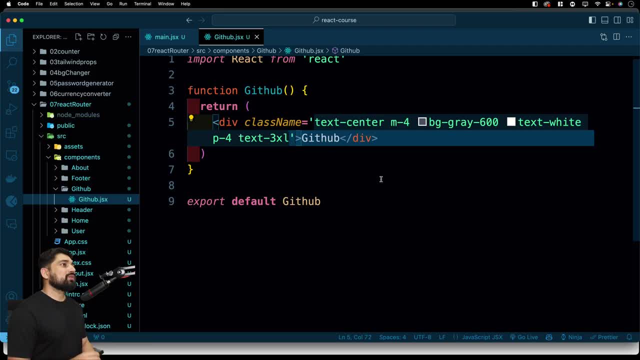 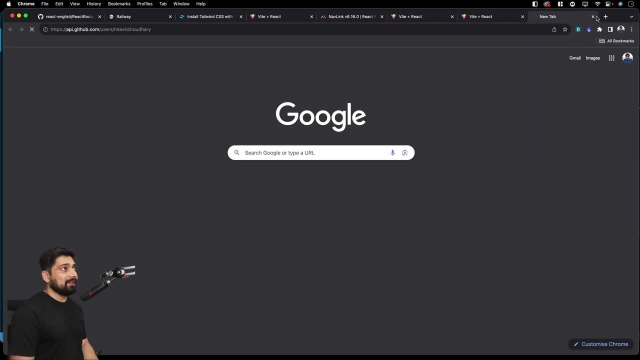 We have decent stuff coming up in here. Okay, now we have this one. Now I want to fetch some data from the API itself And, if you remember, fetching the data is not that hard and I can just visit this URL and grab some of the data. 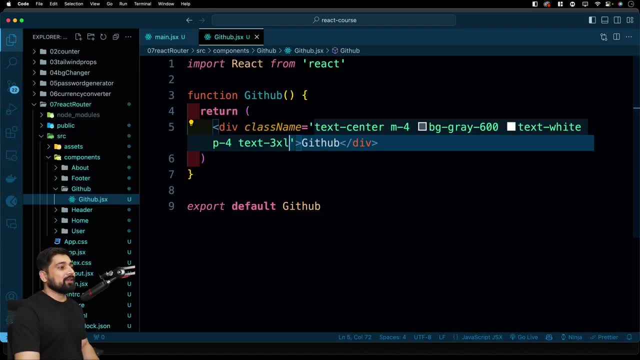 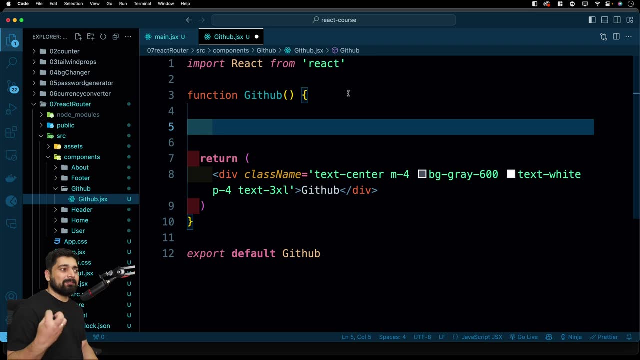 And it's an object that is being thrown at me. It's a public URL. You can also go ahead and make a fetch request there. So as soon as this component mounts, I want this request to be fetched up to me and I want to use that. 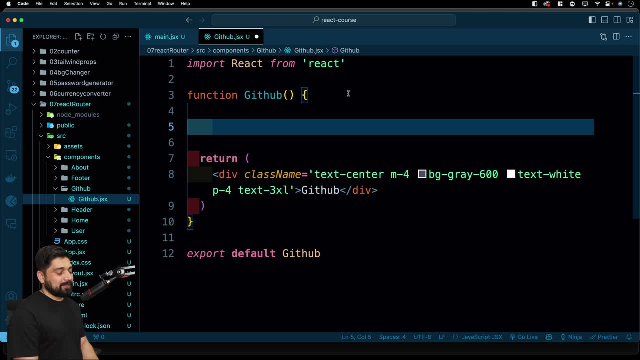 So one easy way of doing that is have a simple data as my state, so setData, And we'll be using reactuserState By default. it will be an empty array object. Whatever you like to have, We'll just have an empty null. 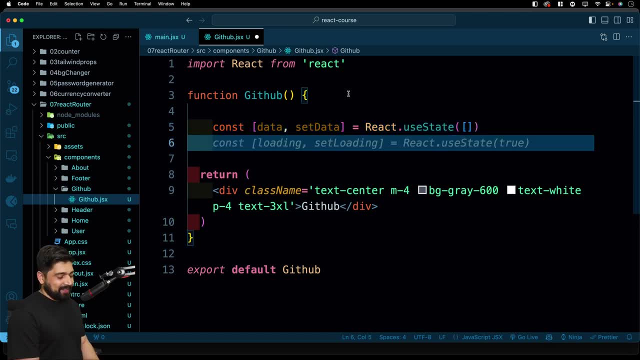 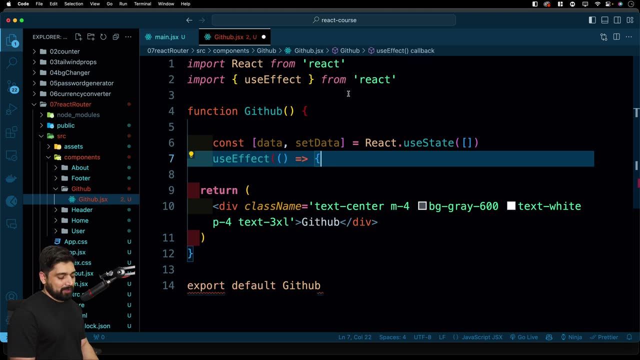 We'll have an array or maybe an object. We'll figure it out. Okay, Now I can use a useEffect, So useEffect in this, And there we go. We have a useEffect. It has no dependency array, so there we go. 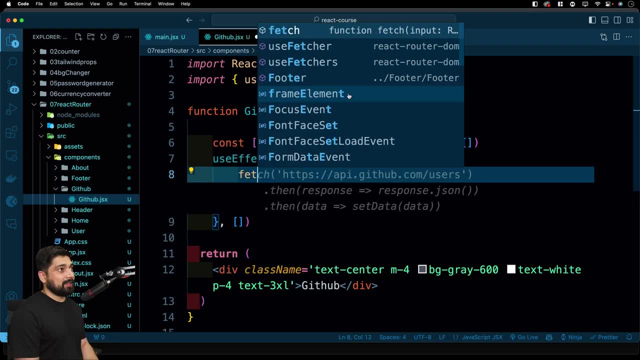 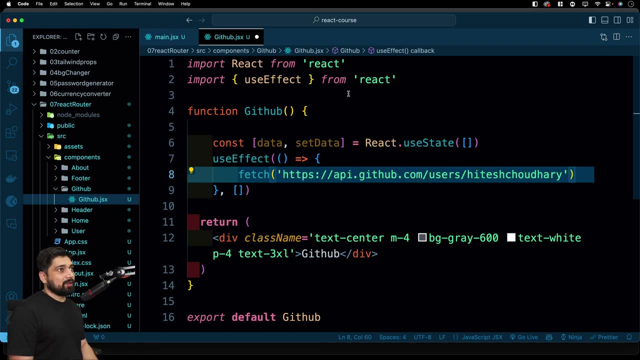 And now what will I do here? I'll fetch. So I'll say fetch, Okay, this is a nice boilerplate, but I'll write my own. I'll simply say: we want to fetch this URL If this URL gets a success. so we'll say then. 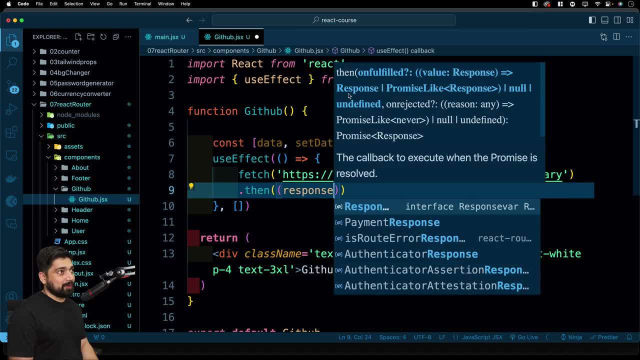 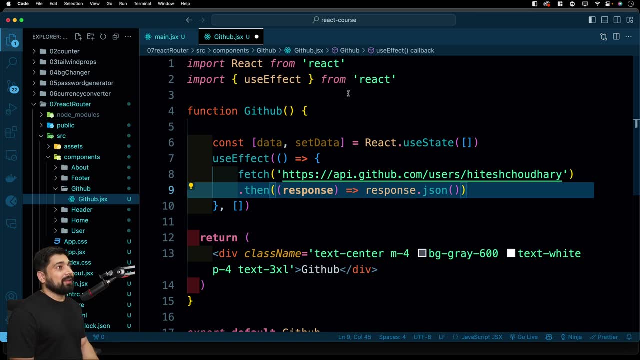 It will give me a callback. I'll say: let's call this one as response. It's in the string format. I need to convert it into JSON, So let's have the responsejson. Okay, Then chain on One more then, because that will actually extract the data. 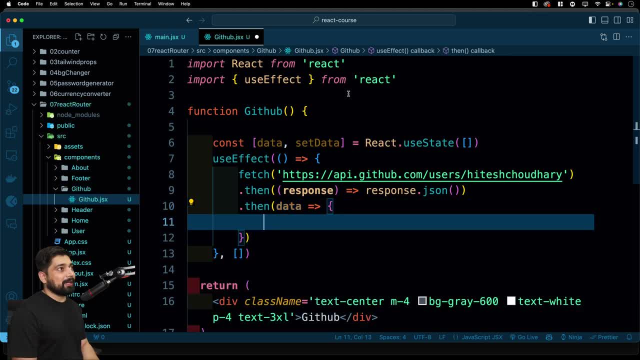 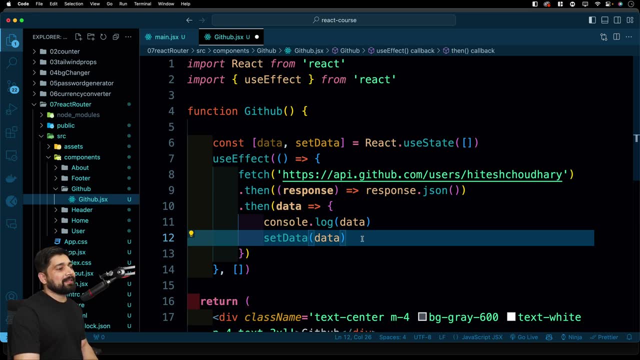 And we'll be having again a callback. Let's call this one as data. There we go, Callback, Just like this, And we can console, log the data as well as set the data into the data. So there we go. Now the data is being set into this one. 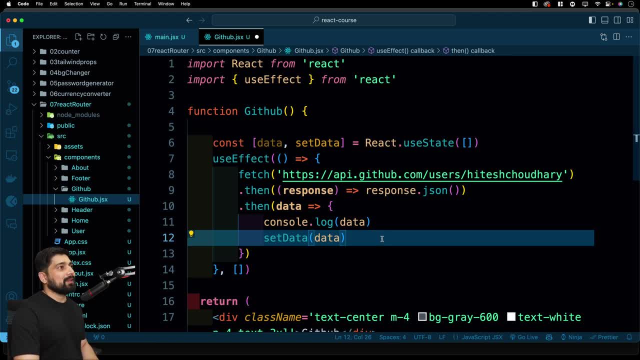 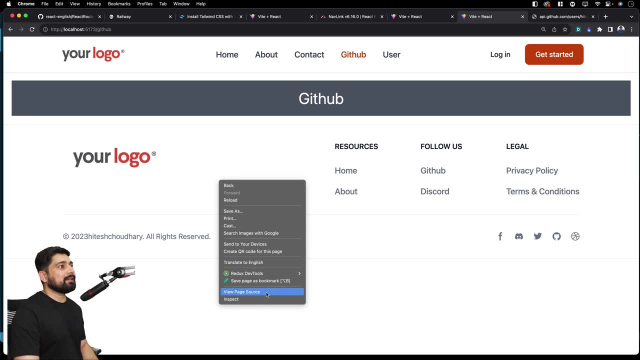 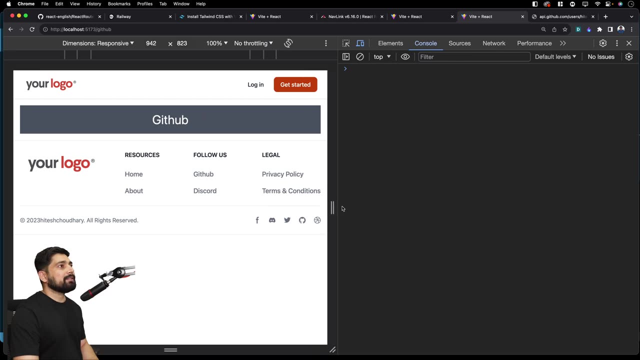 And now we can extract some of the data out of this one. Okay, So let's first console log and see if this is all coming up when we hit this particular route: Right click, inspect and console. Okay, Too much, And we will expand this a little bit. 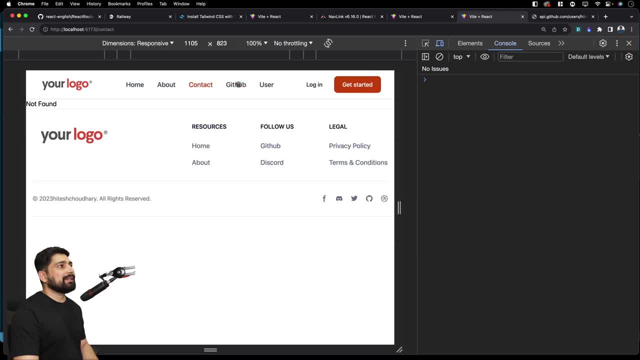 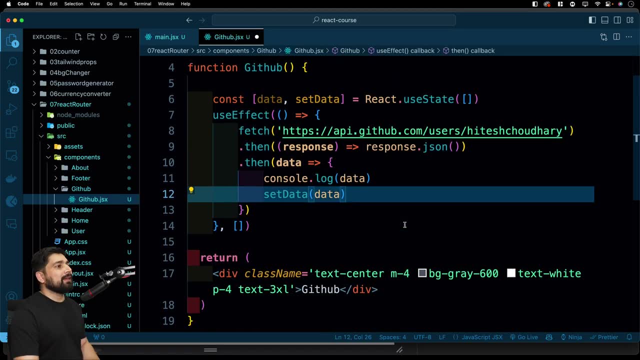 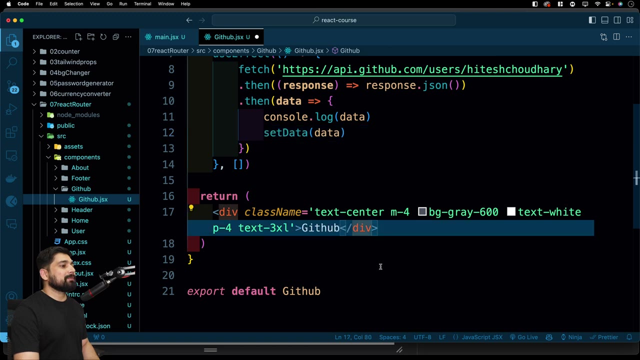 There we go. So if I go back to contact and load the GitHub, it gets nothing as of now because we are not using it. technically, Okay, Time to actually use this data itself. Interesting How we can use this Once the data is actually being set. as soon as the component mounts, save this, go back. 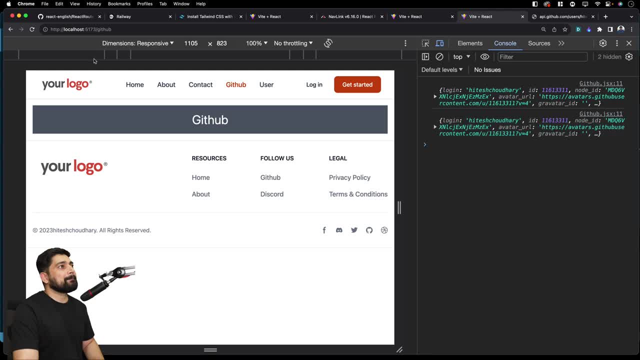 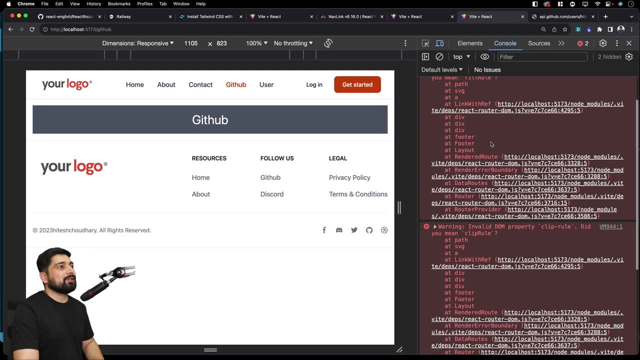 And now I can see I have this object. Let's reload this one more time. Probably I didn't save that. Okay, Fill rule. Did you mean fill rule? No, All these? Okay, These are just the CSS and DOM properties, not interested in them. 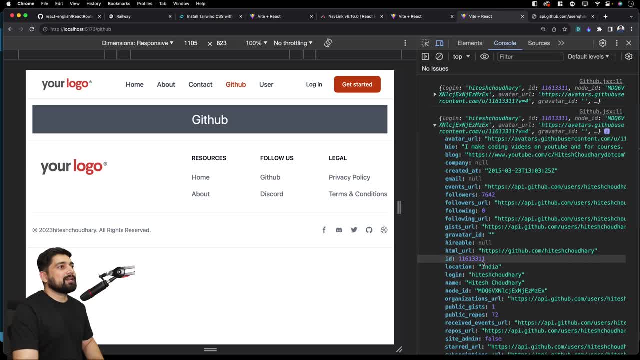 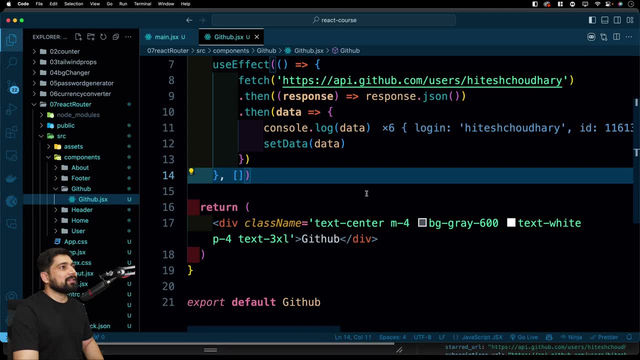 Contact GitHub. There we go. Now I have this object, which has a lot of data And probably out of this data, Because I'm console logging the data And I am console logging this, So let's extract some values out of it. 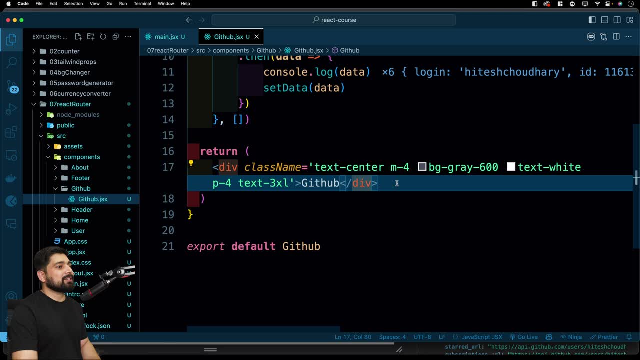 So what values can I grab? First of all, the followers count, maybe Followers? There we go And let's inject the variable. since I have access to this data And if you have studied this, you know that I've actually gone through many times- 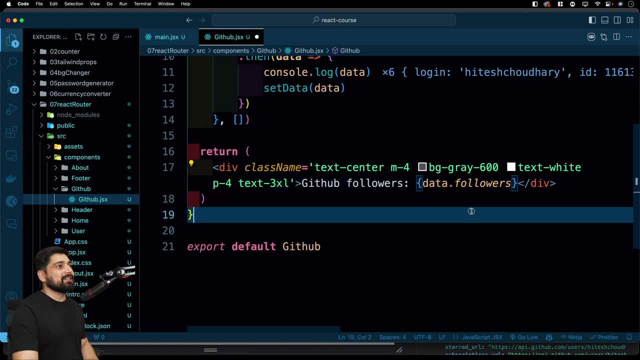 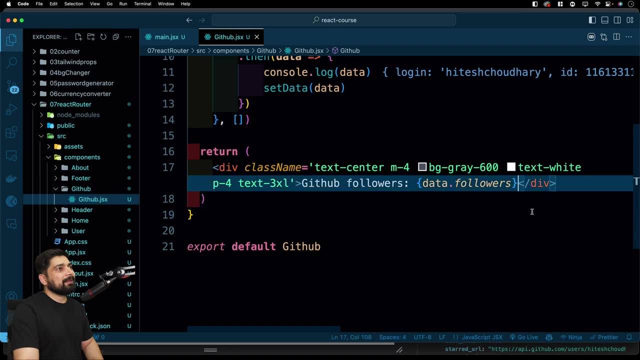 You can just extract what do you want. I want just the followers count here. So that's why I just mentioned this, And there we go, I get the followers count. So notice, here we can grab the image as well, Should we? 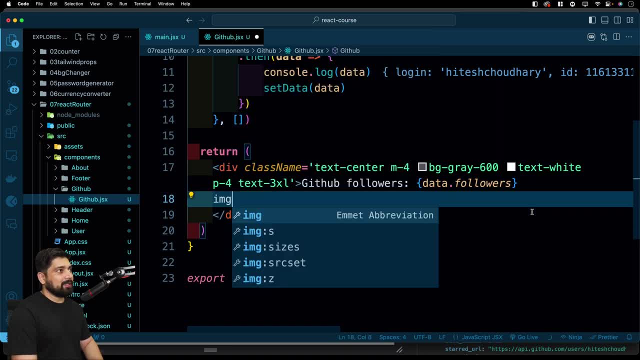 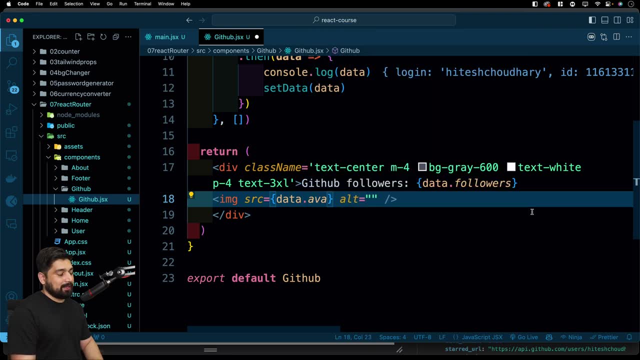 Yeah, Let's grab the image And I'll say I'll be needing an image. There we go. What is the source? Source will come up from data If the data has avatar underscore URL And we'll also need to give a width of 300.. 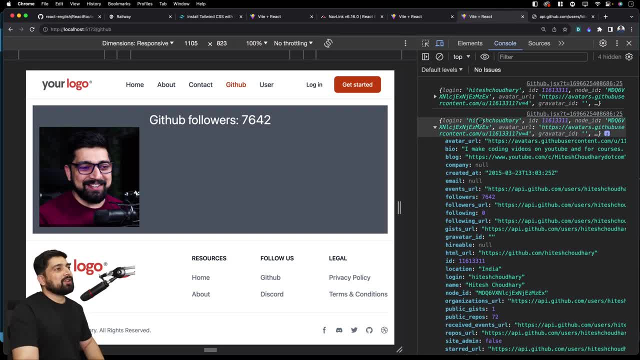 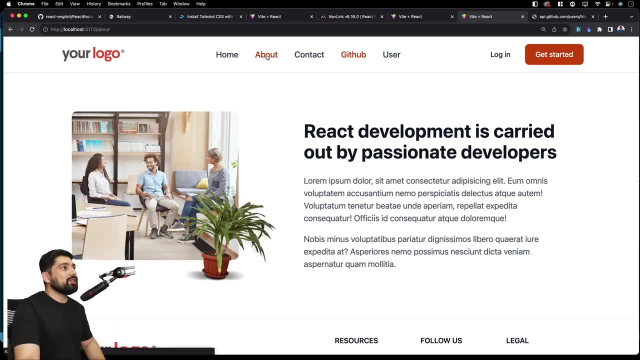 All right, So we have this image. All right, So we have this data. Now here comes the interesting part, where things will get a little bit more interesting: towards the router. I go into about, I go into contact When I go on to GitHub. that is where the request is being sent. 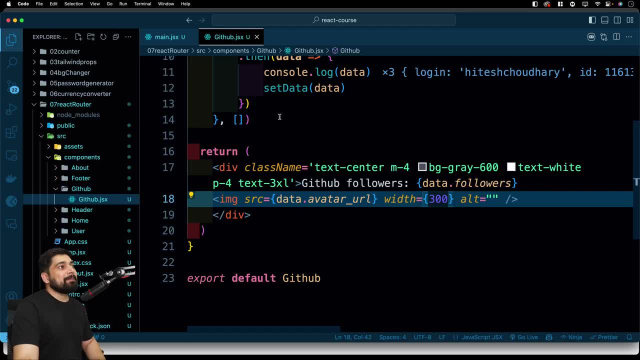 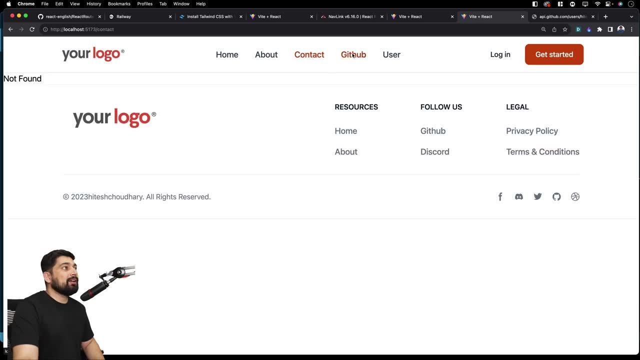 We cannot simulate this one as to come up after a few seconds, But what you'll notice, the use effect will only take place when this component particularly loads up on the page. So contact When I go up here. so this will make a fetch request. 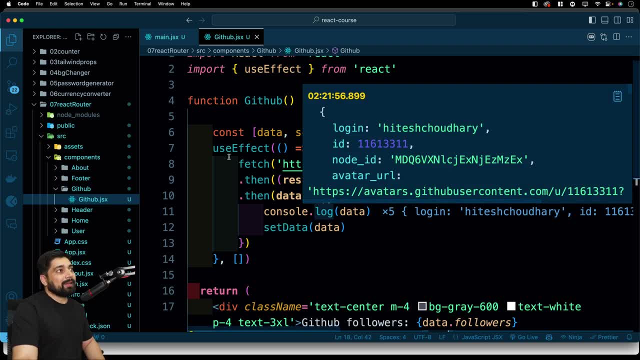 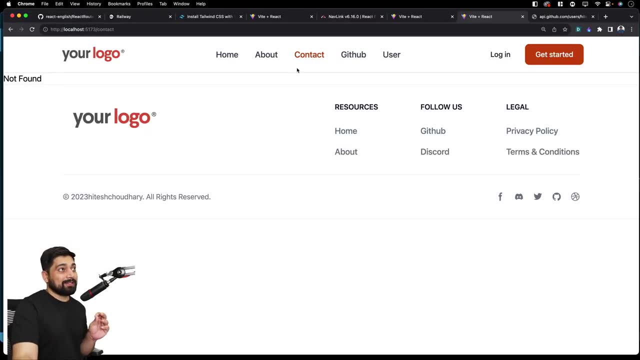 Now, what if we could have done this a little bit better? Can we optimize this? This is already very optimized, But what if there could be advanced stage of this one, Like, for example: I'm going into contact before clicking on this, I keep my mouse hover for probably a fraction of second milliseconds, but then I click on? 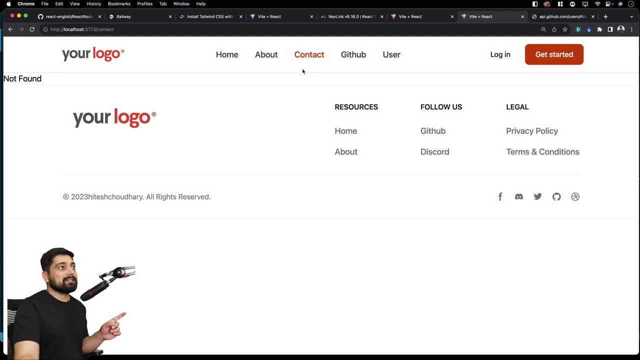 it. The same thing can be used for the advantage. Nextjs does exactly same. when you actually pull your mouse over over this one, It automatically sends a network request to load all the resources that you require, And then, when you click on it, the things are already available for you. 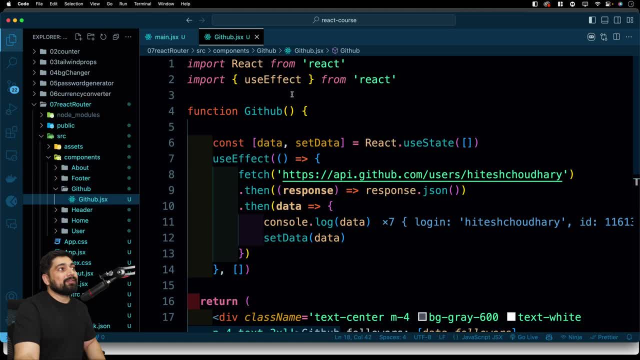 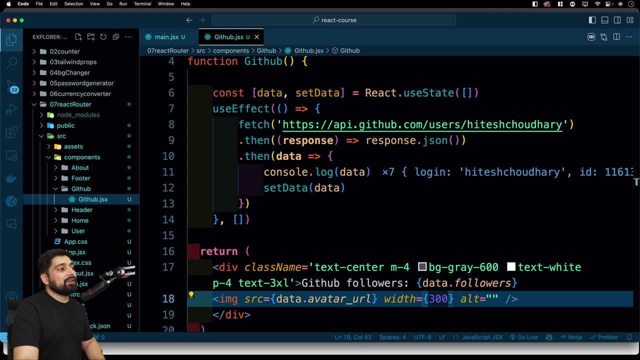 Okay Now how can we do this in this scenario with the React Router DOM In the next years- it happens automatically behind the scene- but how we can actually do this one up here Now doing this. all of this thing is actually super, super easy. 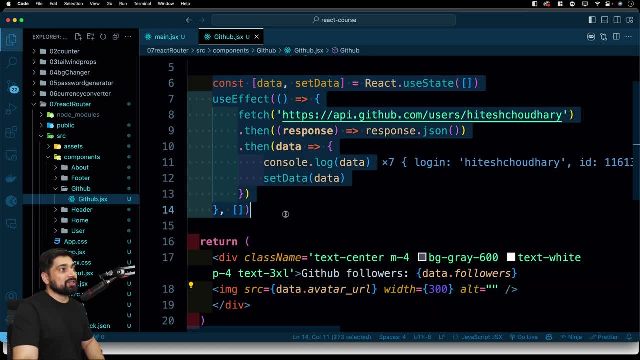 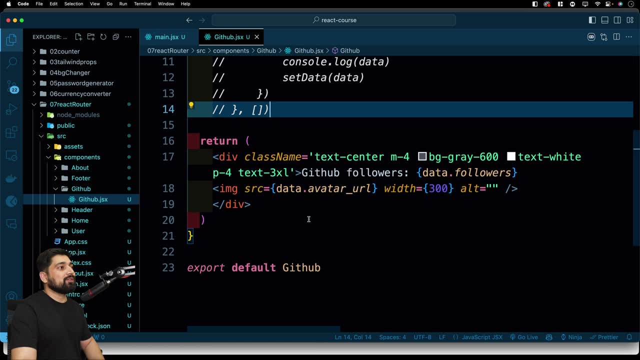 Let me show you how this is done. First of all, we don't need this data and all of that. This was just to show you that, how regularly we do this again, and a good example exercise. We'll just come in this one out and we'll write this thing again. 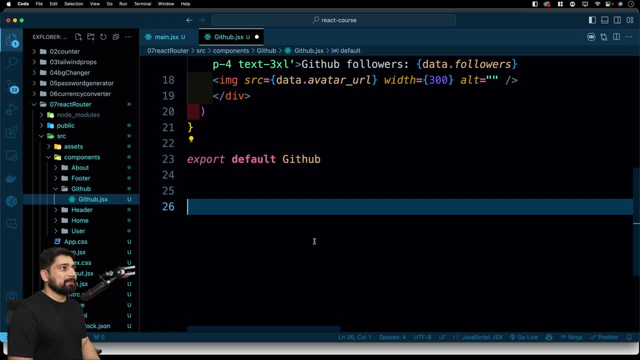 You can. Usually, there's a case where people write these kinds of methods. Okay, You can write these kinds of methods in the component itself, but if you wish, you can separate that out as well. All you have to do is export a kind of a method. 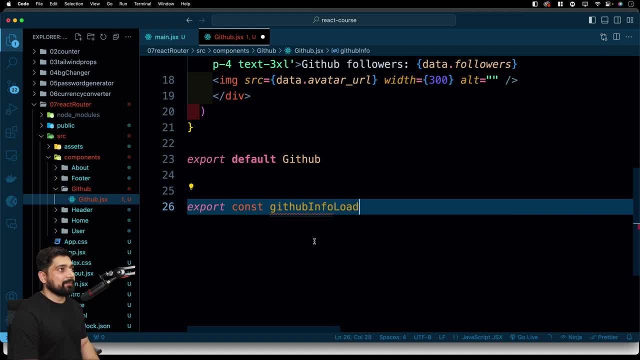 We'll call this one as GitHub info loader And this one is going to be a simple callback, just like this. But the only method only advantage we want to take care here is is we want to make this request as a sync. Previously we were using the fetch in the dot, then syntax. 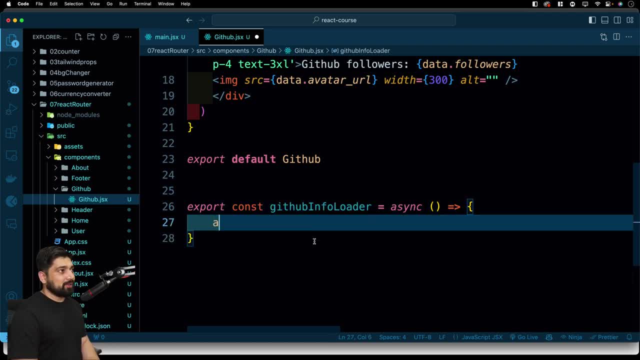 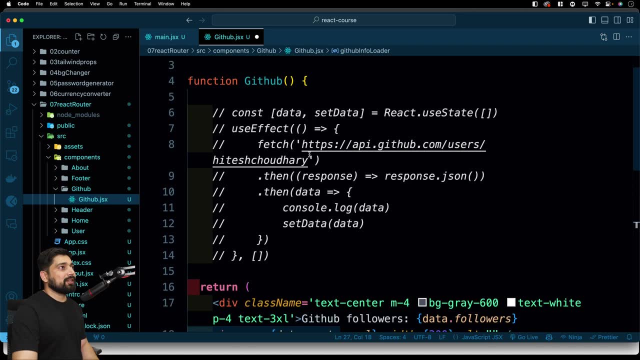 You can use that as well, but I want a sync here as well. Okay, So what we'll do is we'll obviously await and we'll do the fetch, because I don't want to continue if this is not there and the fetch is going to fetch the same URL. 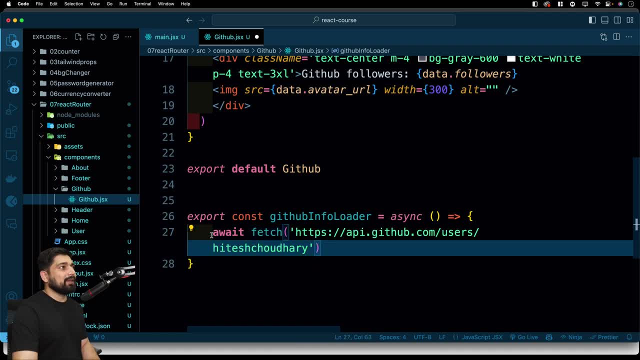 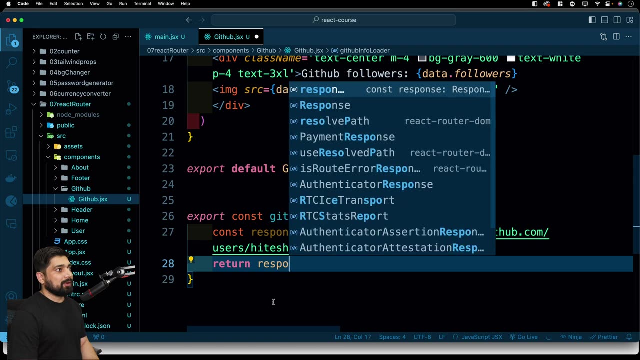 No changes there. We know that this works, and let's hold the response into a variable, So let's call this one as response. So there we go, And now all we have to do is return. return this response. We don't need to await this here. 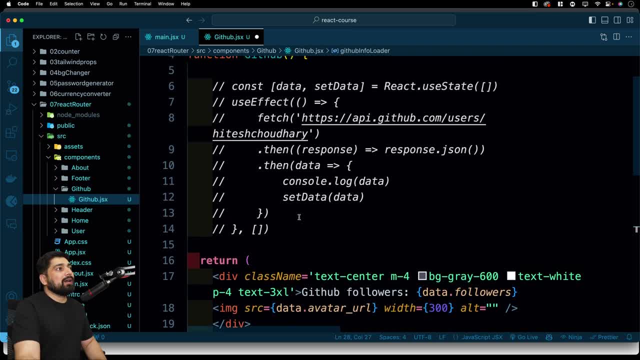 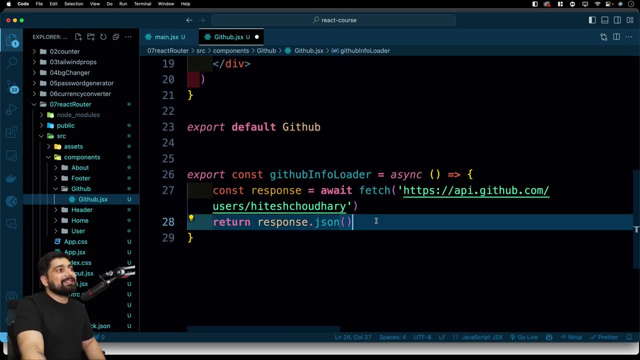 Responsejson. Okay, Now notice, here we are not, we are just responding, returning this response. We are not having this data and whatever that is, The good thing is, I can return this as it is Now. once you are returning this, then the next step actually is almost in this file. 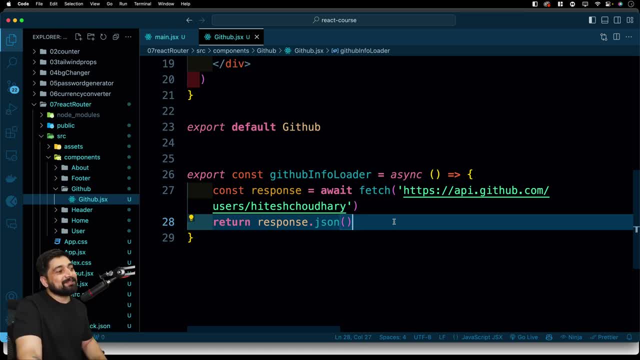 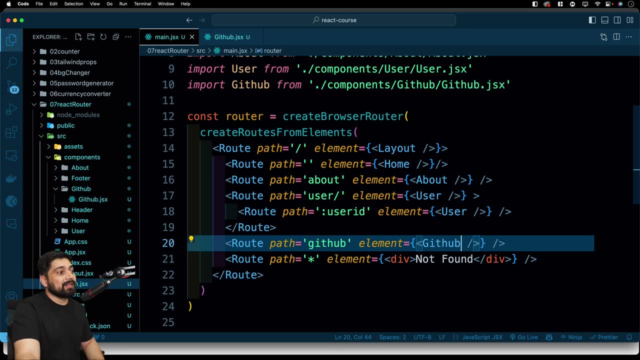 but we don't do this here because this is not the data flow. Understanding the data flow is important. Once you are done with this, this method actually first gets loaded into mainjsx, where you're actually having this routing, So this method needs to come up here. 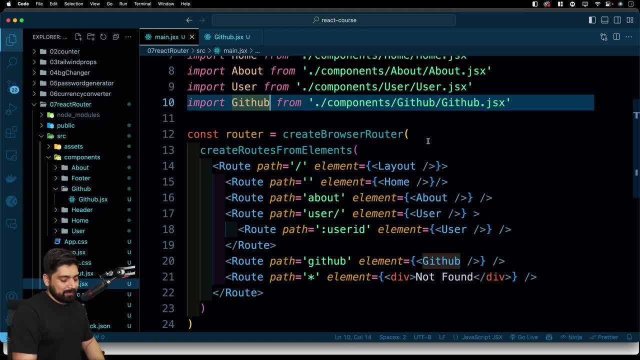 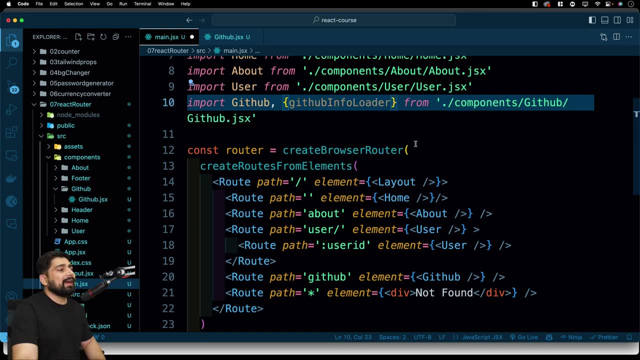 Let's go ahead. Notice, the method actually exists in the same component. That is why a lot of people prefer to have this here. We can just go ahead and say this one is going to be GitHub info loader, whatever the name is, And then, once we are done with this, we don't actually load the GitHub, just like this. 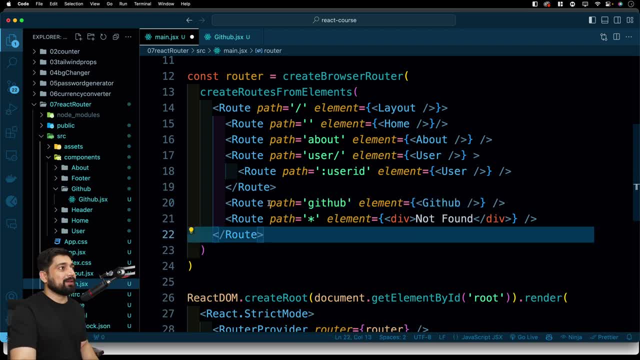 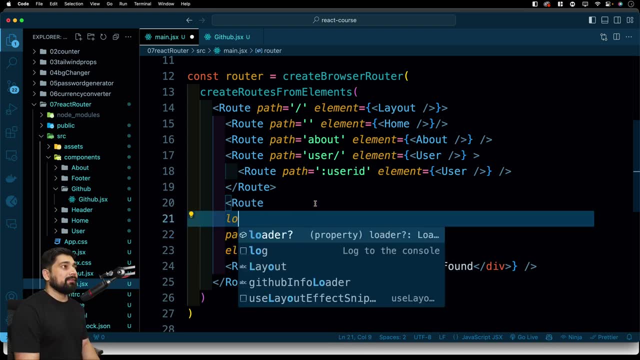 We actually provide additional property. No, we don't need to use the sandwiching, but we need to provide additional. The path will be same, The element will be same, but there is one more element, or prop, which is known as loader. 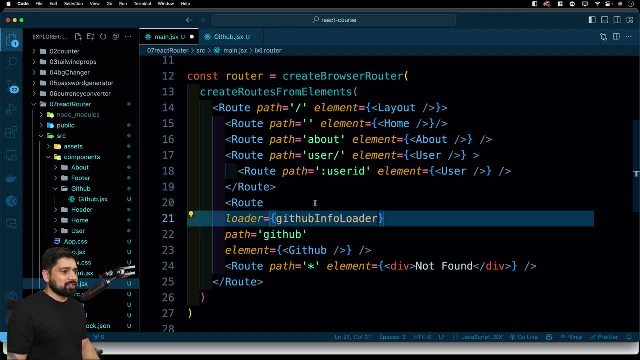 This loader actually takes a method That, whatever the information you need to fetch, calculate whatever you need to do, just get me that method first so that if somebody is trying to load this route, I can do some of my advanced pre-processing on it. 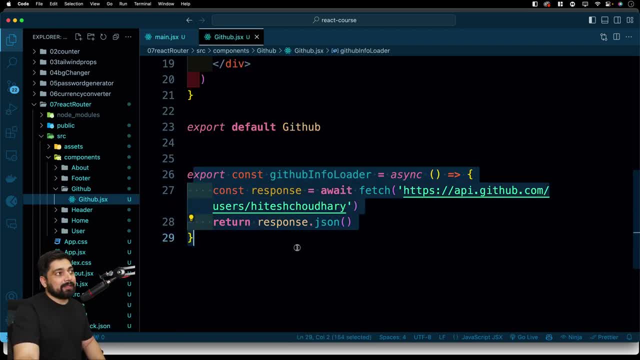 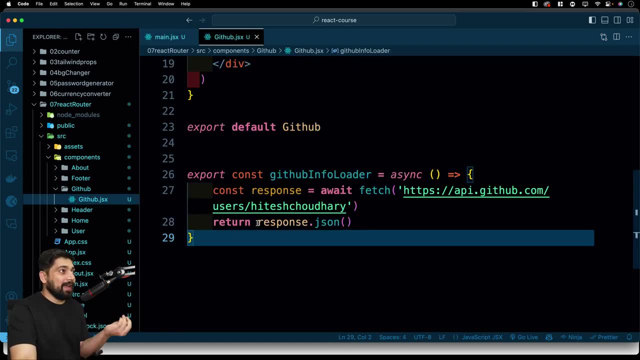 Once you are done with this, the next question in your mind would be: okay, we created a method in this file, We exported, gave this method to this guy, but how can I get the data from this whole method? I have returned the response, but I need this. 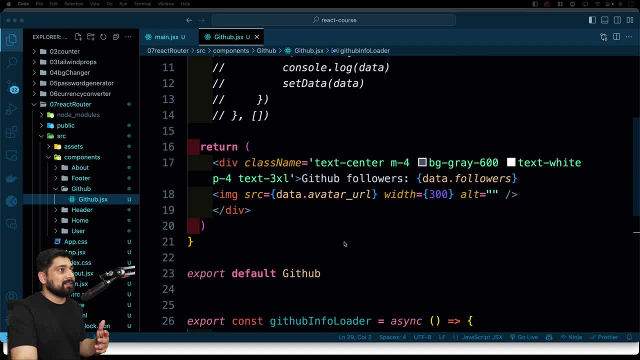 This is a common mistake, that a lot of people do this. hey, since you have exported this here, You can go back to the method and grab the data. No, no, you don't do that. That's not a proper way of doing the things. 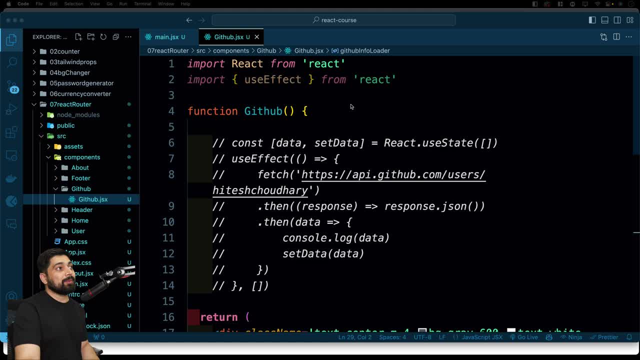 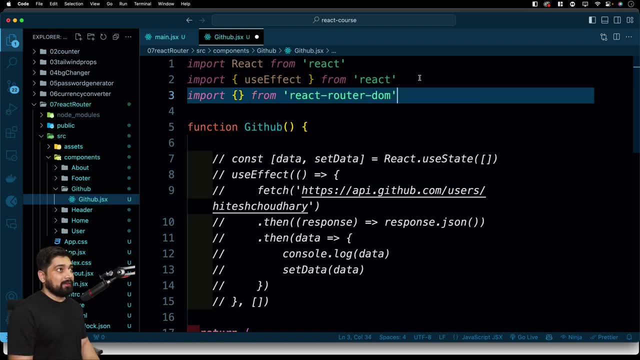 In this case, when you want to have this, you actually use a hook which is given to buy it to you by react router Dom. So let's go ahead and use this, And this one is coming going to come up from react router Dom. 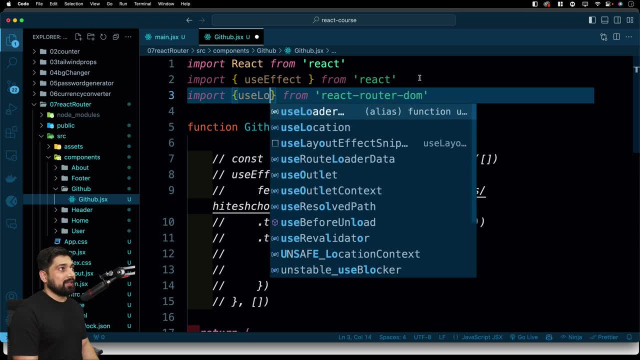 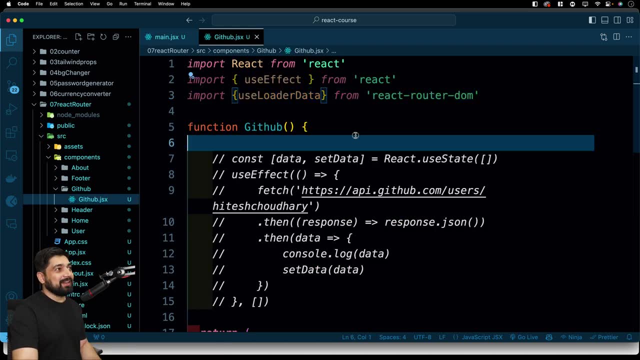 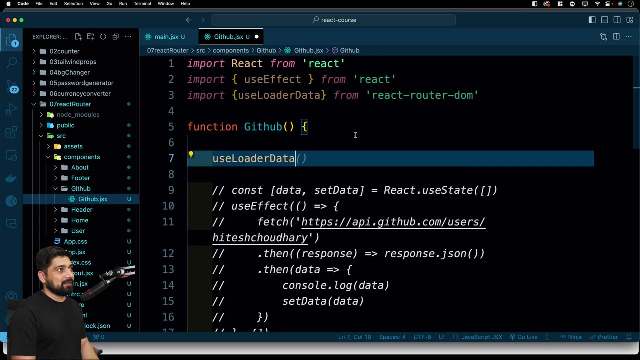 The name of the hook is pretty simple. You can guess that: use a loader data. Yeah, The property name there is loader And here is the use loader data. Since this is a hook, You obviously know how to use the hook, So it's a simple use. uh, use loader, just like this. 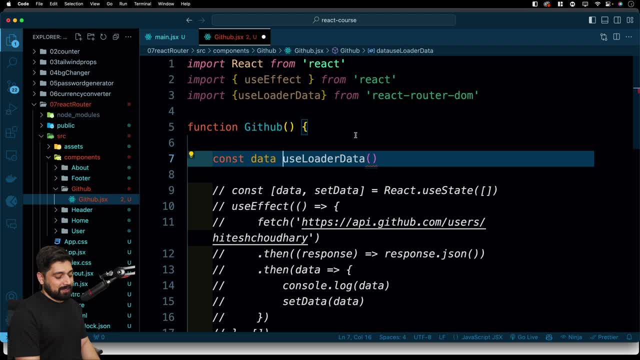 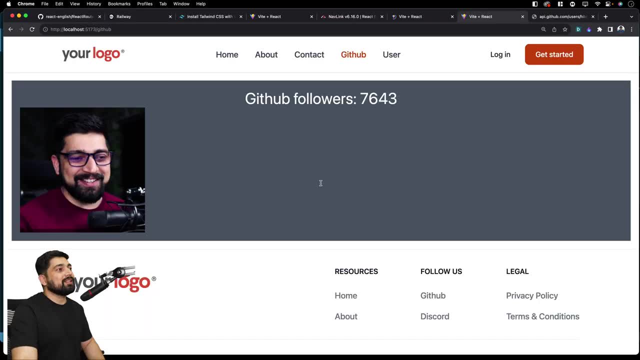 It's a method. There we go And you can extract data from it. So call this one as data, since all the variables that we named them as a data dot followers. So this will have that object and you can extract the information. So now, uh, technically it looks same that, Hey, we have contact about. now. if I go to 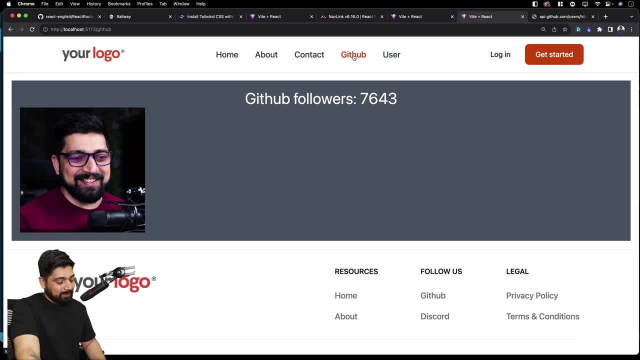 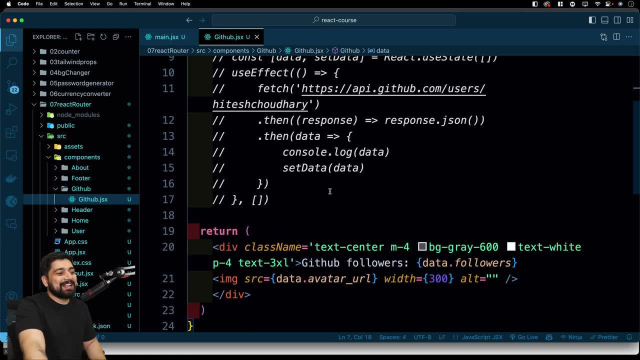 GitHub. it technically looks same, but it's actually doing a lot of pre-processing for you. in the smaller application like this, It is little bit difficult to find that it is adding some value for us. but trust me, it is adding a law, a lots of value and this exact same pattern. 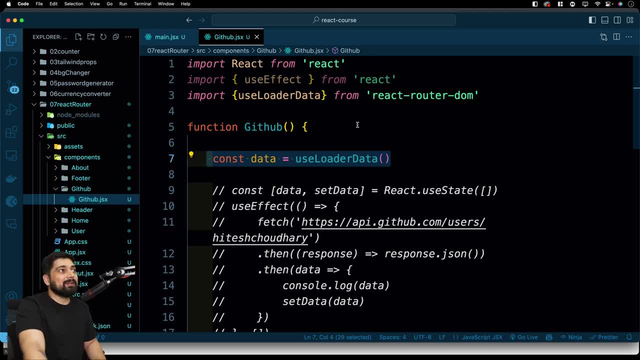 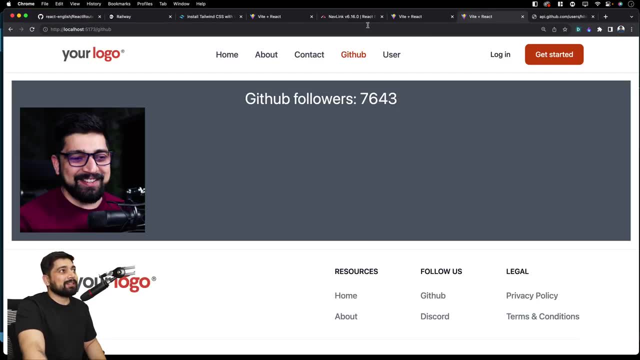 You don't have to use that much of hooks, and stuff is used in the next JS as well. They also do a lot of preloading and pre-processing of data. Uh, a lot of fun stuff is there, but, by the way, this whole thing is actually available. 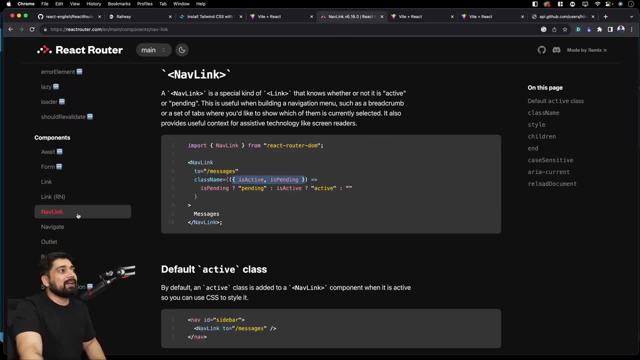 in case you want to use classic react and some of the applications, uh, you can actually go ahead and use that. by the way, there's a lot of things you can go ahead and work on with this one. There's so much of routes available. 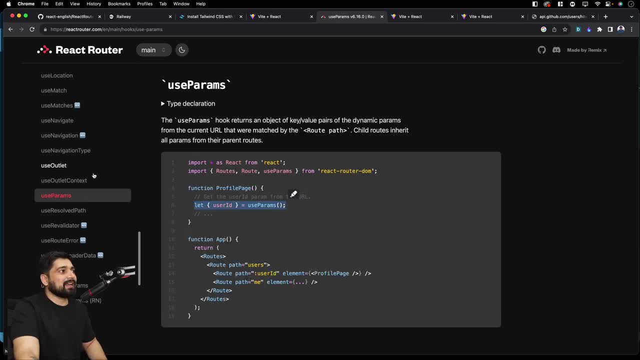 One that we studied is use params. So user ID: use params. This is exactly what we studied. Uh, we have so much more use submit user out there's. there's so much of advancement. In fact, there could be a separate course on this in itself. 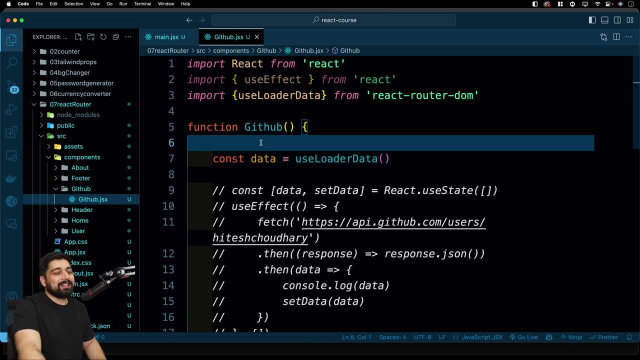 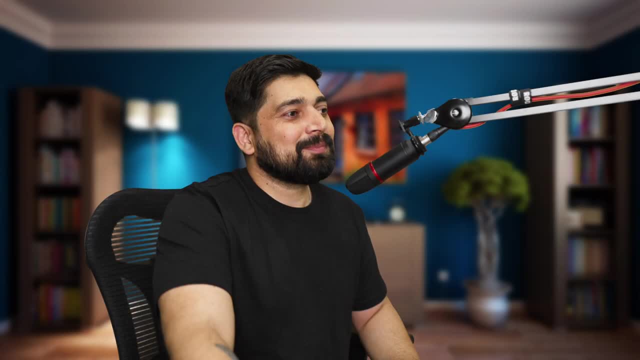 I'll try, probably in the future, to create one search If you have. if you really want this one to happen, let me know in the comment section. I would love to do this as a as a course in itself. So this is pretty good off. one crash course on the react router. 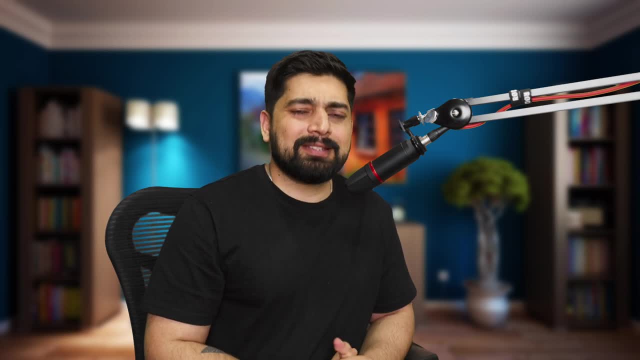 All the advanced things Which you probably are going to need are covered up. Yes, there are still more. uh, something like forcefully pushing the user onto some page once we have logged in, and all of this will be covered up later on when we'll do some. 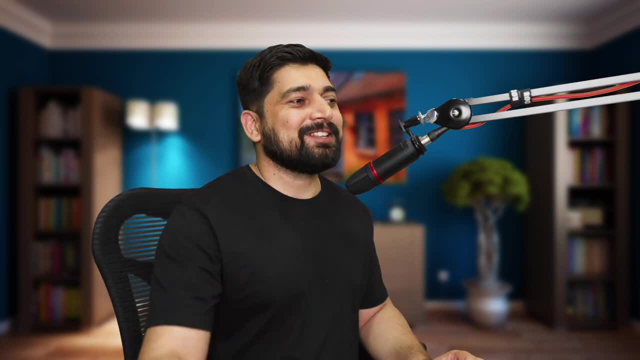 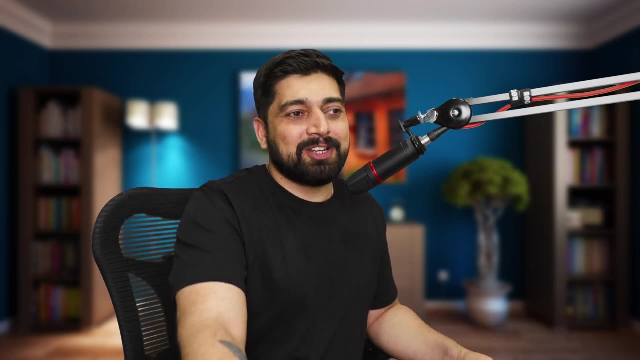 of the mega project, But I think that is enough. That is more than enough for you as a react router. crash course. Uh, that's it for this one. Make sure to leave a comment in the comment section. I would be really, really appreciating that. That's it for this video, and let's catch up in the next one.